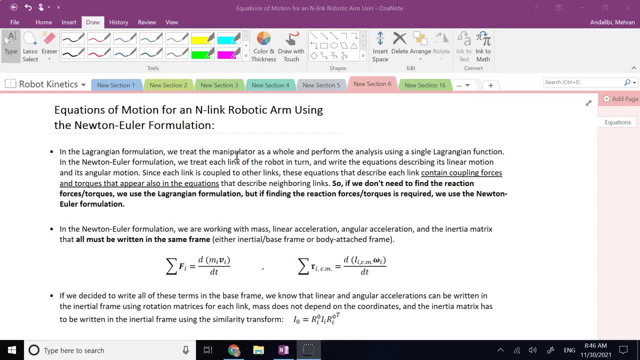 But if the joints fail during the motion of the robots, that is definitely not desired. So in those cases the second formulation is going to be the Newton Euler formulation, And this is what you are familiar with from your dynamics right. Some of the forces is equal to time rate of change of linear momentum, which is mass times. linear velocity. 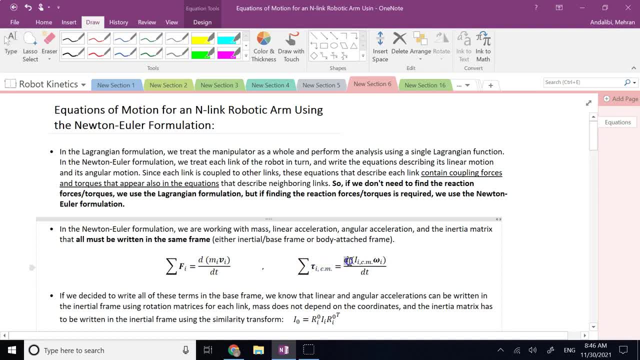 And some of the moments or torques about the centroid- is equal to time rate of change of angular momentum, Where angular momentum is the inertia matrix, I times angular velocity, omega. So these are the two important rules That we have in Newton Euler formulation. 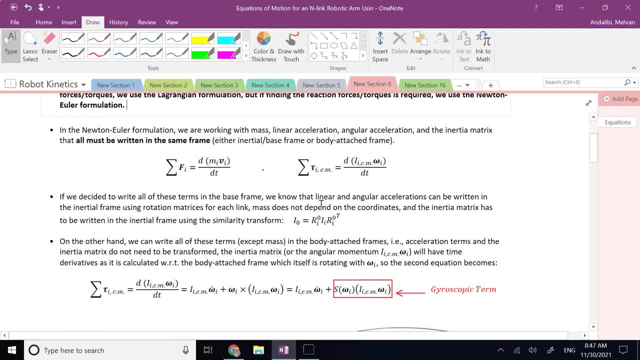 And the important thing here is, when you write these equations, you describe everything in which coordinate frame. right, Because you know for a robot you have lots of different coordinate frames. right? Specifically for a link. you can describe everything either with respect to the body attached frame, which is a rotating frame, 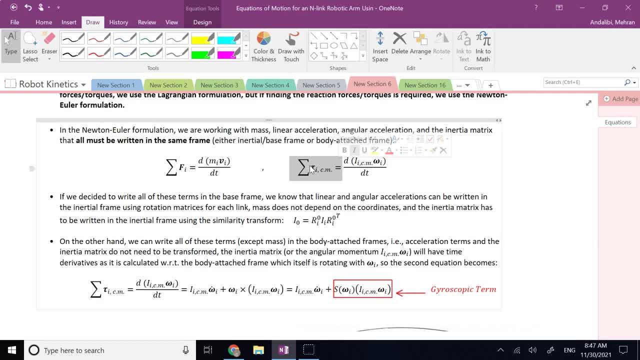 It has motion, it's not an inertial frame. Or you can describe everything in the base frame which is inertial And with respect to time, the unit vectors of that base frame do not change While the body attached frame it has time varying unit vectors because they do have rotation. 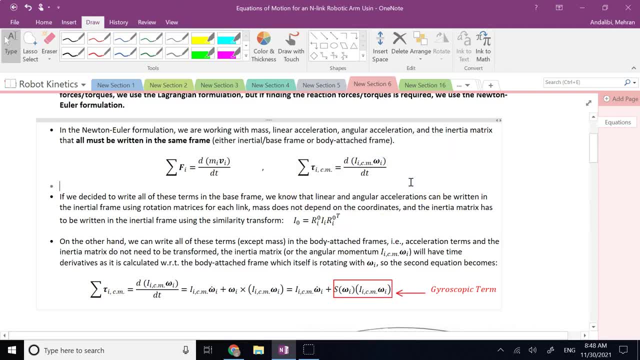 So, depending on which frame you write these equations in, you will get a different appearance Of the final formulas, But at the end of the day, both of them will provide the same kind of motion And the same calculations for the reaction forces or torques or anything. 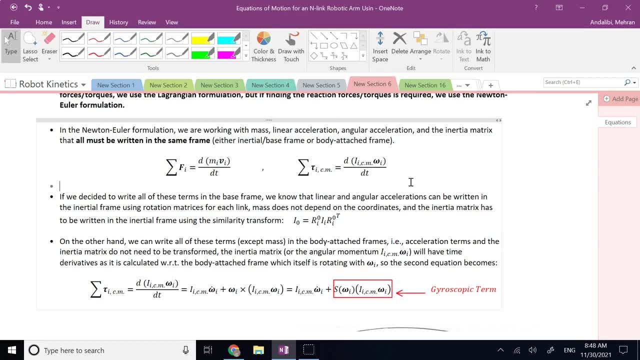 So, although they might look quite a bit different, But if you really do some heavy algebra and try to simplify, you can see that they are the same thing. Or if you do numerical solution, you'll see they give you the same number Or numbers. 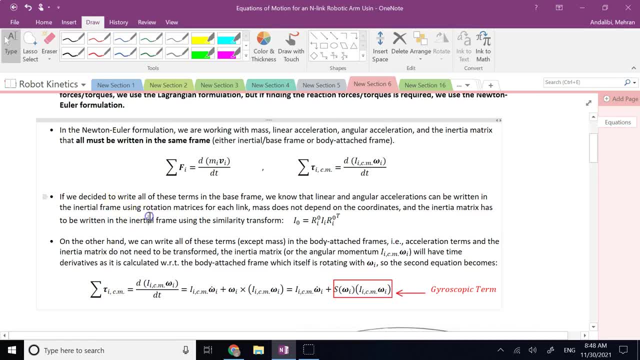 So let's discuss each case. If we write everything in the base frame, okay, If we write everything in the base frame, what's going to happen? Let's look at the entities that are involved. We have the forces and the torques. 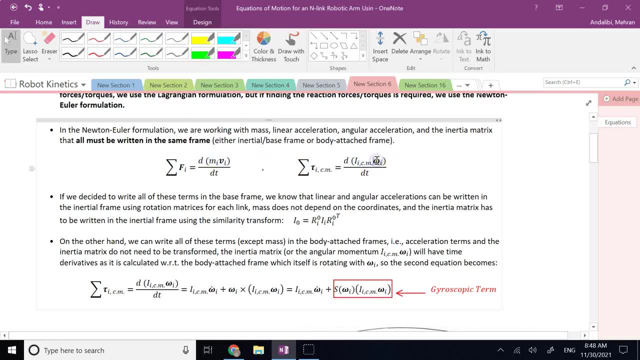 We have the mass linear velocity, inertial matrix, angular velocity. Which one of them do you need to care about? Which one of them is it that You have to pay attention to its variations? So how can I write linear and angular velocities for each rigid body in the base frame? 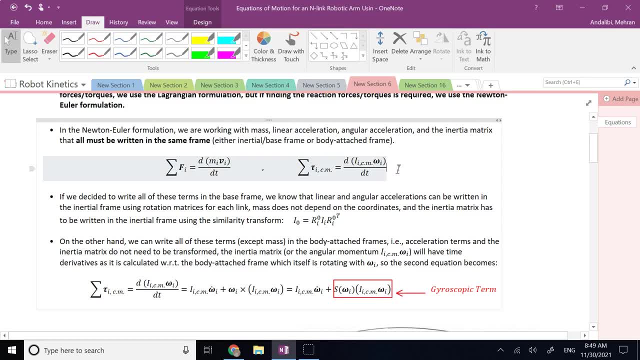 Well, that's not a big problem. We learned about Jacobians And we learned that V and omega right Can be written in terms of Jacobians, Or you can directly use the kinematics formulas of rigid bodies, Which is equivalent to that, correct? 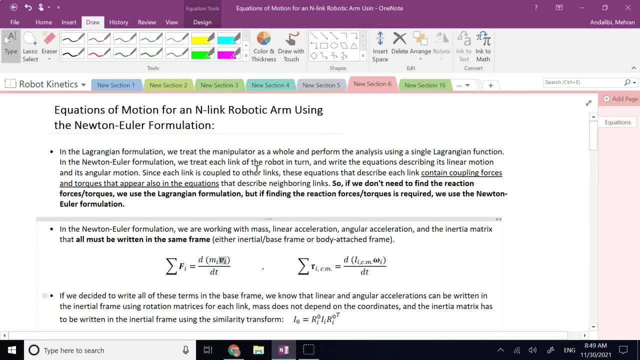 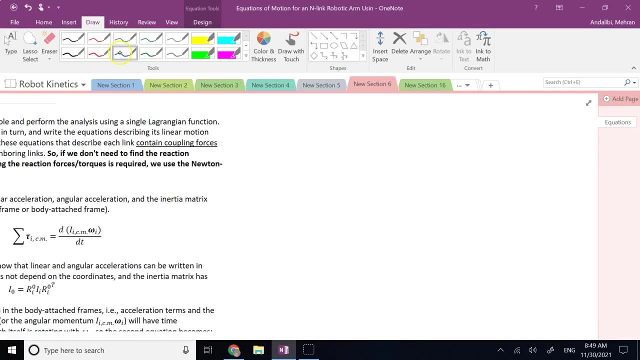 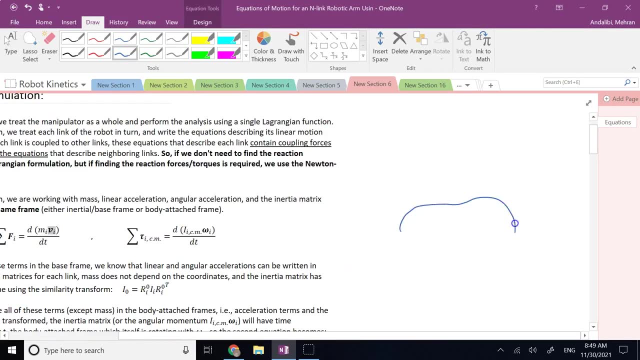 So if you remember from rigid bodies, you know that if I have a rigid body then Let me show you. So if I have a rigid body like this, Let me try to write a little bit better. Here we go, If I have one point here, right? 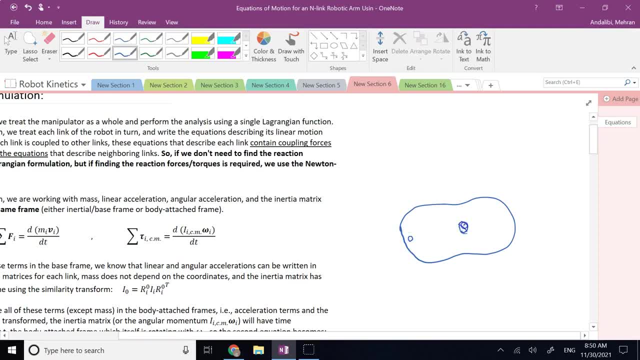 And then I have also the center rate here. If this one point on the rigid body I might call it point A And the center rate I call it point C, If I know the velocity of point A correct. So if I call this V. 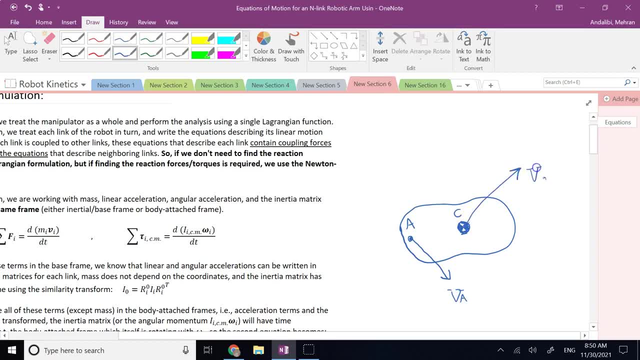 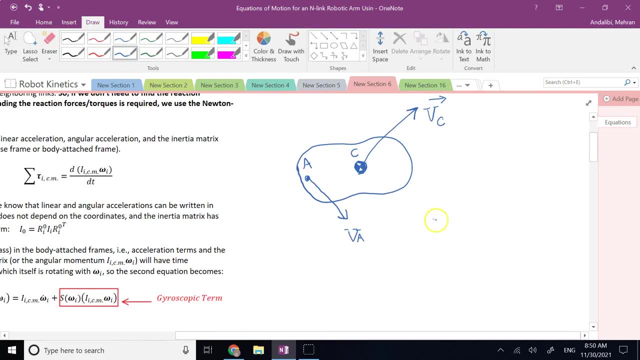 And the velocity of center rate is this one, V. I can relate V to V based on what we have learned in dynamics And if you forgot about that, please watch my playlist called Dynamics And look at the velocity analysis of rigid bodies. 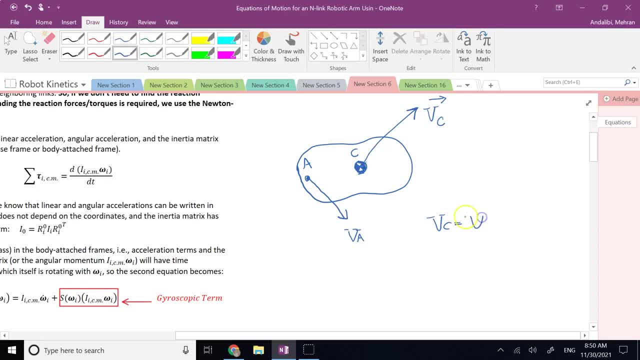 Okay, And you will see this formula and how it is derived. V will be V plus omega of the rigid body cross R with respect to A, Where R of C with respect to A goes from A to C, this vector Right. So this is what we learned from the rigid body kinematics. 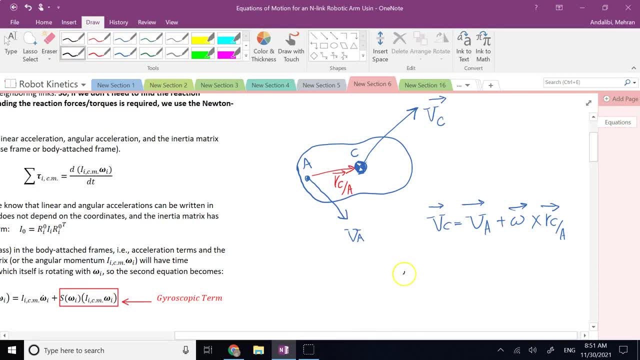 And similarly also, if you remember, A of the centroid is equal to A of A, If I know the motion of A, both V and A of it. then plus what Omega dot Cross, R of C with respect to A. 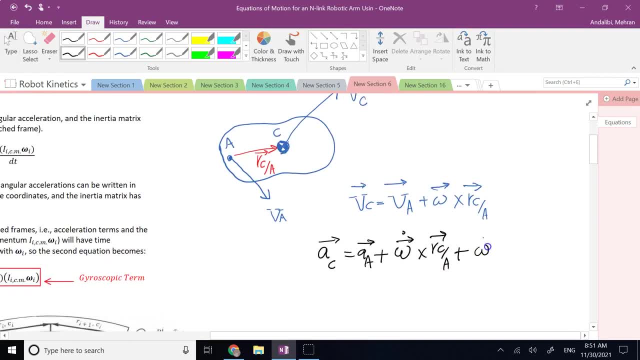 And then plus omega cross, Omega cross, R of C with respect to A, Where this is called the relative centripetal acceleration And this is called the relative tangential. So this is called A of C with respect to A tangential And this guy is called A of C with respect to A normal or centripetal. 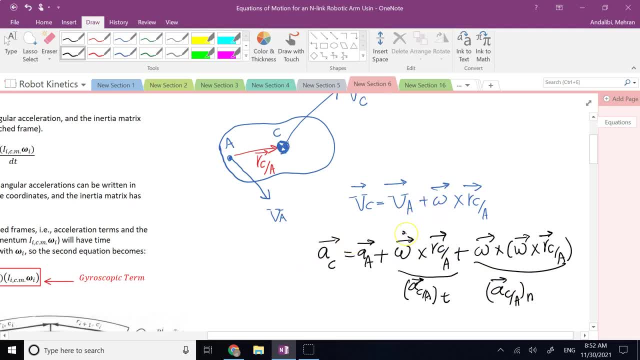 Correct. So these two formulas are what we remember from rigid bodies And we can use these to find what To find? omegas Vs As and alphas really that we need, Or omega dots, So why don't we use the Jacobian here? 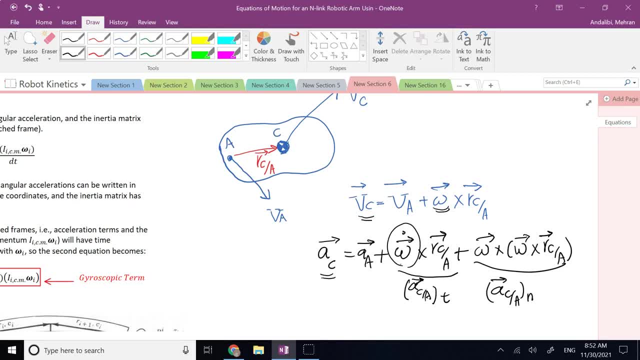 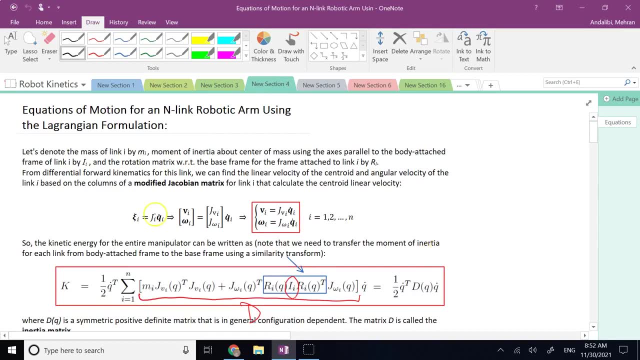 We can if you want to. But since that Jacobian method we mostly use in the Lagrangian formula, here we are using the different analysis. As you remember, we used V and omegas, We determined them using JV and J omega. 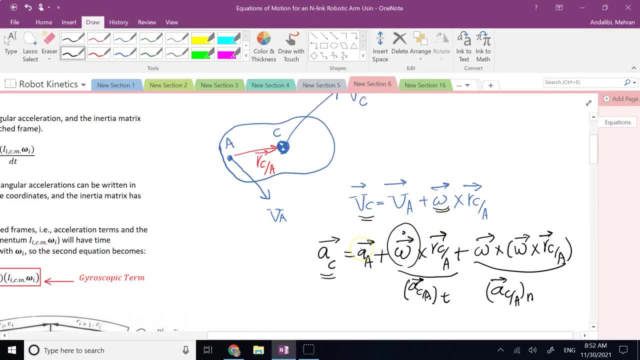 So again, we can do that, But we're trying to not mix the two formulations And here we're trying to stick to the knowledge that we had in dynamics, in Newton-Euler formulation, not Lagrangian dynamics. So why is this good? 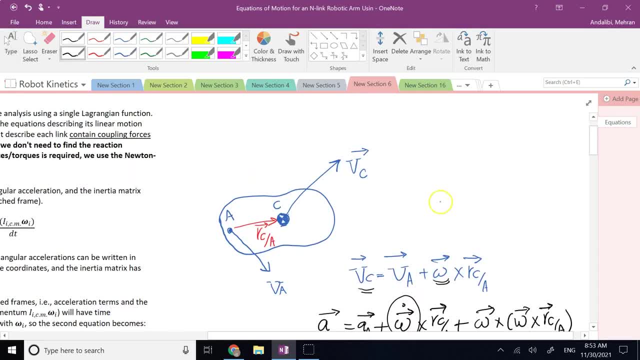 Because typically when you have a robot, then when you go to a link, you typically know the motion of one end of it And then you're trying to find the motion of another end, or the centroid. Let's say here, if it's, 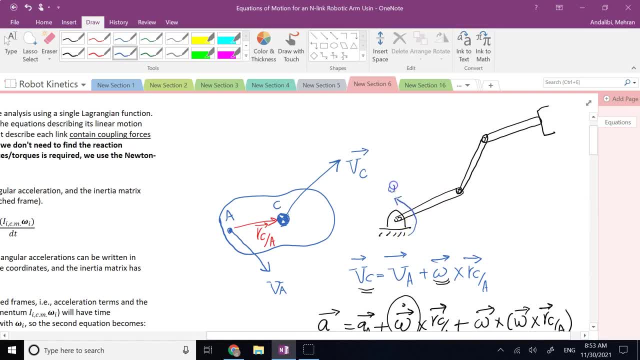 if I know, let's say, the omega of the first link, omega one right And V of A. A can be considered as pinpoints because pinpoint has zero velocity. And if I know omega, then I can clearly find V of C1.. 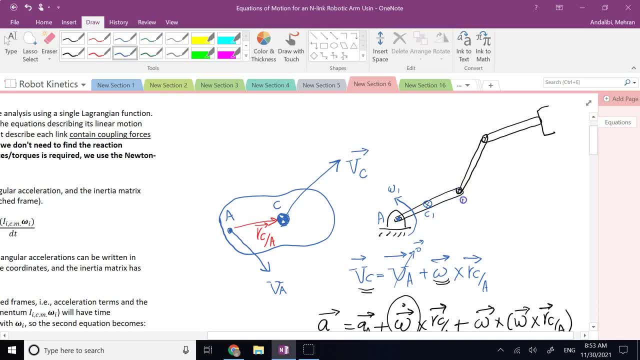 And when I find V of C1, I can also find V of point B, the next joint. And when I have V of B, if I know omega two, then again I can find what V of point C2, as well as this point. 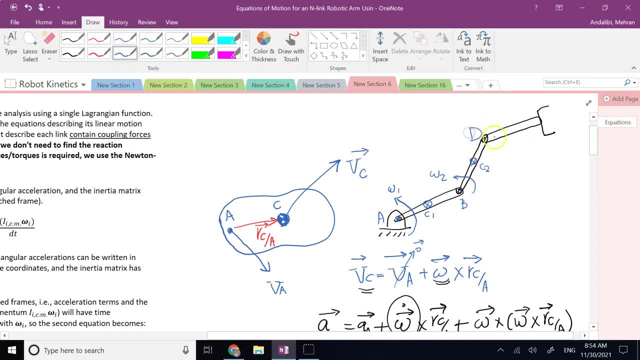 you might call it something else, maybe D, And once I have D and I know omega three, I can find what V of this C3, as well as the end effector, Correct. So that's what we are going to do in this formulation. 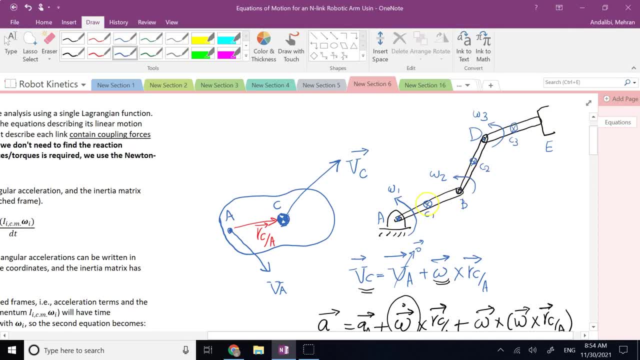 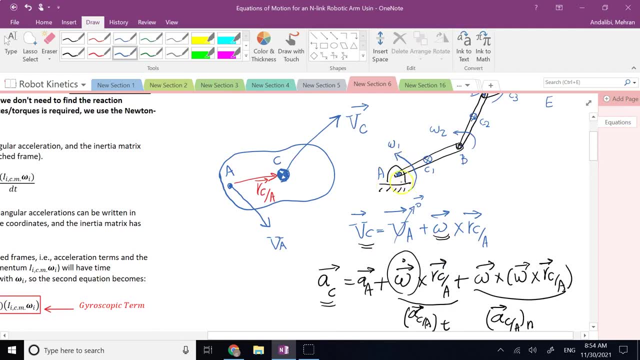 is called the recursion. And so we start basically our motion analysis from the base. because the base is stationary, We know it has the stationary point on the base has a V of zero and A of zero. So we start from there And then go one by one. 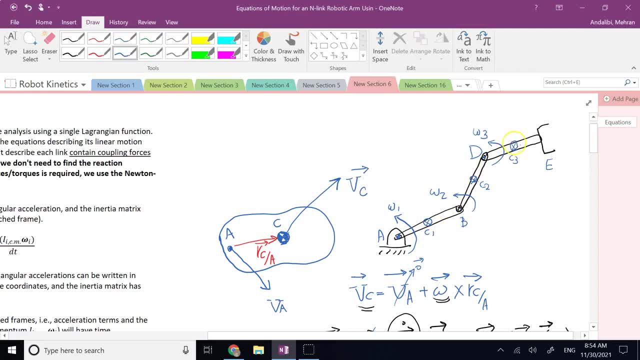 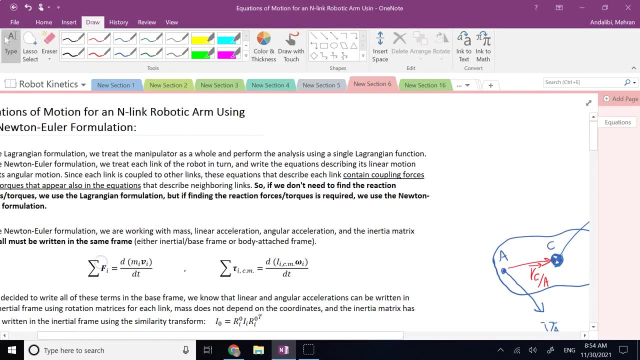 all the way to the last link, And we calculate the velocities or the accelerations of all of the centers, especially the acceleration is what we care about This one, Why? Because that is what you will see in this formula Here. we assume that for a robot, 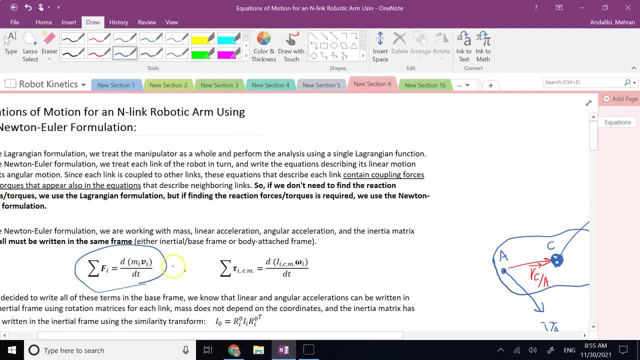 the masses are constant. And when mass is constant, then this is going to be what It is going to be: MI, derivative of VI, which is going to be AI, But A of which point On the rigid body, That's, acceleration of the centroid. 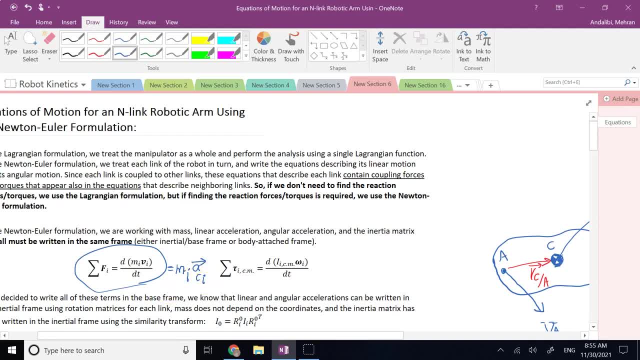 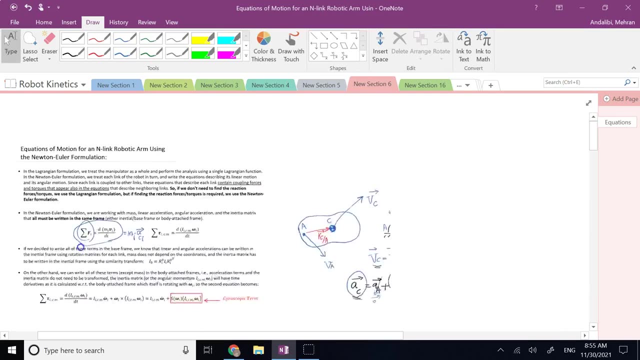 A of CI Correct Centroid number I. So you see if I can find acceleration of centroid I multiplied by mass of link I, that's sum of the total forces applied to that link I. So definitely I need acceleration And, as I said, 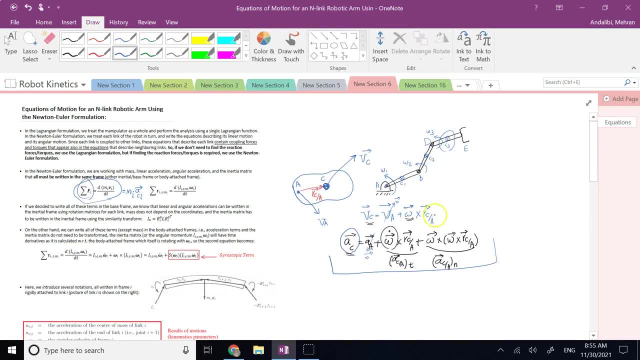 I will do it through this formula. Now, why do I need to do a velocity analysis also Many times? because not always you have omegas for each and every one of the links. So through velocity analysis you try to find omegas. really. 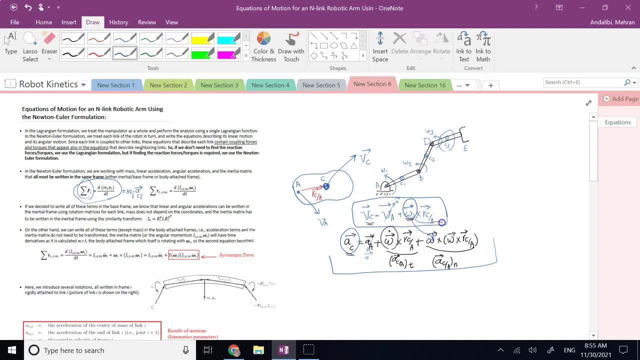 And you need omegas definitely in your acceleration analysis. So we always do velocity analysis, then followed by acceleration analysis. to give me A's And masses are typically given. then I can find the forces on the rigid body, including the pin forces. 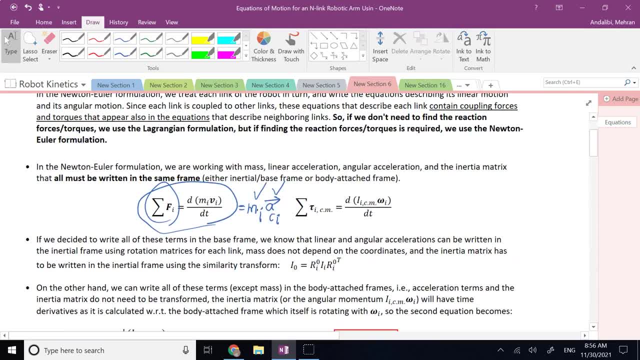 Now, what about the torque equation? Well, the torque equation similar thing, So it depends on, as you can see, omega, which we could find through velocity analysis, and I Now here. there is something that we need to say about I. 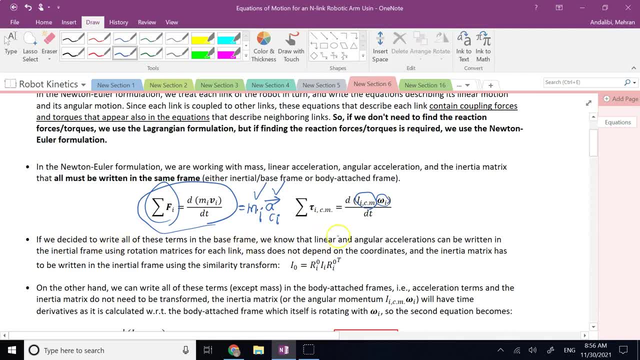 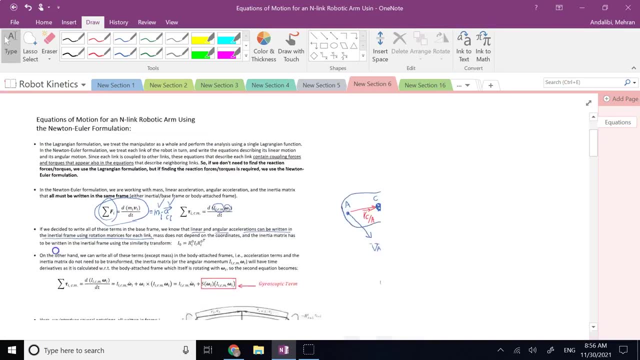 So, as I clearly mentioned for you here, if we want to write everything in terms of base, then the linear and the angular acceleration can be written along the inertial frame using rotation matrices. Okay, because when you find this acceleration, you have to make sure. 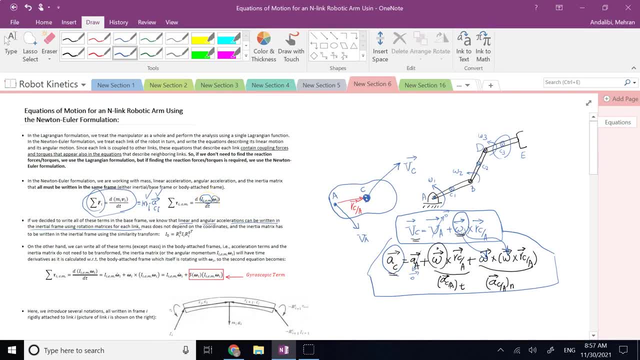 we are writing now everything along the base frame, about the axis of the base frame. So definitely, if this acceleration is somehow measured in a body attached frame, you multiply it by the rotation matrix of that link. take it to the base frame. 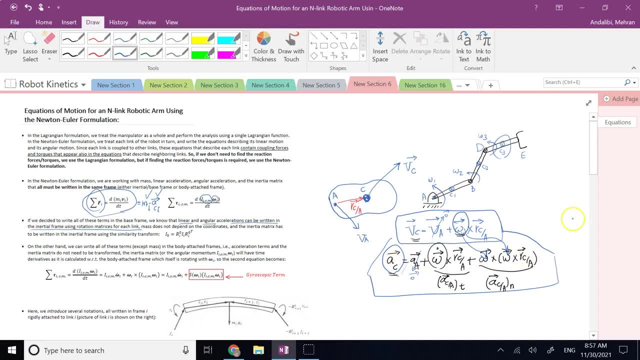 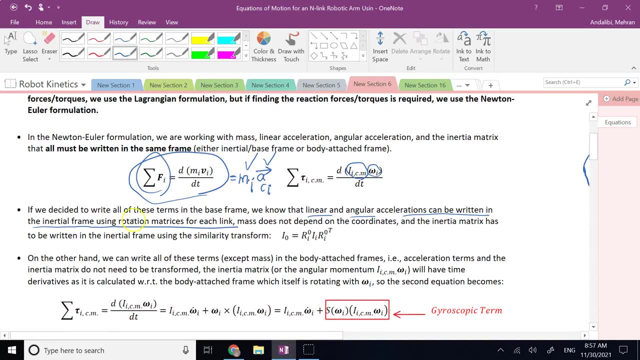 If everything is already written in base frame, then you are good, But we always have the option of what? Multiplying any entity that is written in the body frame, multiplied by a rotation matrix, and take it to the base frame. Mass does not depend on which frame you are using. 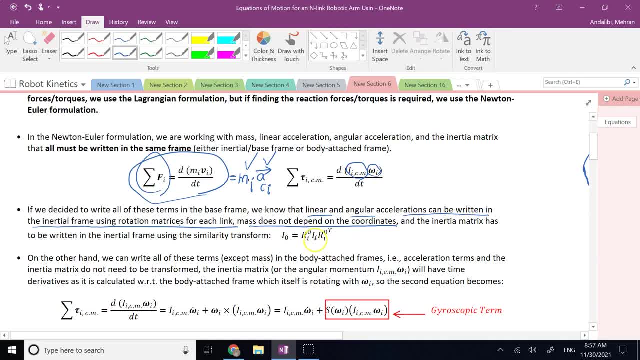 Right, The inertia matrix does, Because if you remember the inertial components of the inertia matrix, there is X, Y and Z in them. So it definitely does. now How do I take this inertia matrix here to the base frame? 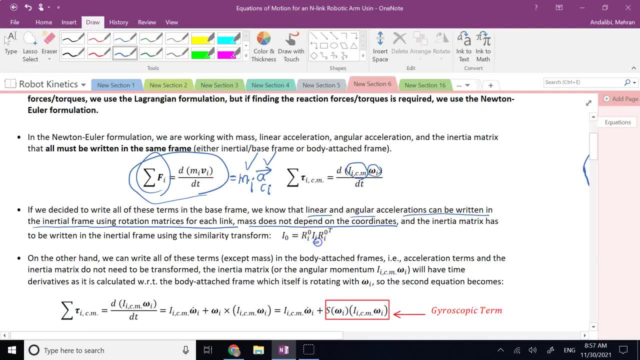 So if I know the inertia matrix about a frame that is parallel to frame I but passing through the centroid and I call it II, If I want to know what is that, I rotation the inertia matrix in the base frame. I need to pre and post multiply it. 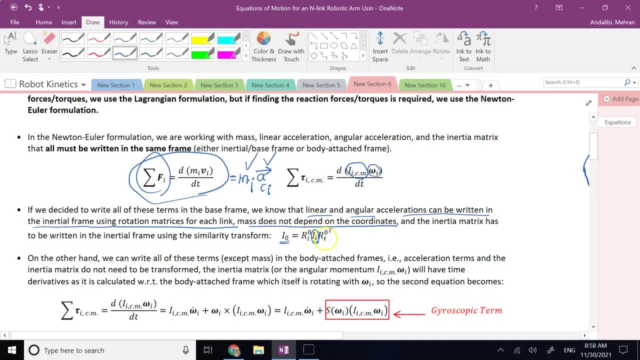 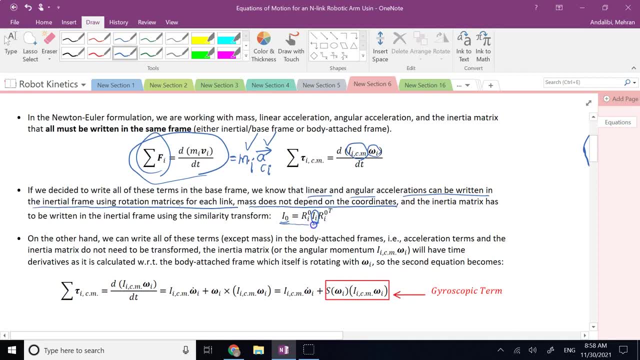 by rotation of that link and the rotation of that link transpose. Okay, So let me clarify this, and we have talked about it in one of my previous videos, when I talked about rotation matrices. we call this guy similarity transform, And I talked exactly about this similarity transform. 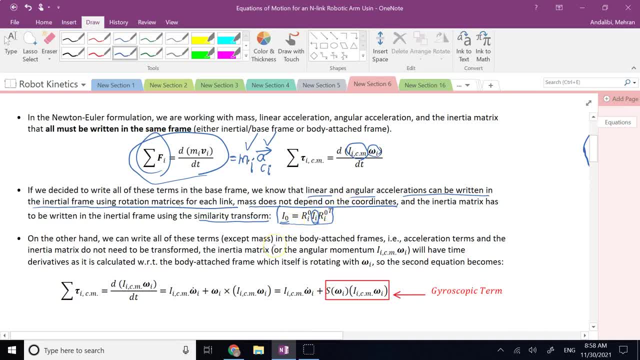 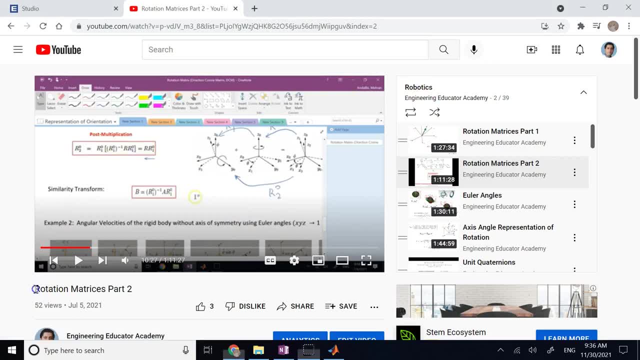 I talked about principal moments of inertia and so on, So let me show you those. So here is the robotics playlist on my channel and this is this video called rotation matrices, part two. And you see, here I define the similarity transform. 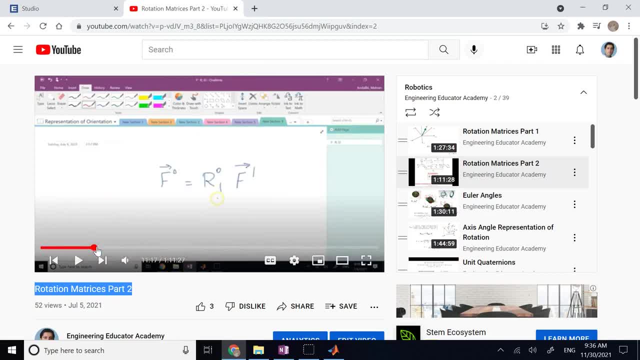 which is exactly what you can see here, And then I used it later to talk about the moments of inertia, As I mentioned over there. these moments of inertia, like when you have IX, XX is the integral of Y squared plus Z squared DM. 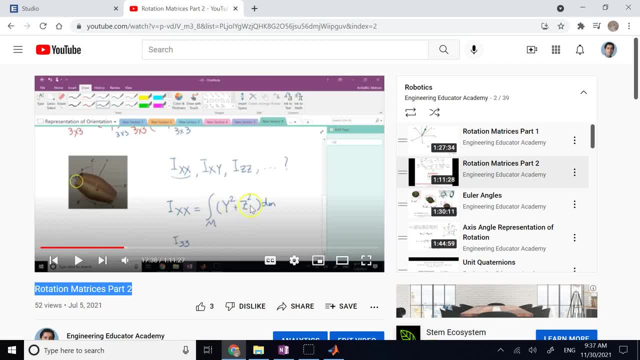 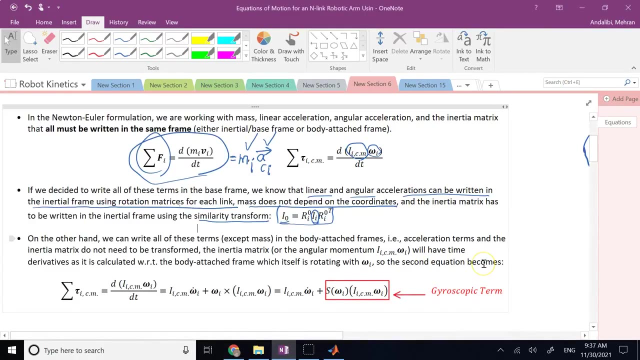 So, depending on which XY or Z frame that you use, these values of IXX, IYY, IZZ or the product terms, they will all change. Okay, So it does matter which frame you are using for the inertia matrix. 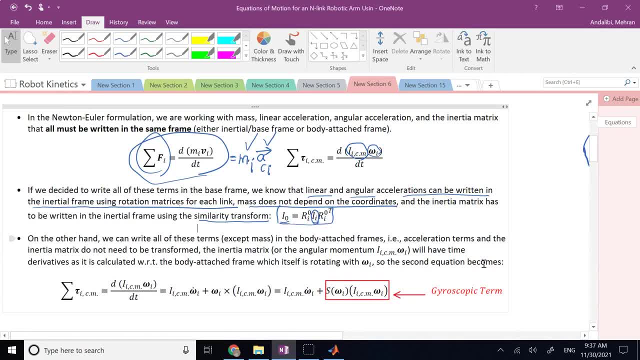 Now, here, the important thing is this: this II, this little one. here again, that is the moment of inertia. matrix for link I. about which frame? About a frame parallel to frame number I attached to that link. 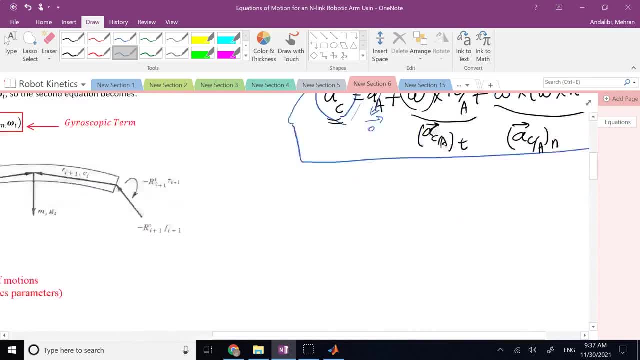 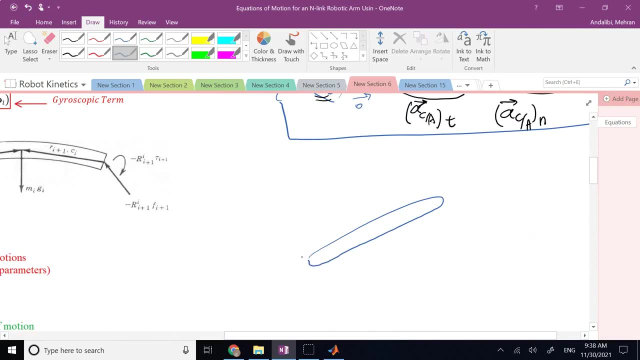 but passing through the centroid. So if this is my link number I- and I have a frame I attached to it, right Like this: let's say So. let's say this is XI, this is YI and this is ZI. 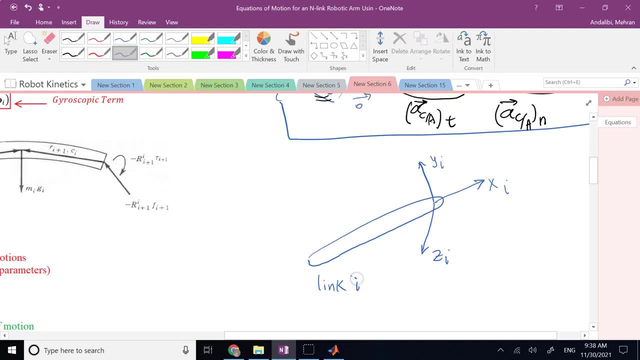 And this is link I. Then this I moment of inertia is calculated about a frame for which the axes are parallel to this: X, Y and Z. So the same X, the same Y and the same Z parallel to the body attached frame. 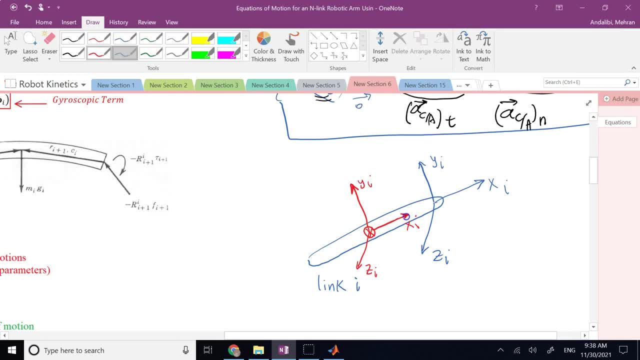 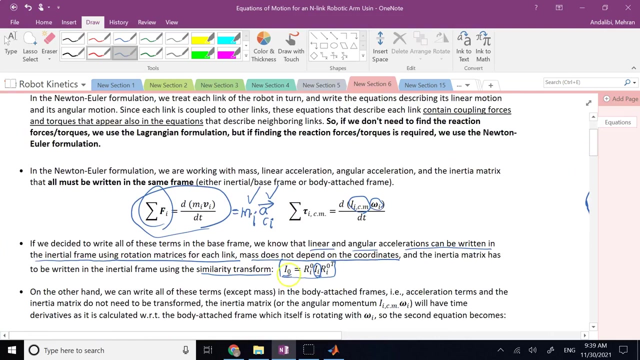 but the origin of that frame is at the centroid. So about this frame is what you calculate? II. And now use the pre and post multiplication by the rotation matrix of this link. I with respect to zero. You use that and then, using the similarity, transform. 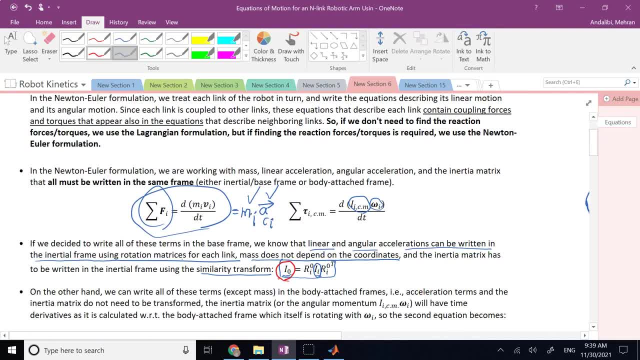 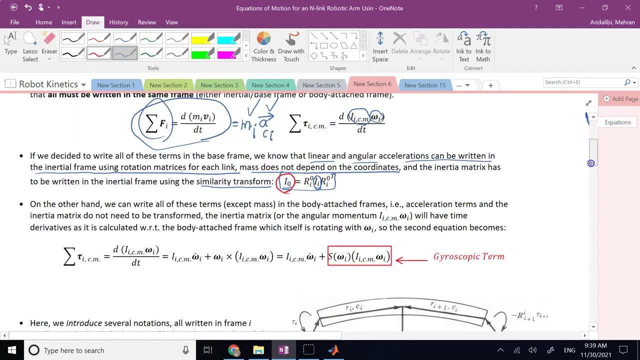 you calculate the moments of the moment of inertia matrix for that link, but in the base frame. Okay, so this is everything if you want to do it in base frame. On the other hand, many times it's easier to calculate many of these entities. 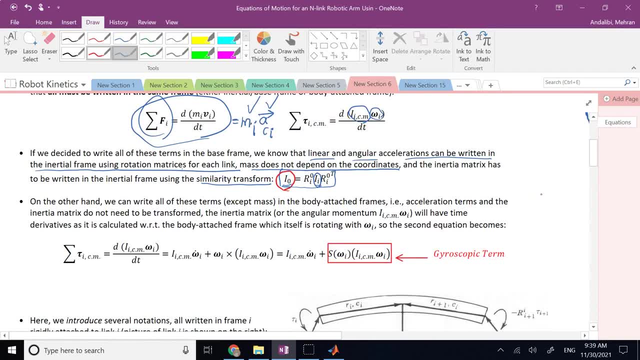 in the body attached frame. You might say why? Well, the reason is this: If you paid attention here for my omega and V, when I want to write them in the base frame, I have to use the rotation matrix for each link. 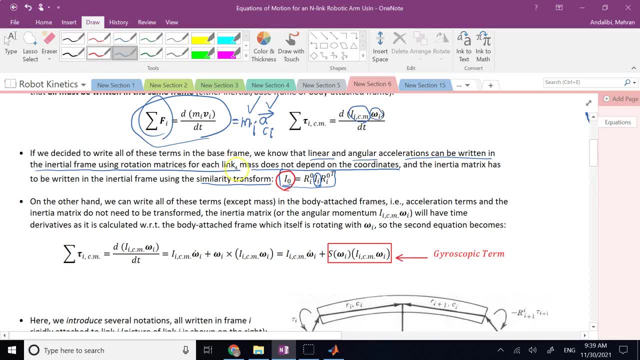 and then take them to the base frame, correct? So I have to basically take my omega and V to the base frame using rotation matrices, pre multiply by rotation matrix. But when I'm writing everything in the body attached frame, guess what? I do not need to transfer V and omega. 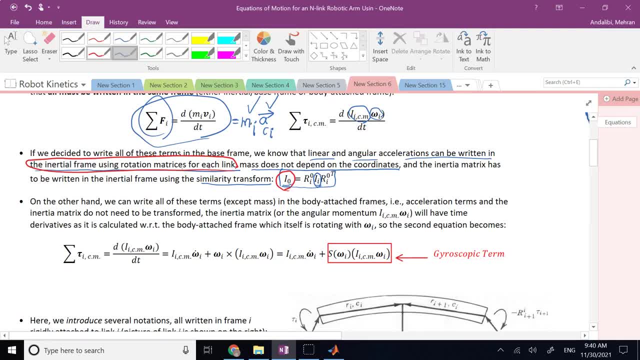 because they are already in that frame. Okay, so I mentioned that for you, that one, That the acceleration terms and the inertia matrix do not need to be transformed. Instead, you might say: well, that's perfect, Nothing needs to be transformed. 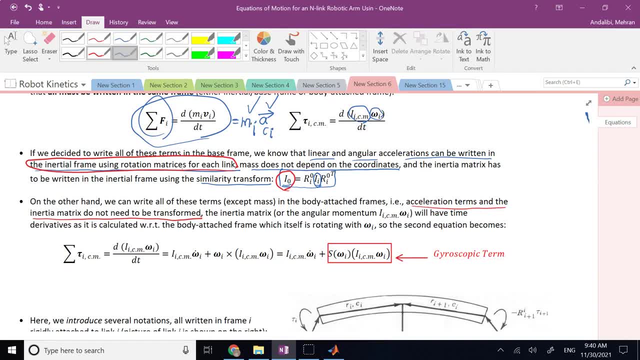 The mass never needs to be transformed. V, omega, A, nothing has to be transformed. That's right. but there is one caveat here. What is the caveat? The caveat is here: when you take time derivative, This inertia matrix that you have, 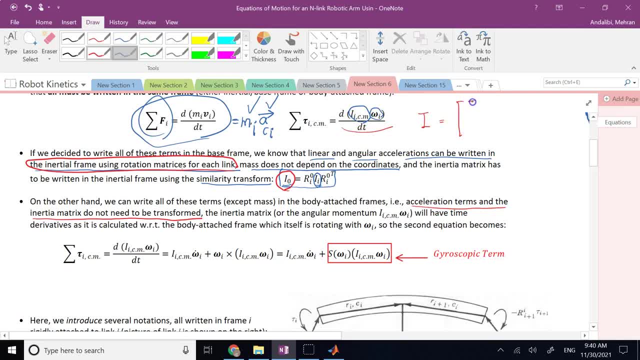 right, which is like, as you know, I X, X, I Y, Y, I Z, Z, and then the product terms correct: I X, Y, I X, Z, I Y Z. 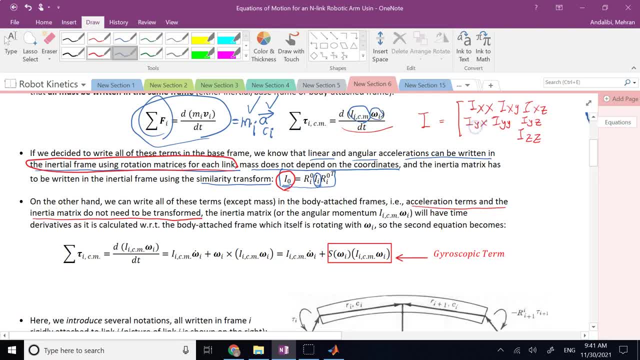 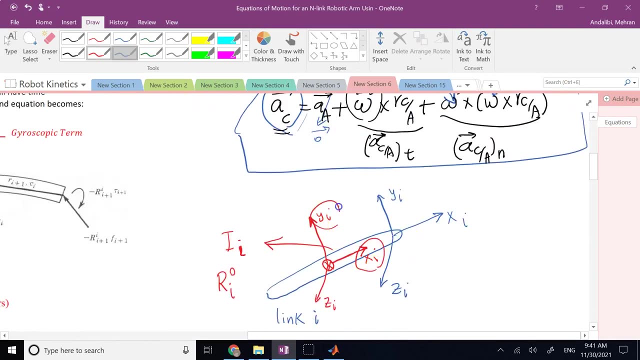 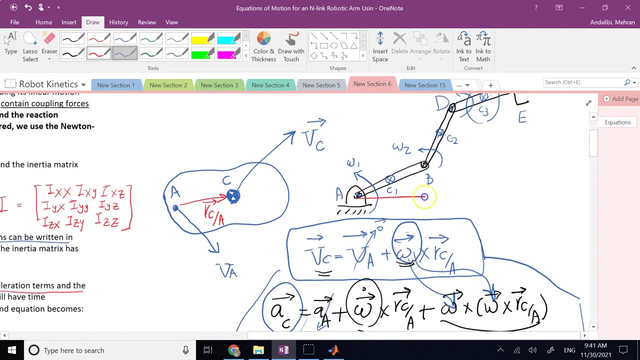 and then the mirror image of that, This matrix. remember, when we are using body attached frame, this X, this Y and this Z. they are not constant- X Y Z- like the base frame of the robots. They are different than this X. 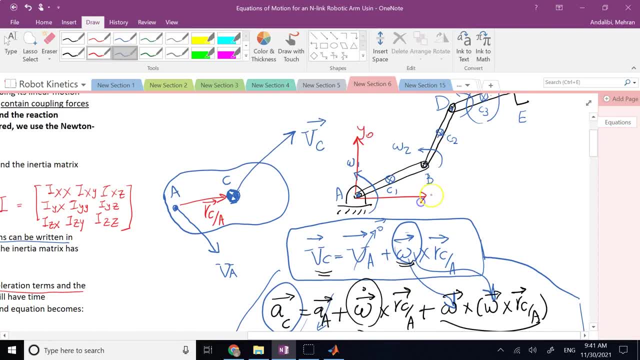 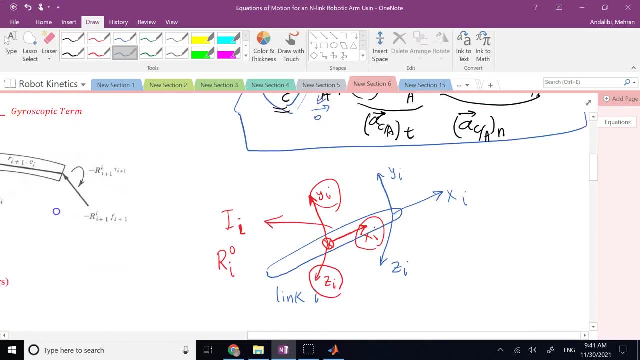 and this Y and Z, This X, knot, Y, knot and Z, knot. they do not have time derivatives, They do not rotate. These guys do So if I say what is like this X, I hat, or the I, for example. 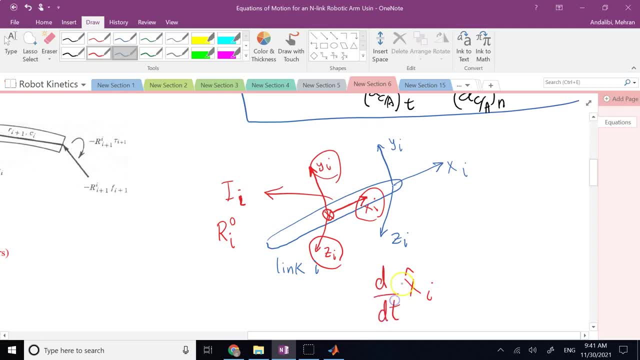 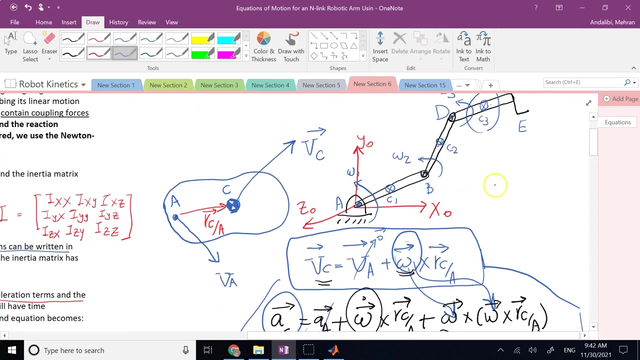 does this guy have a time derivative? The answer is absolutely. It is equal to omega I cross that X I hat, Because that vector is rotating with angular velocity. omega I in the space. But here if I say how about this X, knot. 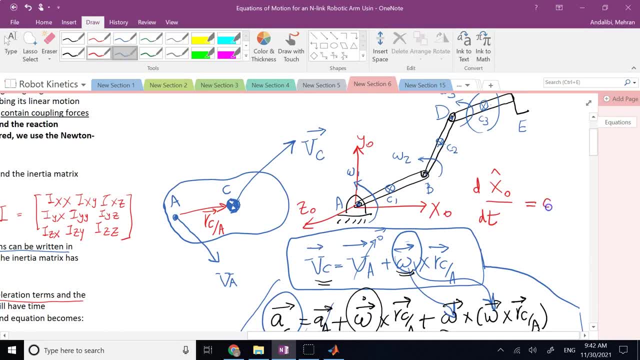 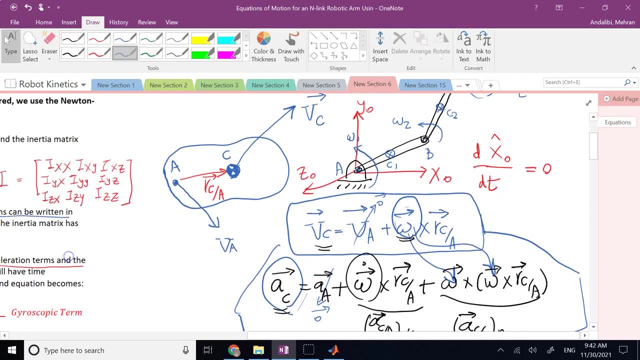 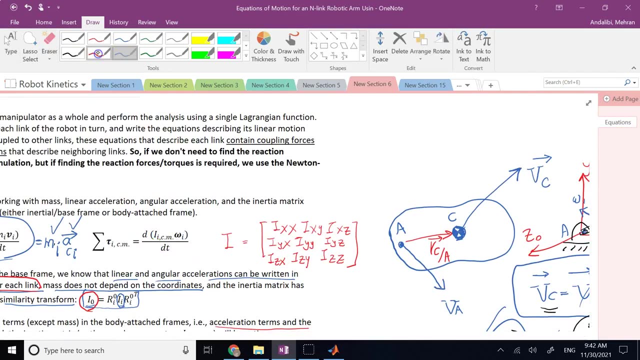 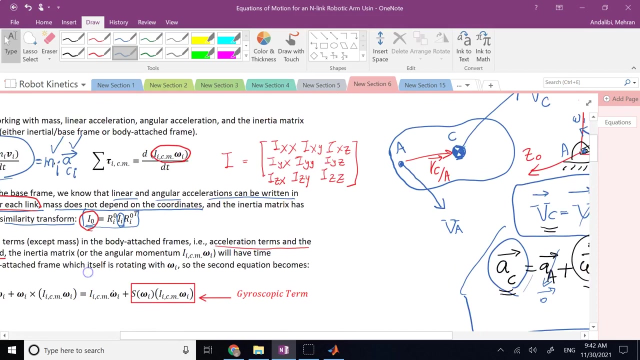 Does this have a time derivative? And the answer is no. It is a fixed vector, Fixed magnitude one and fixed direction. So for that reason, this entity here, this I omega, when you calculate the derivative of that, it does have two terms in it. 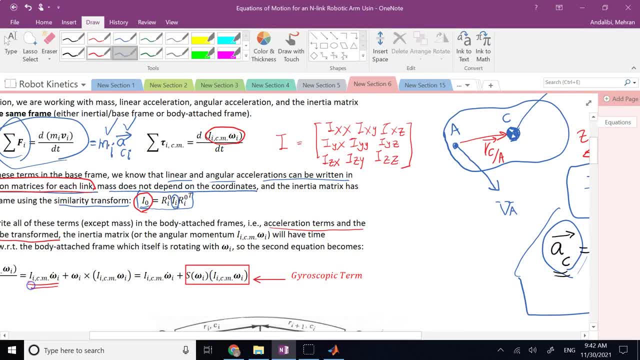 One is this guy here, which comes from the fact that omega does change with respect to time, You can have alpha. And the other one is because this whole entity, which we call angular momentum or H, this H is on a frame that is rotating with omega. 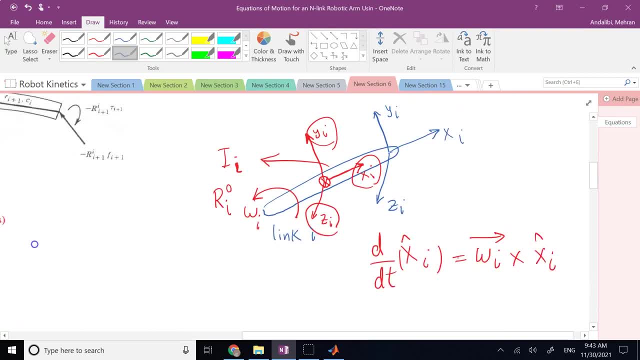 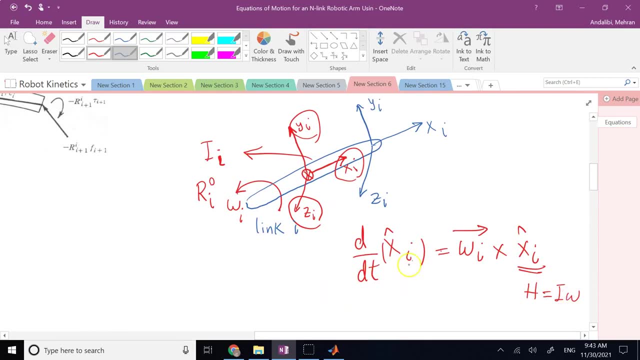 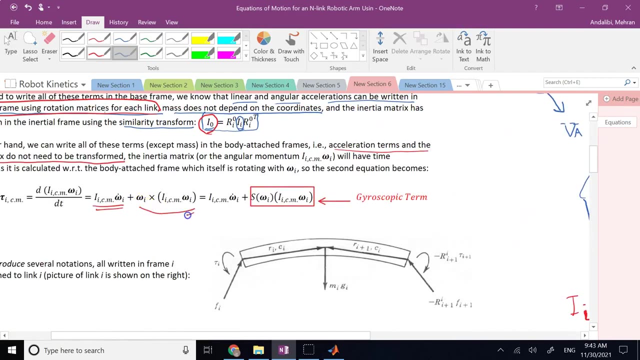 So time, derivative of that H is going to be omega cross H, So instead of this you can replace it with H, And remember H is I times, omega. Okay, So that's another term that you have And that is what you can see here. 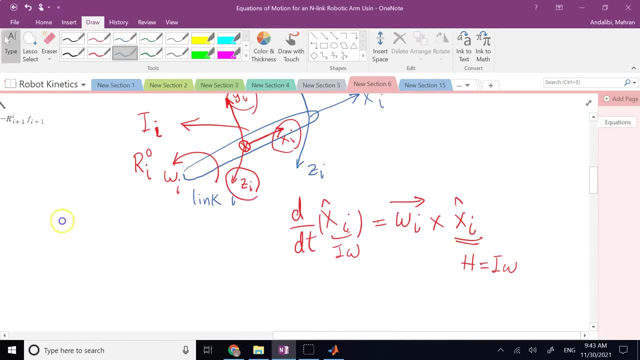 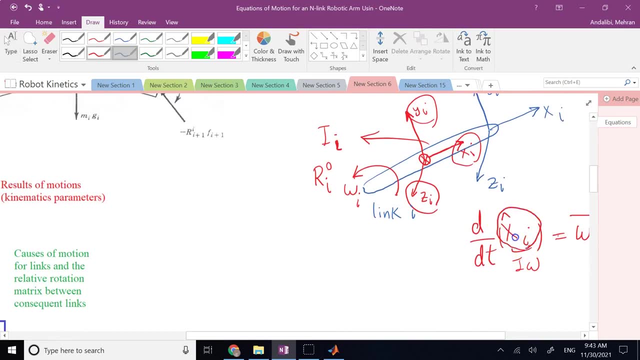 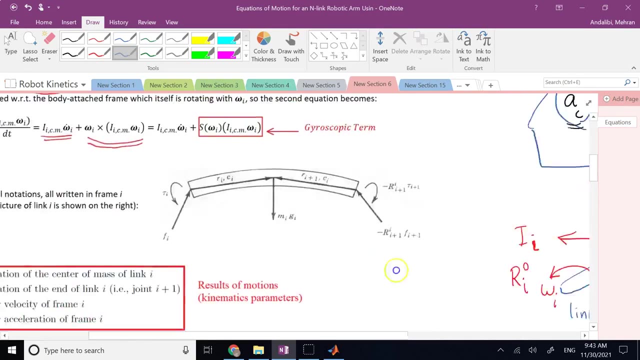 Now you might say: here I only have one term. How come here you have two terms? Well, because in here this unit vector had a constant magnitude. The magnitude of it did not change, Only the direction of it did. But in here, 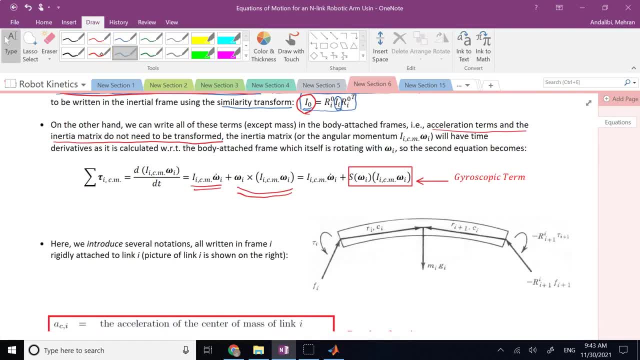 this vector, I, omega, can both change magnitude and direction. The magnitude of it can change because the magnitude of omega can change with respect to time. The direction of it can change because the direction of components of I or the frame XYZ of link I can change. 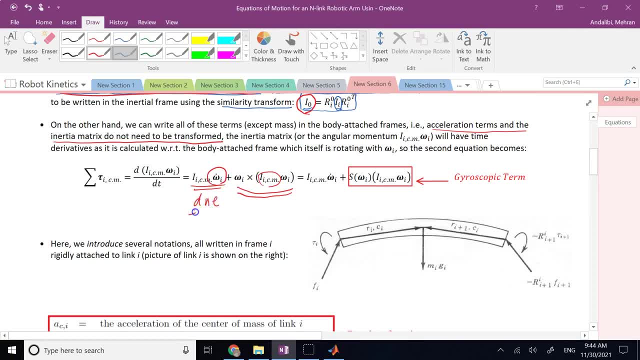 So this is due to change in magnitude, magnitude of what? The whole vector, Because omega changes, then I omega does change, And this one is due to change in direction. Okay, So here you have two terms And then, based on what we learned, 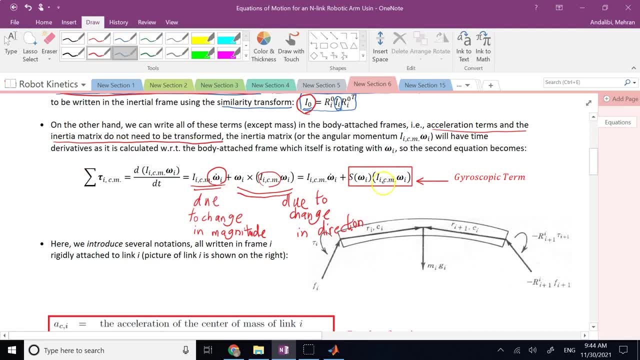 about the skew symmetric matrices, one way to calculate A cross B. right, if you remember from our introduction to skew symmetric matrices, A cross B can be written as skew symmetric of A times B, And that's exactly what you can see here. 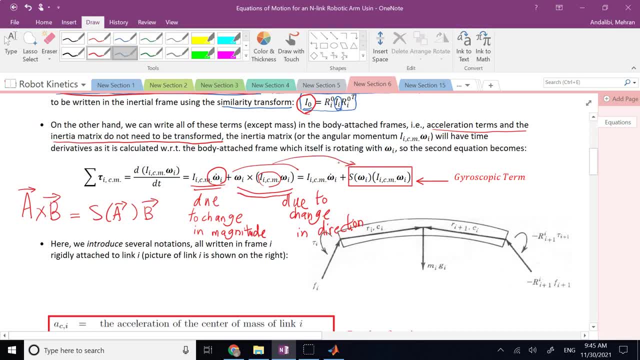 This one is written like that. So the body attached frame has advantages. Many of the things do not need to be transformed. But when you come to time derivative of the angular momentum, you have two terms, So we have to keep that in mind. 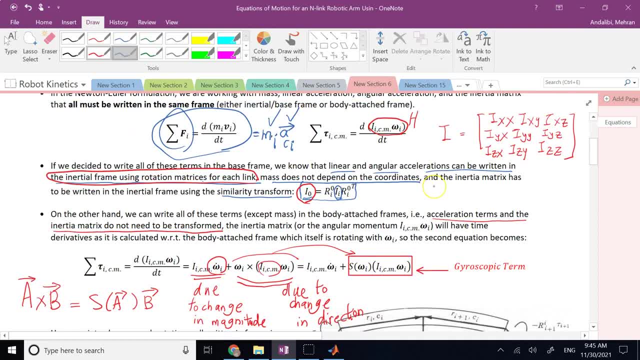 So in general, there are two ways you can handle it: Write everything in base frame or write everything in body attached frame. Typically, the form of the body attached frame will be a lot easier and nicer than the base frame, And that is what you are going to see. 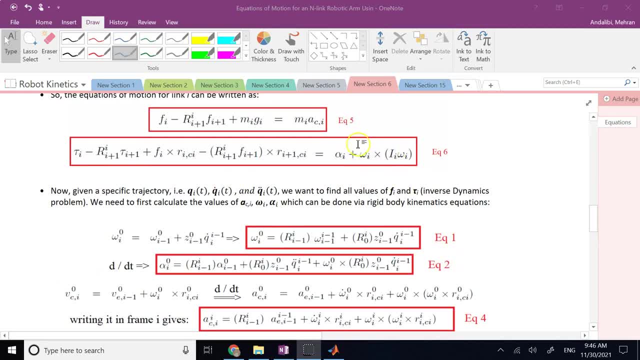 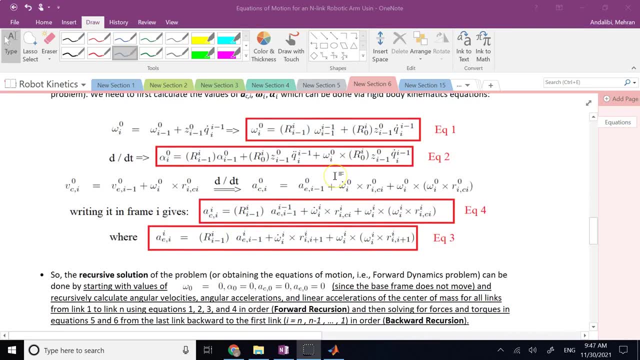 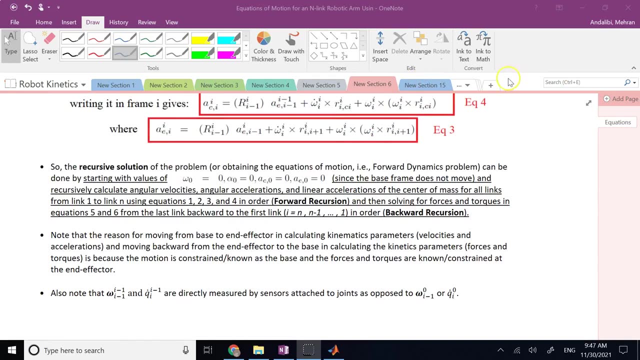 in these derivations and these formulas, equations one to six which we called forward, and inverse recursion formulas. So here everything is written in the body attached frame basically. But I can show you also if we use the inertial frame and write everything in the base. 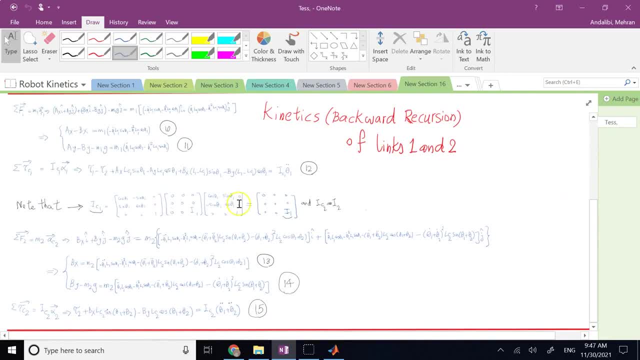 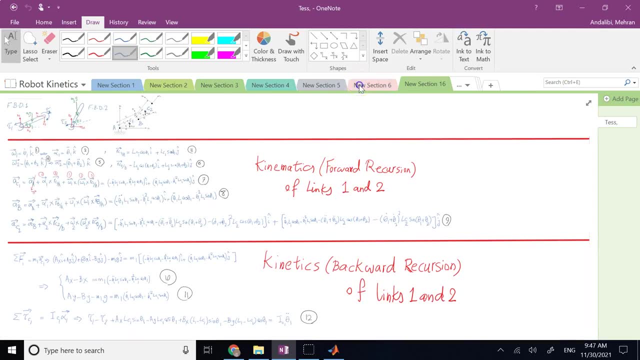 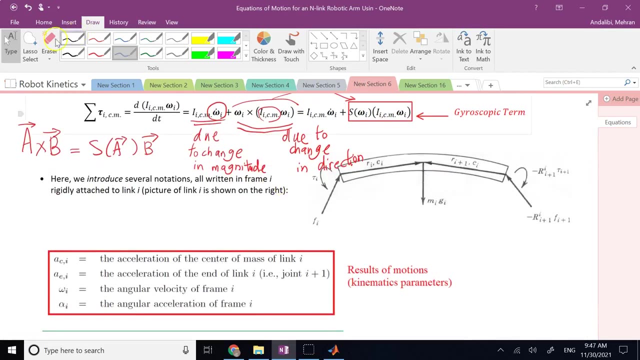 or inertial frame. we can get another way to formulate this. So in this case we are going to look at the general formulation for body attached frame. So here we use some notations and symbols. So here this is what you can see. 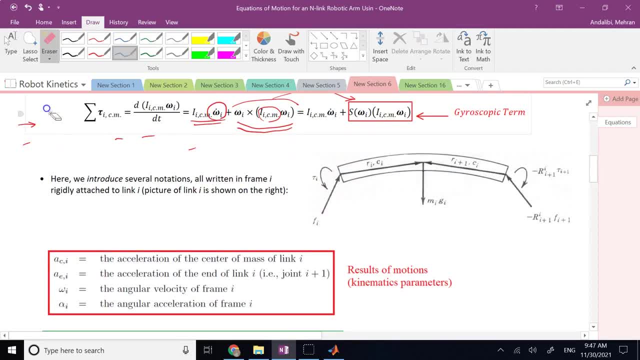 for link number I. This is the square And here we are going to look at the general formulation for the body attached frame. So here we use some notations and symbols. This is the schematic of link number I And the centroid of link I. 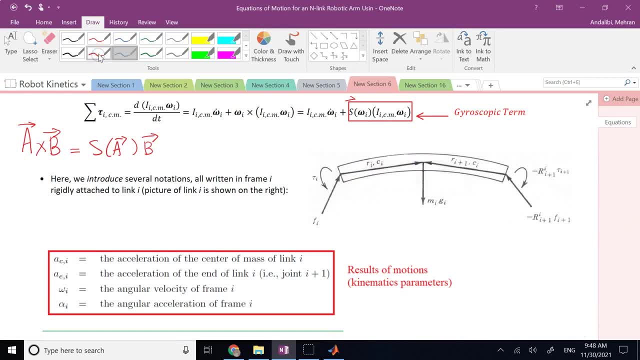 here is shown. So this place here is the centroid And these two points here and here are the two joints that that link has and it's connected to the member before that and after that. So this one connects it to link number I minus one. 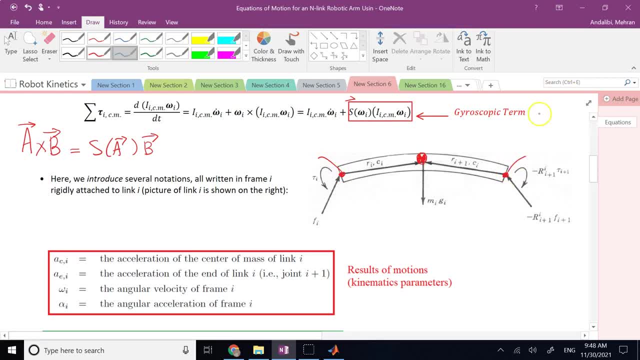 This one connects it to link I plus one, correct? So this is the joint with link I plus one And this is the joint with link I minus one. And here we use two vectors: R I- C I and R I plus one and C I. 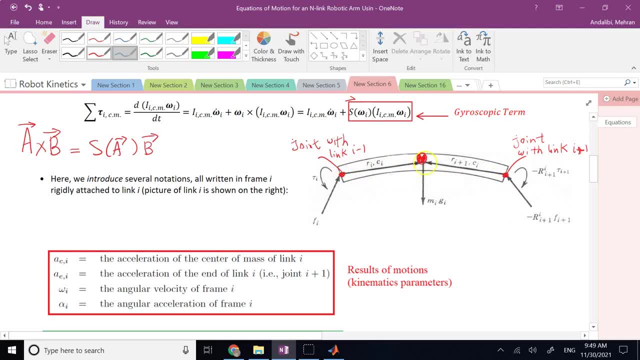 And these are the vectors from each one of these, And these are the vectors from each one of these joints to the centroid of the link. Here, the only force, the body force that is applied to the link I is gravity. M, I, G, I. 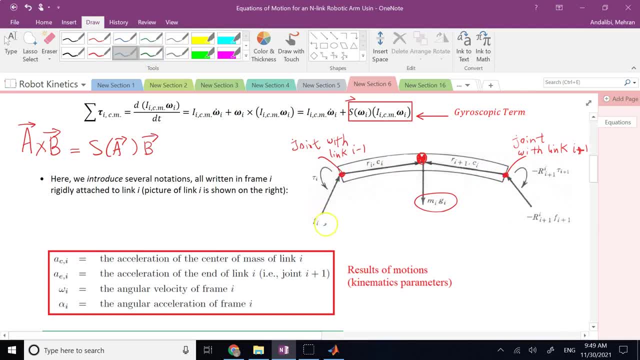 There are two reaction forces on the two ends: F I and F I plus one. These forces are coming from what? From the adjacent links, link I minus one and I plus one. They are applying those forces through the joints to this link number I. 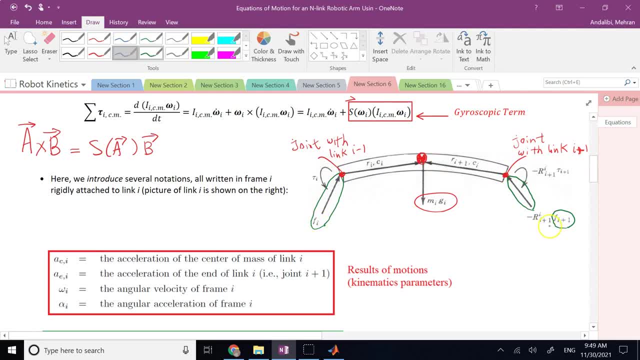 Now you might say: why is it that you multiplied F I plus one by a rotation matrix? Because here this F I plus one is actually written in frame I plus one. So it is actually like this F I plus one, but written in frame I plus one. 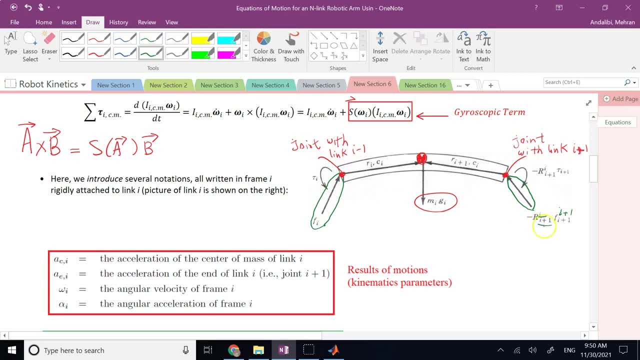 So when I multiply it by what? By rotation of I plus one in I, it is like I'm bringing that force F, I plus one, but write it in frame I, Because everything here has to be written in frame I. That's why you see G, I, F, I. 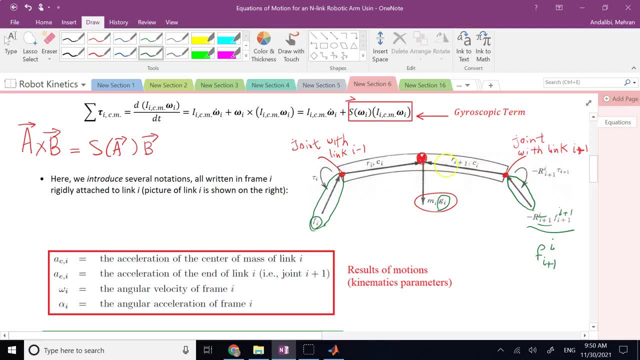 Every force, anything, any torque, has to be written about the axis of frame I. That's why I multiplied. And you might say: what is this negative doing? Well, that's action and reaction. This force is applied by this joint to link I plus one. 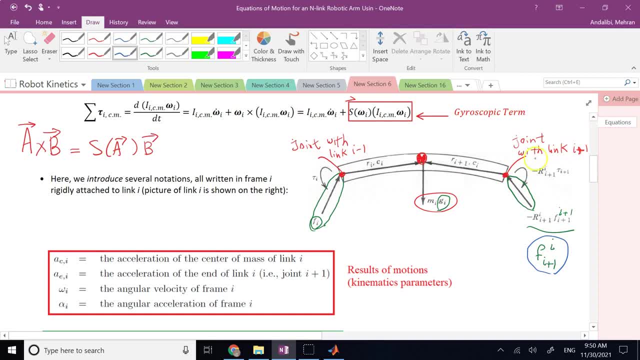 from link I And then the reaction of that from link I, plus one is applied to link I. So this negative is because of the reaction. The same thing goes for the torques. Here you have torque I, which is the torque applied at joint I by the motor. 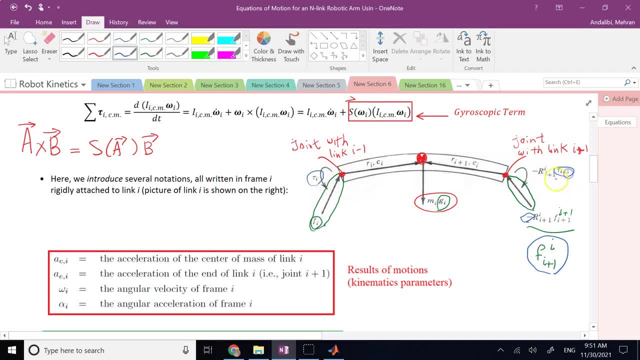 And then torque. I plus one is the torque that is applied to link I plus one through the motor. But the reaction of that is applied to what Link I? And again, I use a rotation matrix to convert that torque that was already in frame. I plus one. 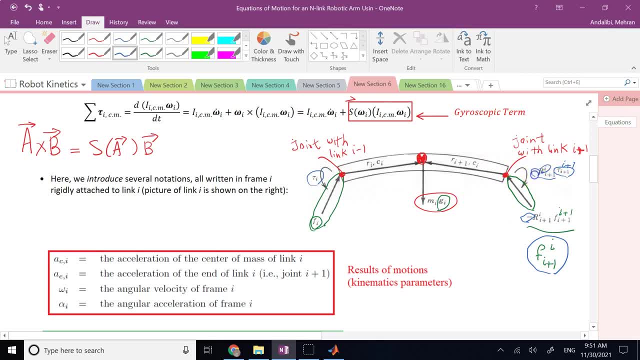 bring it back to frame I, And negative again means reaction. So hopefully it is clear where each one of these five forces or torques coming from and why they are written the way they are written. Alpha and omega are definitely angular and angular velocity and acceleration of frame I. 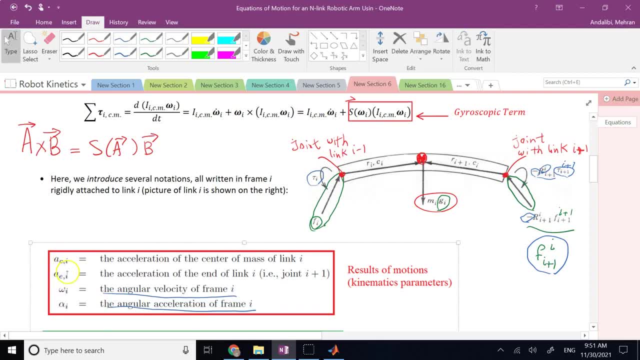 And A of C I and A of E I are what? A of C I is definitely, of course, the acceleration of centroid of link I. A of E I is the acceleration of end of link I plus one. So basically, acceleration of this point. 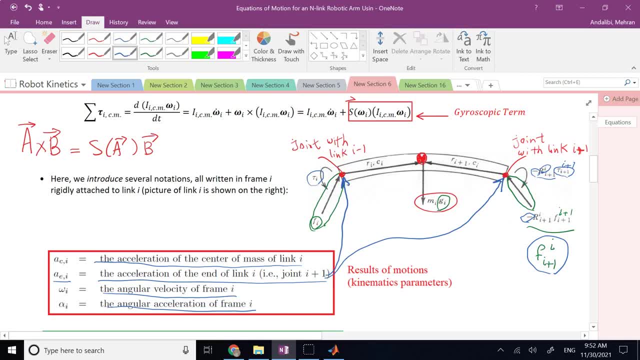 Or this point Right, Depending on what this I is. If it is I minus one, it is going to be this. If it is I, it is going to be this one. So when I say A of E and I minus one, 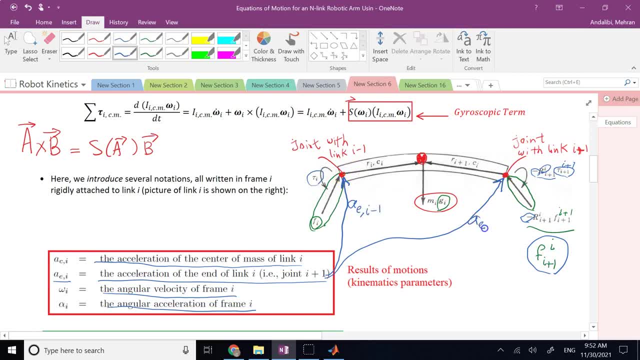 that is this point. When I say A of E and I, that is the right point. It is one of the two ends Good. So that is the notation. G is clear, F, tau is clear. Rotation of I plus one. 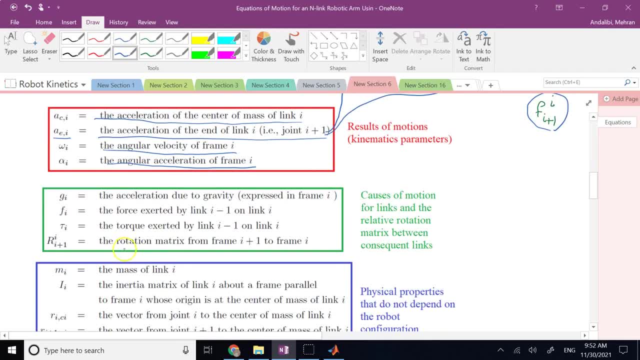 with respect to I. That is the rotation of one link with respect to the adjacent link. In terms of Denovit-Hartenberg notation, this R I plus one to R I. we showed it with matrix A I. Okay, That is the same notation. 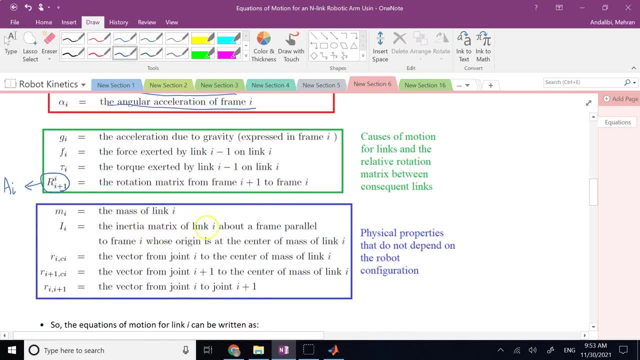 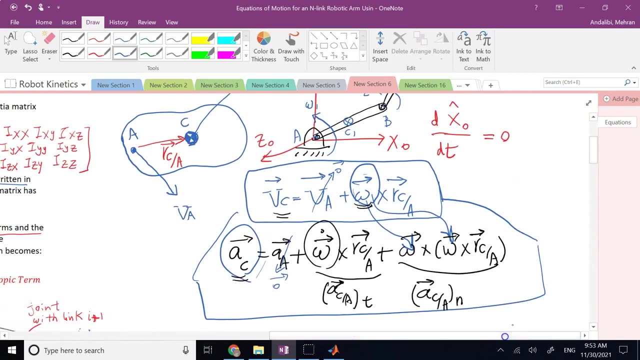 Mass is clear. I is clear And again, pay attention- The inertia matrix of link I about a frame parallel to frame I, but origin at the centroid. So it is exactly this guy that I mentioned for you here. Right, This one. 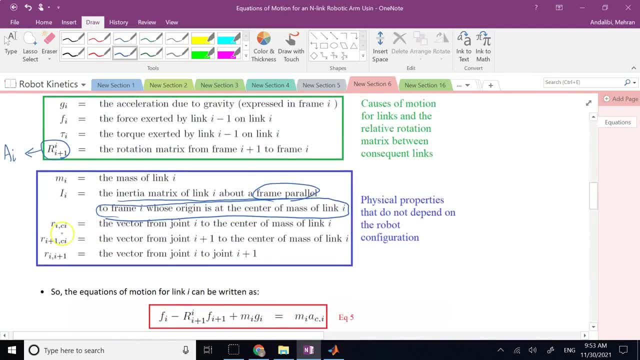 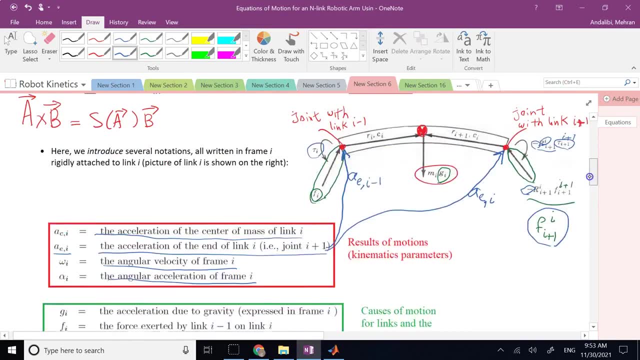 And now going back, these vectors are also clear. Right, There is R of I, C I. R of I plus one C I, both of them you can see here. And then R of I I plus one, which we never use. 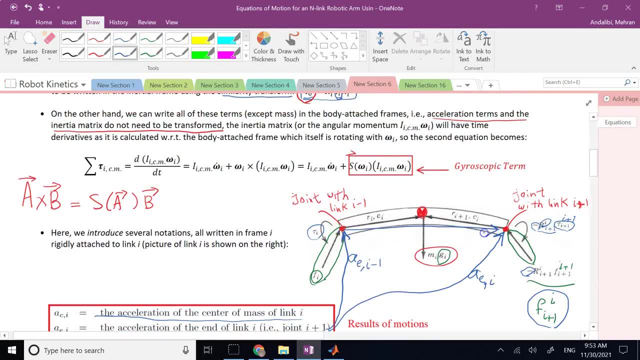 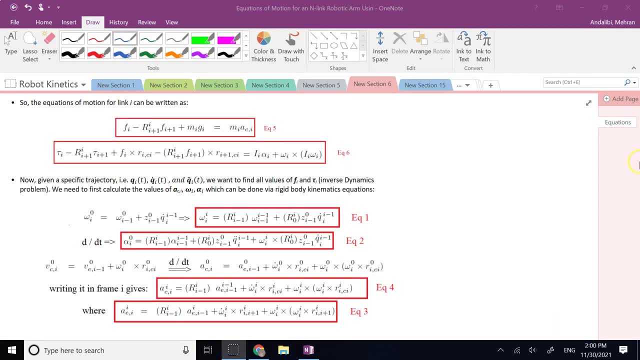 but that is the vector directly going from one joint to the next. So this is like R of I and I plus one. So now let's look at the equations of motion. So if you look at the free body diagram of link I, 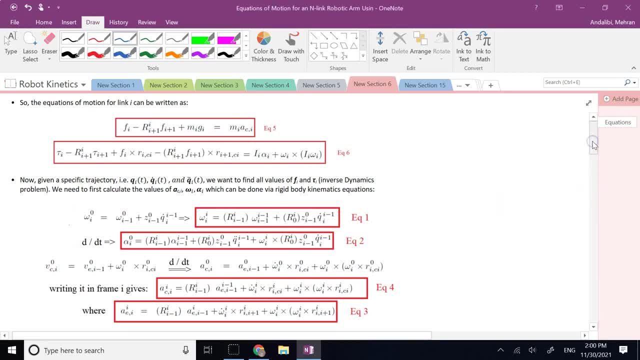 there are three forces acting on it, The forces F? I and F? I plus one, and then M G, And so some of these three forces have to be equal to the mass of the block times acceleration at the centroid here. So that's what you can see over here. 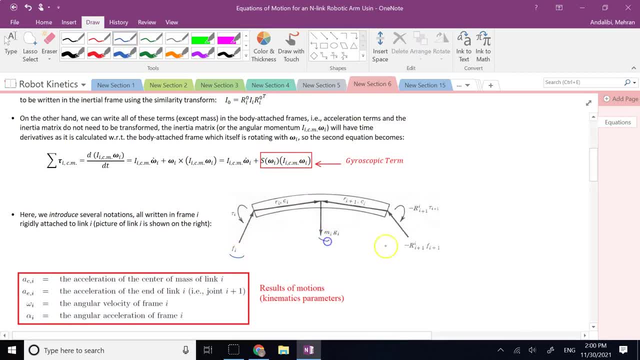 Right, There are these three forces. Also, if you take the some of the moments or torques about the centroid, M G doesn't do anything because it does pass through the centroid. The two torques, T I and T I, plus one, transform back to frame I. 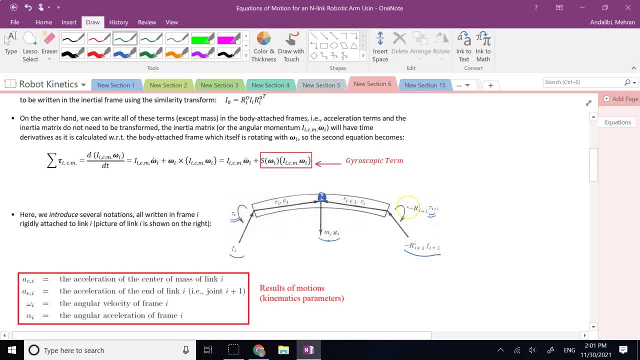 They definitely do something. You have to add them together. They are coupled, And then this force F and F I, F I and F I plus one. they do also create moments about the centroid. For them. we need to use this position vector. 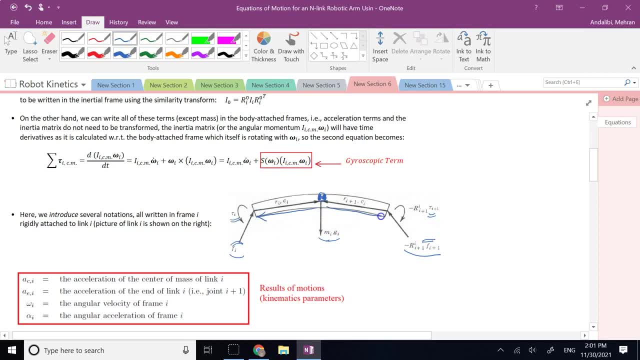 this one Right, And this one We have to cross. multiply those position vectors by the forces And if you look at these vectors, they are the same as R I, C I and R? I plus one and C? I but with a negative sign. 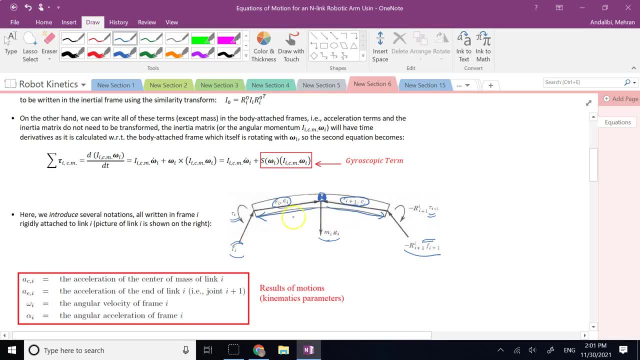 So if I want, let's say the moment of F? I about centroid, it's going to be this vector which is really negative, of R? I and C? I, That's this position vector here, And then cross multiplied by F? I And a similar thing for this one. 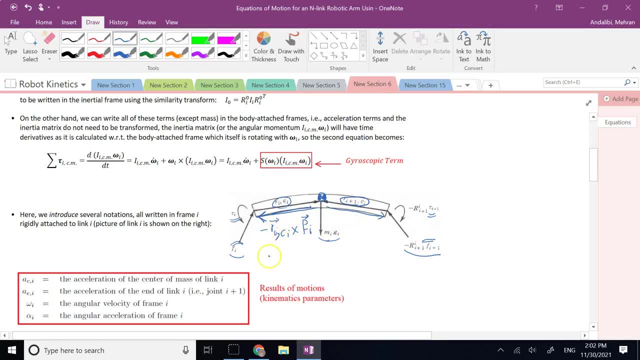 And, as you know, if you change the order of a cross product, the negative sign goes away. So you can also write it as F I cross, R I and C I, And that's what you see here down in the equations of motion. 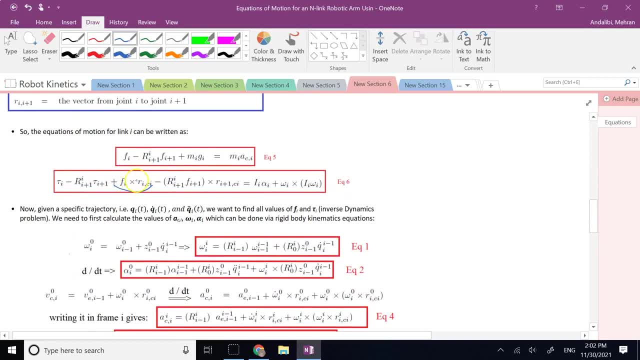 So if you see F cross R, not R cross F, is because of that negative sign and reversing the order. So you see, these are those two couples, the torques. the torques, due to the forces, That is equal to rate of change of angular momentum. 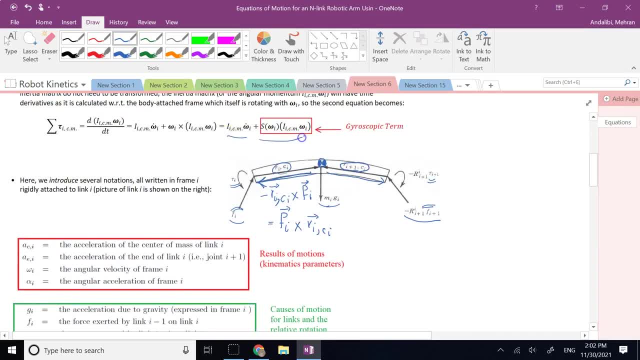 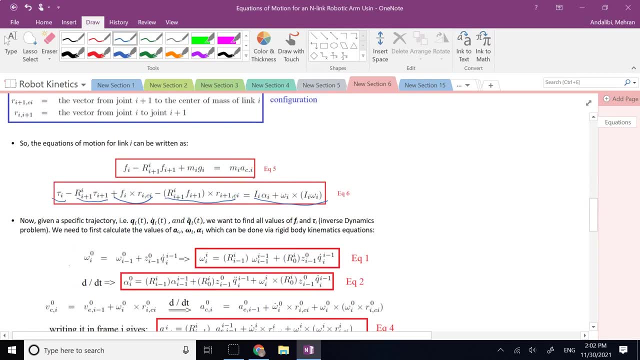 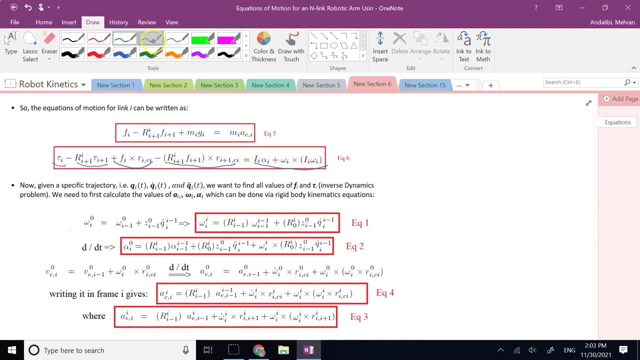 And, as we learned, this rate of change has two terms that you can see down here. So equations five and six are the equations of motion for the rigid body And clearly, if you look at these equations of motion, they need some entities in order to be able to calculate. 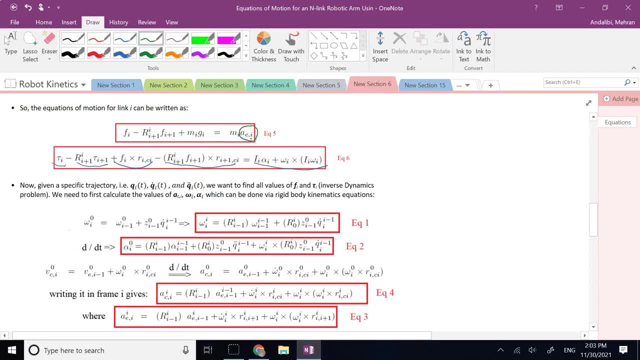 them. One of them is acceleration of link I at the centroid. The other thing is angular velocity and then angular acceleration of each link with respect to either base frame or the body attached frame Right. So I have three kinematics quantities: A. 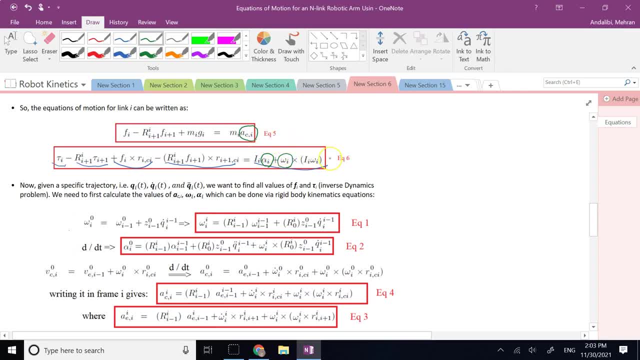 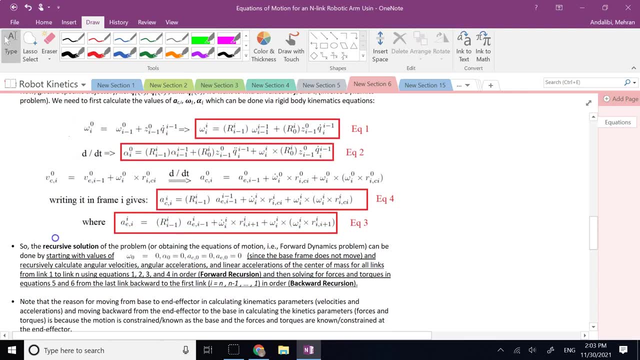 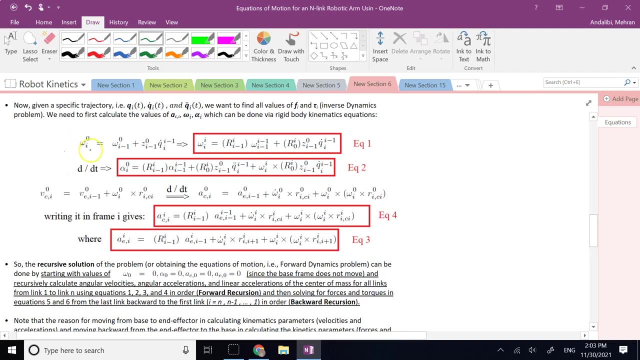 alpha and omega that I need to calculate in order to be able to use equations five and six. And that's where we go to our kinematics knowledge and kinematics equations, the equations that I earlier mentioned for you. So here we say that omega of link I in base is equal to omega. 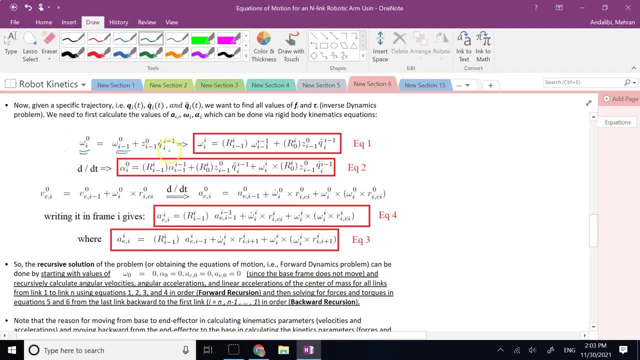 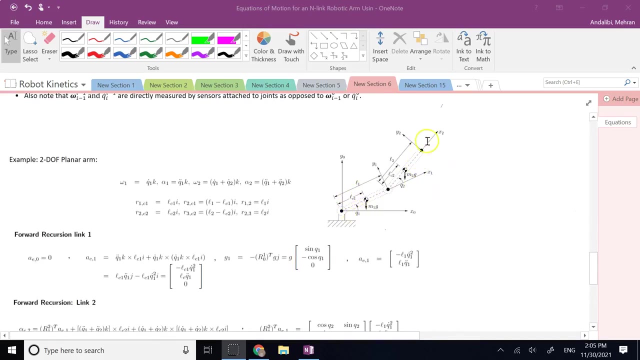 of the previous link in base, plus the RPM of link I, multiplied by the unit vector of that direction Right, So this whole thing is the relative angular velocity between frame I and I minus one. And we can apply that here toward our example two degree of freedom, plan or arm. 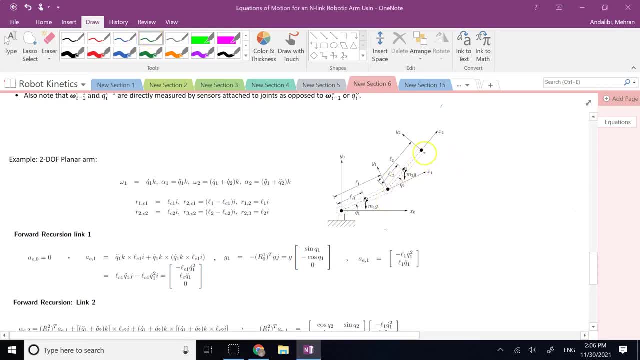 Right. In this case, if I want omega of member two with respect to the ground or base, based on this formula, it is omega of member one, the previous member, with respect to the base, and then plus the relative angular velocity of these two. 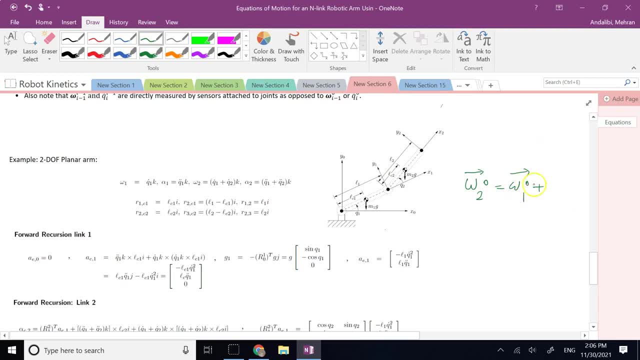 correct, which is omega of two with respect to one. But since everything here is written in frame zero, I cannot really write omega of two with respect to one unless I really multiplied by a rotation matrix of one with respect to zero. So I bring the whole thing down to frame zero. 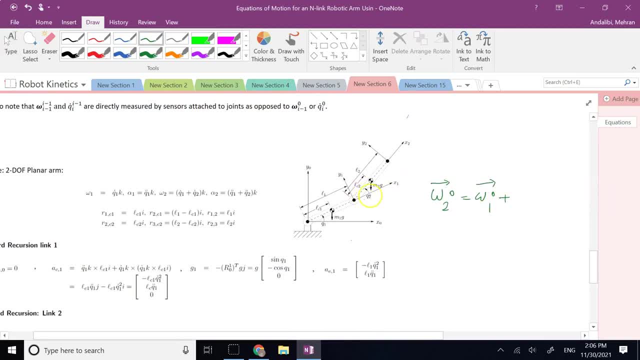 So what I do is I say: well, this link two is rotating with angular velocity, Q dots with respect to one. So the magnitude of the rotation is Q, two dot, and the direction of rotation is the axis of Z, axis of frame one. So there's going to be like this: 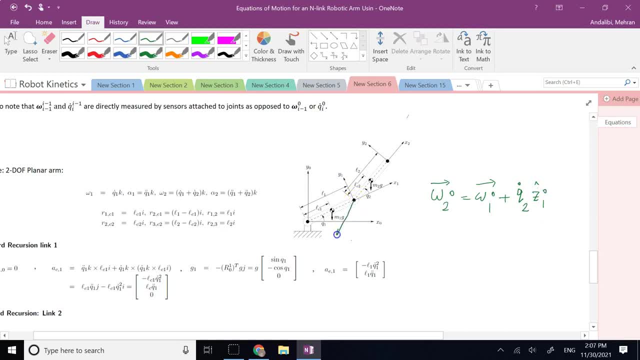 right And clearly here. your Z one is out of the plane, the same as Z zero. That is also out of the plane, right? So this one is. this one is definitely omega one with respect to zero. The magnitude of it is Q one dot times Z of zero. 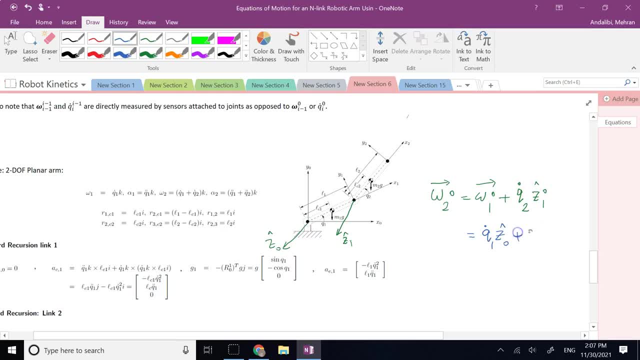 right Then plus Q two dot times Z of one in zero, And clearly, if I call this guy to be K, this one is also K. They are both out of the plane. So it is going to be like Q one dot plus Q two dot. 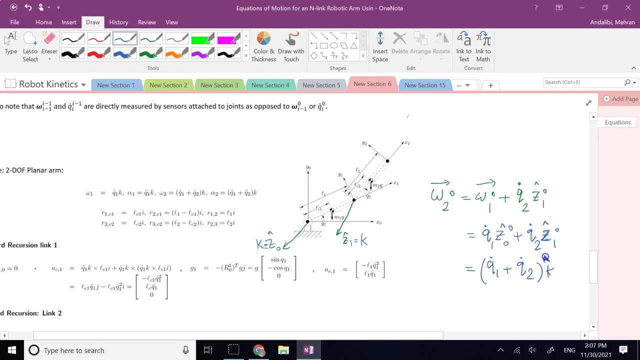 both of it times K And that's what we also know from our previous videos. correct, Because Q two dot is measured with respect to link one, So I have to add both of them together. Know that this Q two dot is not measured from the base. 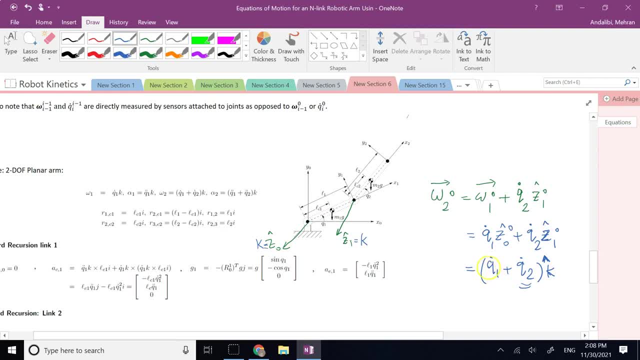 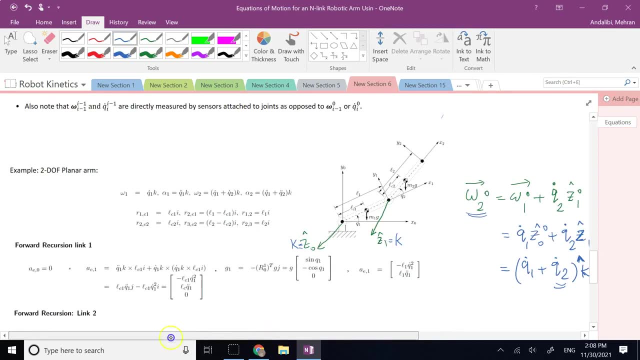 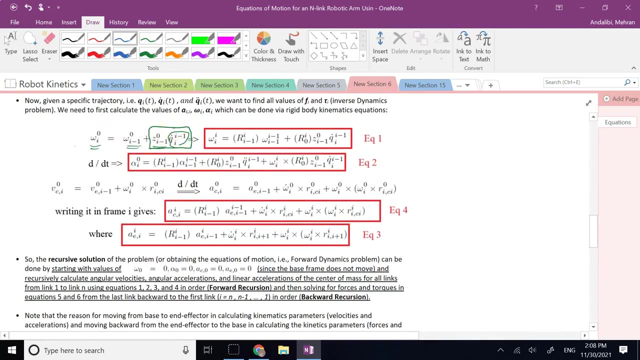 This is measured from frame one, So I have to add it to RPM of frame one to get the absolute RPM of link two with respect to the base. Okay, And that's exactly what you saw up here. Now, as I said, the bad thing about it is in many applications. 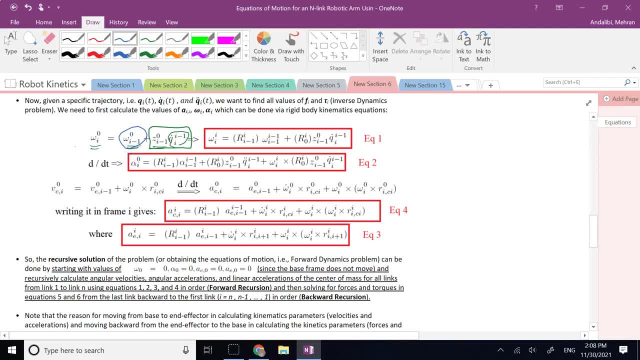 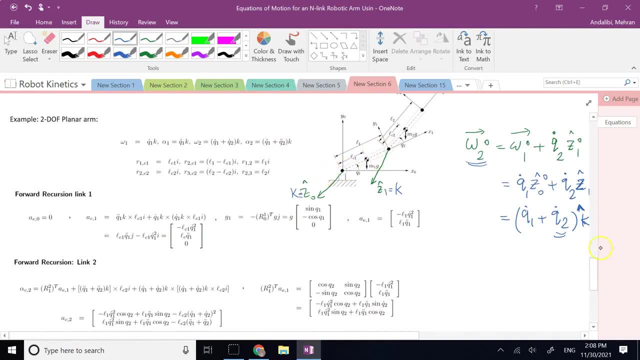 these guys here cannot be easily directly measured right. In this case we were lucky because the previous link was directly attached to the base. But if I had one more here, let's say I had one extra link here and I wanted to do something. 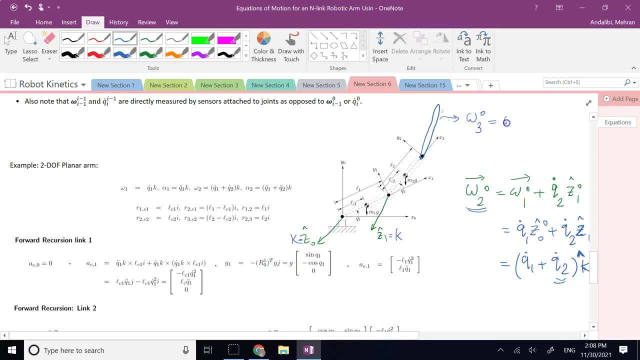 similar thing. say: omega of three with respect to zero is omega of two with respect to zero, plus Q three dot times Z of two in zero. Good, The thing is this: omega of two with respect to zero. I do not have it. 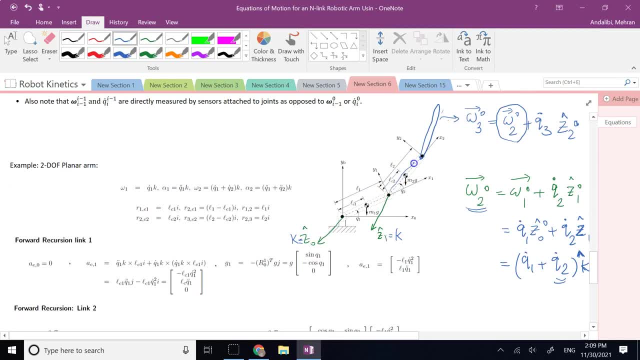 No sensor can directly measure the RPM of link two with respect to the base because link two is mounted on link one, So I can never get omega of two in zero. I can get omega of two in two Really with respect to the body attached frame. 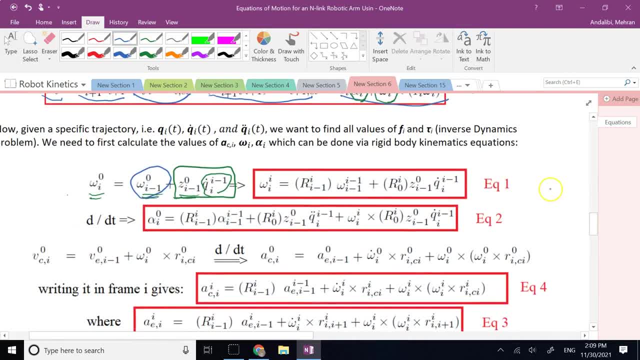 So a better way, better approach. This is I. instead of writing here all of these omega terms in the base frame, I can write all of them in the body attached frame. I you see here everything is in the base frame. 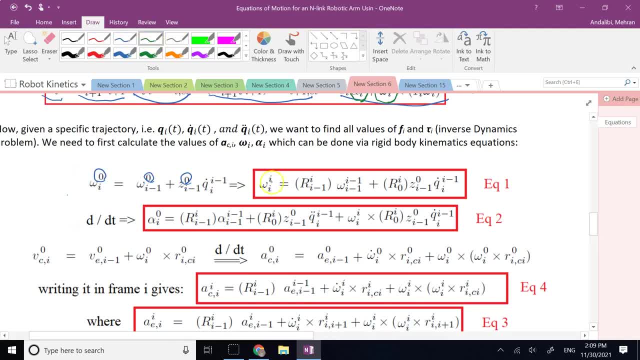 but I can. instead of that, I can write everything in frame. I instead. what's the good thing about it? The good thing is, now I need what I need, Omega of: I minus one in I minus one, not in zero. 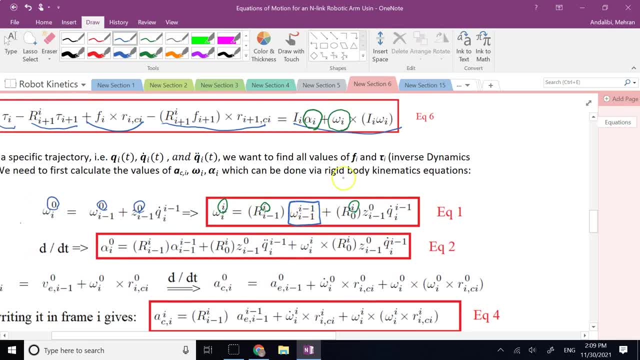 And this is the omega that your tachometer or any other RPM sensor can directly give you. You can read it off the sensor right As well as this one. This is also directly measured in with the tachometers, So these are directly. 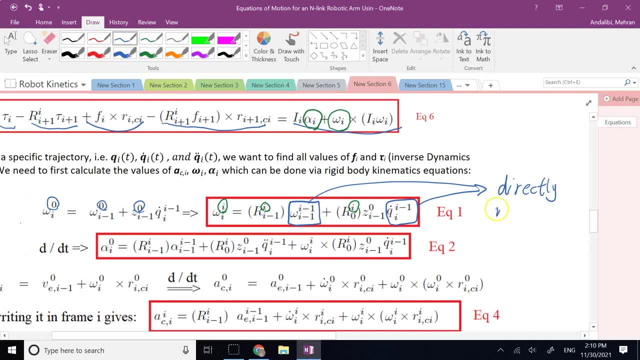 easily measured by RPM sensors Like, as I said, hollow fake sensors or tachometers, While this one you cannot easily measure. So writing everything in frame- I in the body attached frame- can facilitate our calculations and match our calculations to the physical measurements to be matched with physical 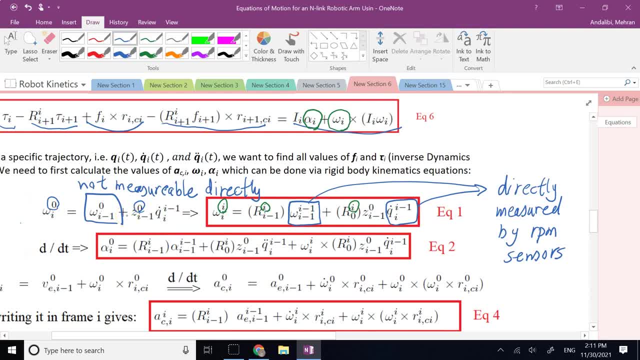 measurements, not to something that you cannot measure. So that's what we do: Instead of using this equation on the left, we use the equation on the right for equation one, that everything is basically projected back into frame I by the help of these two rotation matrices. 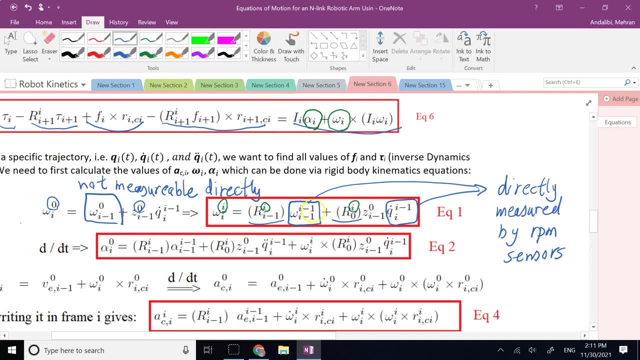 right. So you see, this omega of frame I minus one is now multiplied by R of I minus one in I, So it takes it to frame I and this whole thing here again, which is Q dot of I with respect to zero, multiplied by R of zero, with. 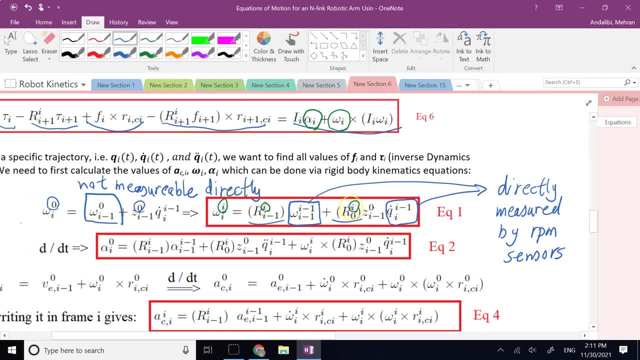 respect to I. And that takes that whole thing again back to frame I. So by the help of these two rotation matrices again, I make everything what Entirely written in the body attached frame. So in order to update my omegas that I need in equation six, 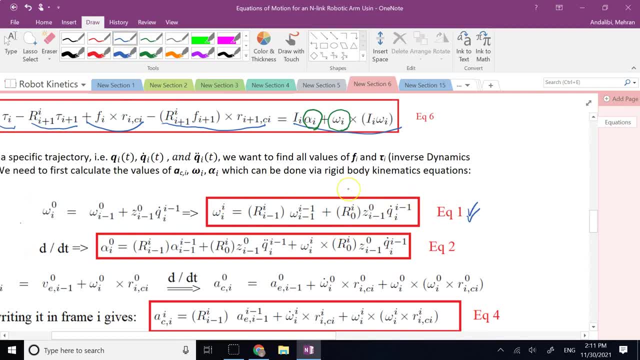 I will use equation number one in this red box right And now we have to talk about how to update. So so far this omega is taken care of by one. How do you update alphas? That's where we look at equation two. 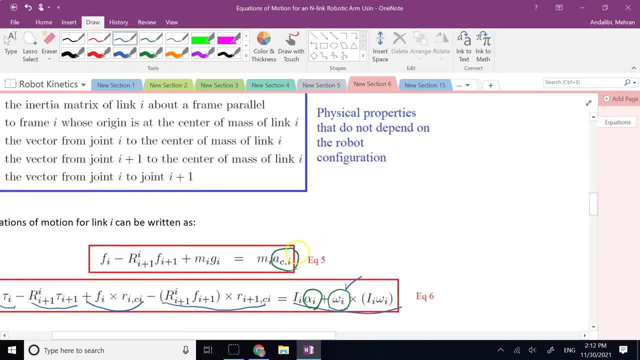 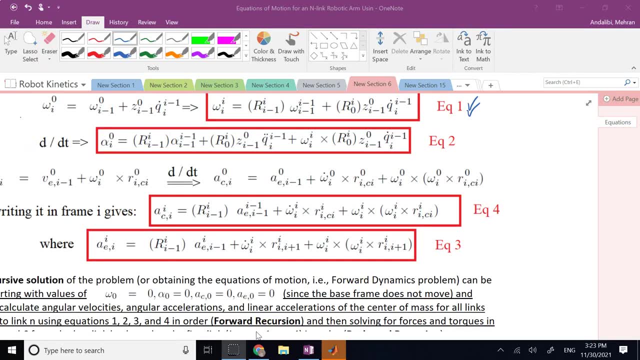 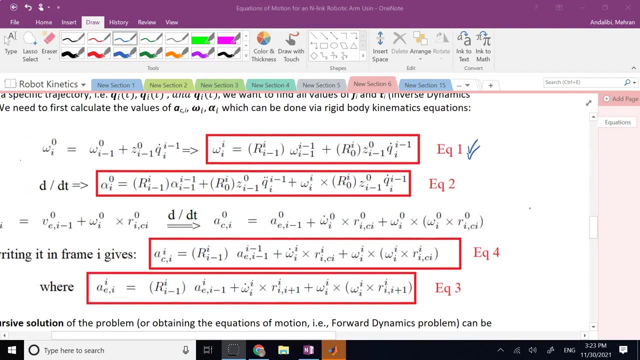 And then how do you find acceleration of the centroid that we need in five? And that's where we go to equation three. So if you look at equation number two, all we have done is taking time. derivative of equation one And you clearly can see that the derivative of omega became alpha. 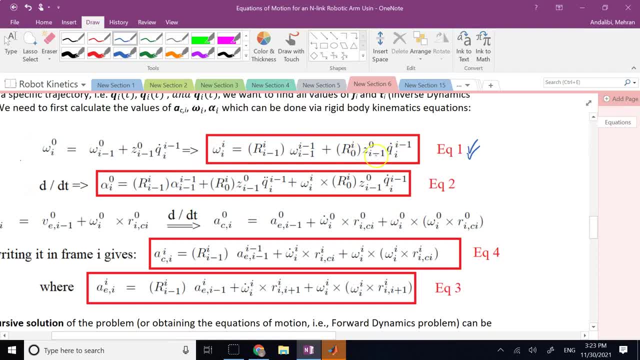 And then this term. here, the second term, it has one derivative, because Q I dot has magnitude change, So it becomes Q I double dot. And the other thing is because this axis, Z I minus one with respect to zero, does change orientation. 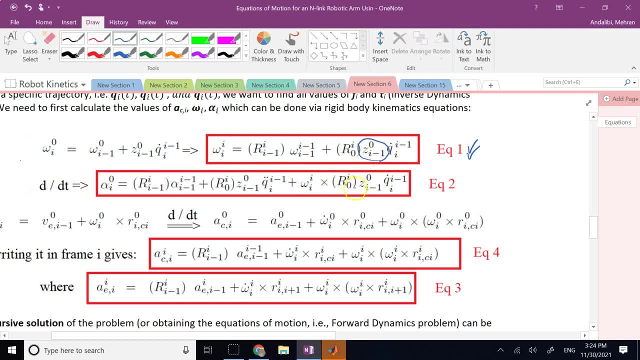 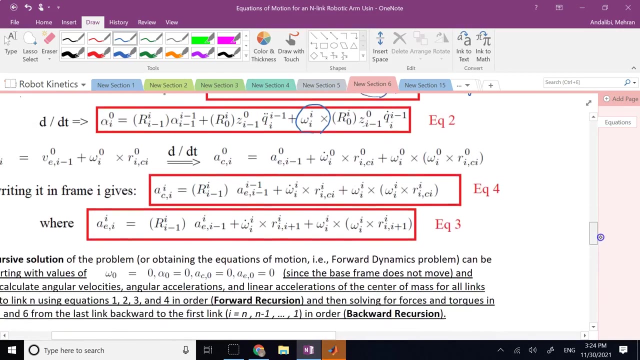 So because of that right, because that axis does change orientation, So the time derivative of that we calculate by omega cross. And here this whole thing is acceleration of frame. I have written in frame zero And this is what we are going to also use in equation number six. 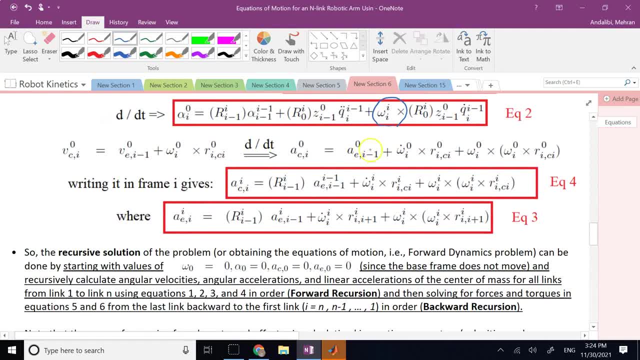 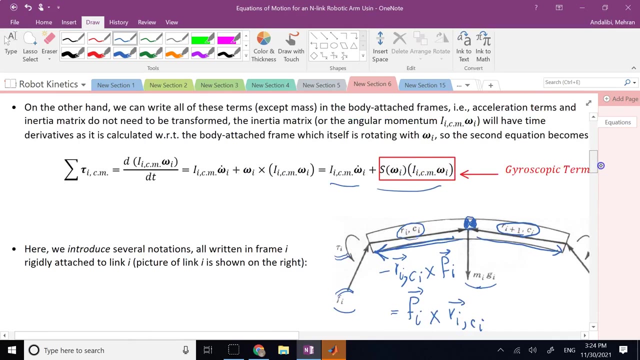 Then we write our acceleration of the centroid equation right. So acceleration of the centroid can be found for link I through the left node or the left joint And then plus the omega cross I right. So here we are using the velocity of this point here. 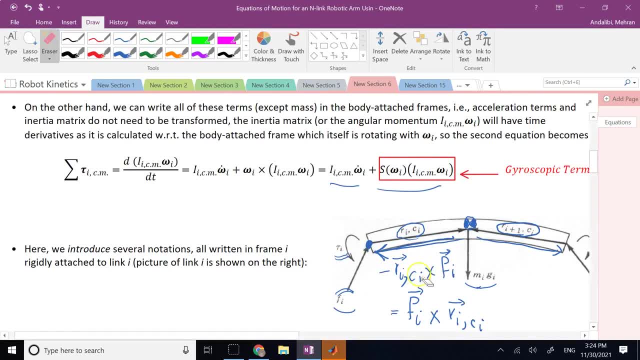 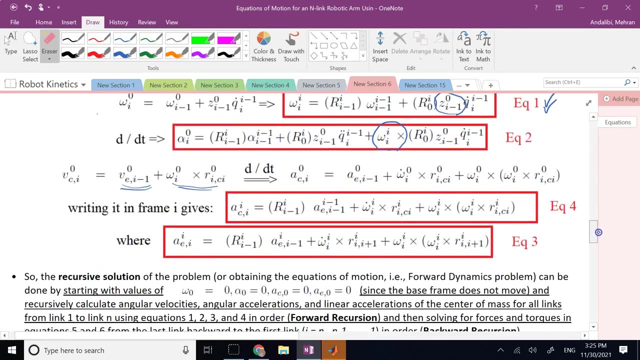 And then add the omega term And that will basically give us the velocity of the centroid And then we can take time derivative from that to get acceleration. And this is what you can see: that the acceleration of the centroid is again acceleration of the left node. 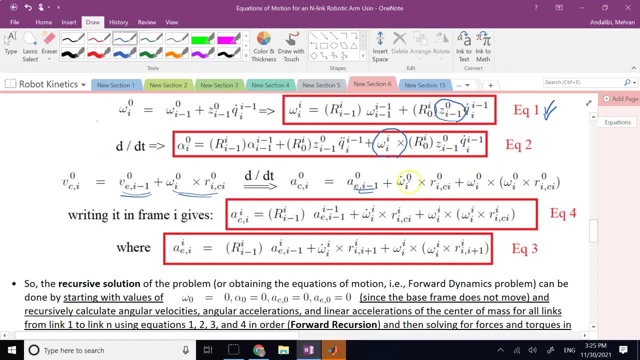 right. So we can write the velocity of the centroid in that picture plus the tangential term, alpha cross I plus the normal or centripetal term, And instead of writing everything in the inertial frame, we can write everything in the body attached frame. 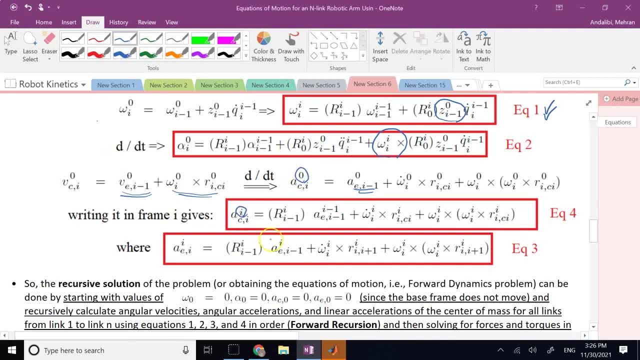 So see, instead of writing it in frame zero I can write it in frame I, And for that I will use again a rotation matrix to do the projections, because this a of the left node can increase the velocity And this node can easily be measured in its own body. attached frame. 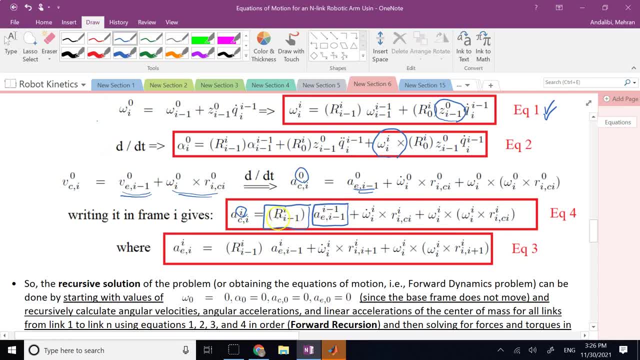 So if you basically multiply by rotation of I minus one to I, it will definitely take it to frame I for you, right The same thing that you have here, And then, for that reason also, you need your omegas and omega dots to also all be written in frame I. 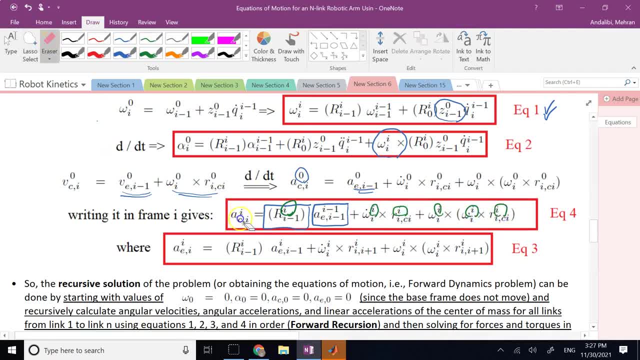 So you can have the acceleration of the centroid calculated, but in frame I body attached frame instead of the centroid, which makes it a lot easier to calculate, right? Because again, if I have a sensor, this term here, this angular acceleration. 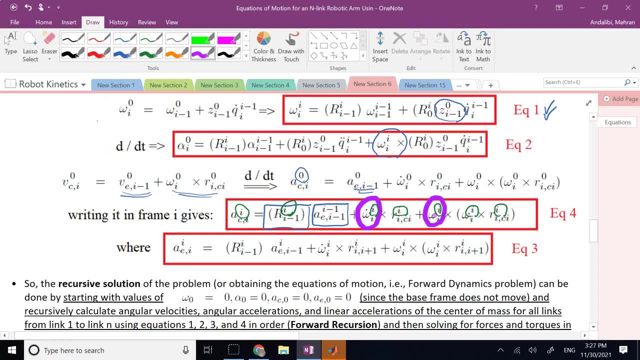 and this term. they are much easier to measure in body attached frame. There is no direct measure of them in the inertial frame. And now you might say: well, okay, fine, I have omega and alpha for this formula from these top relations. 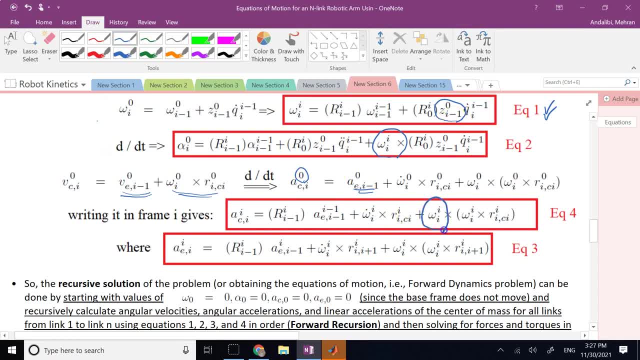 right. So if I wanted omega, I have it, because this omega here and here, that comes from this equation number one, So I have that one covered. The R vectors are typically part of geometry, The omega dots. I can get it from this alpha relation. 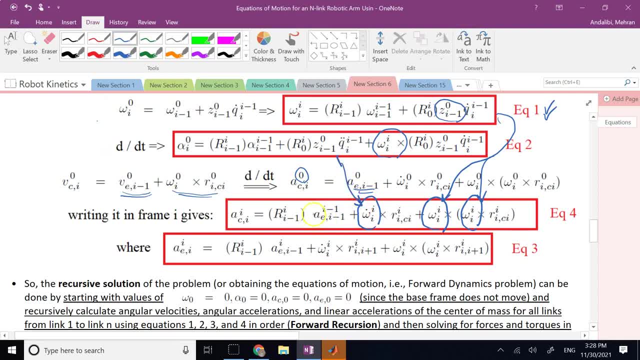 And the only thing remaining is: what is the acceleration of the centroid, The acceleration of the left node or any specific node that I know something about it? Where do I get it? You say, well, you get that from what. You get it from the previous link. 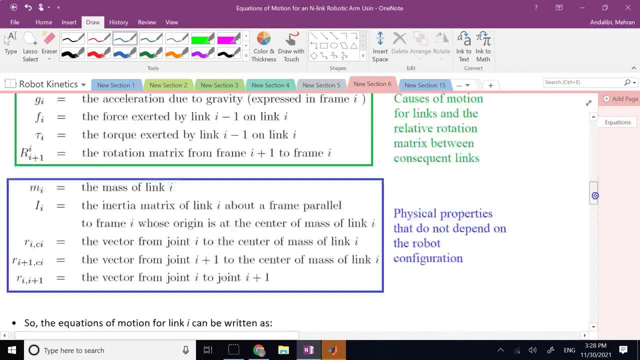 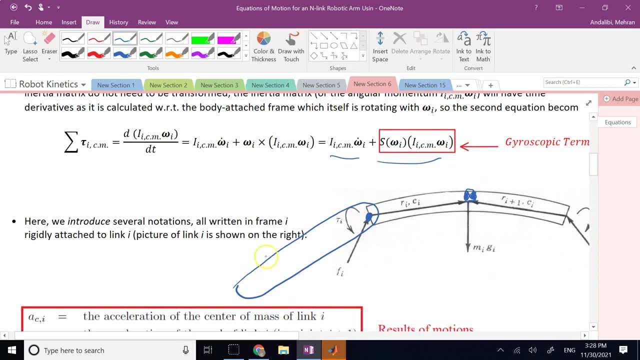 correct, Because this node on the left is the intersection point between link I and then what Link I? minus one, correct. So if I want, I can find the acceleration of this point through the previous point right. The previous point And for the previous point. 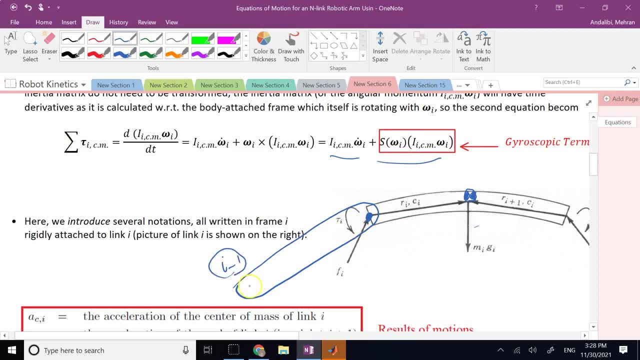 if I know the acceleration of this point. what I need is this vector that goes from: basically it is going to be like R of I minus one. right, It's this vector that we have not used so far. This guy is R of I and I plus one. 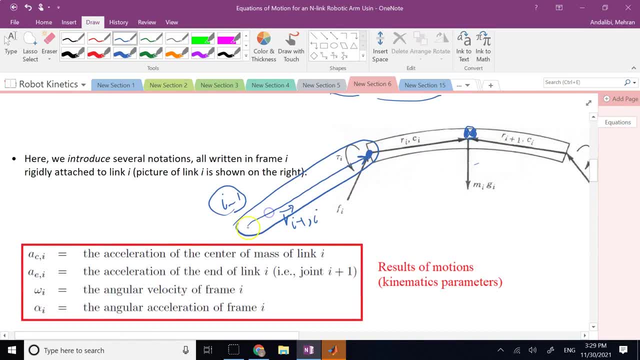 In this case it's going to be R of I minus one and I, If I have acceleration of this point here, the left node on the previous link, and I know this vector which is part of geometry, and I know omega of the previous link and alpha of the previous link. 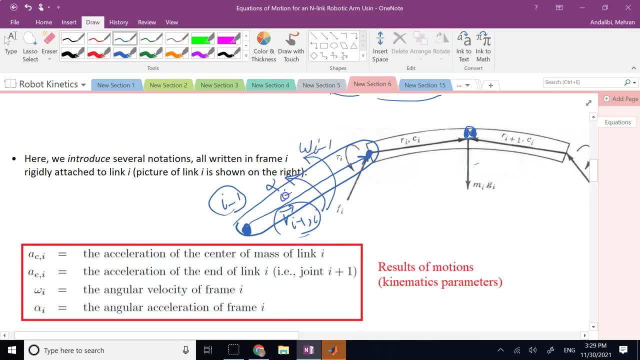 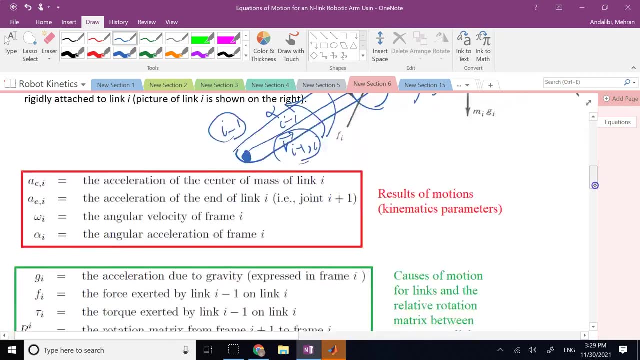 correct, Then I should be able to calculate this point. Once I know that through the info about this guy here, then I can calculate the acceleration of the century correct. So you clearly see, you have to go back and that's what we do. 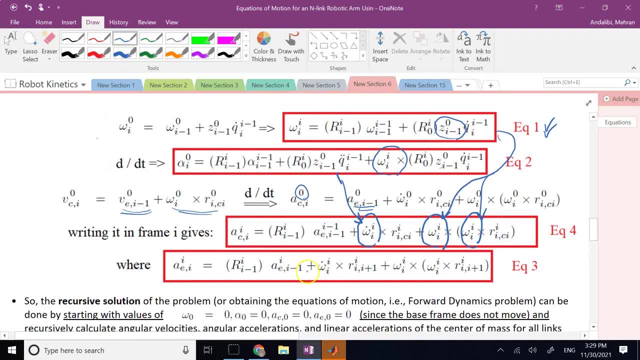 It's called the recursion formulas. So if you look at this, equations one, two, three and four each link. its kinematic entities. omega A's and alphas are related to the previous link, not directly to the base. 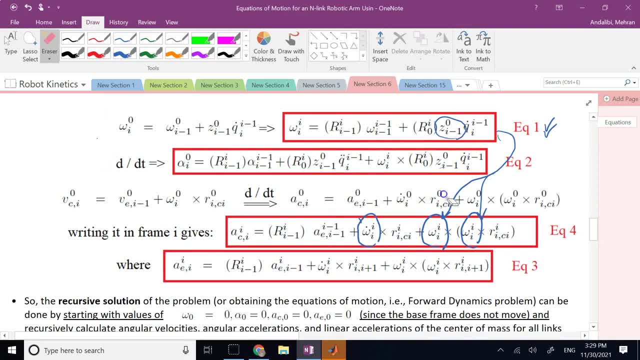 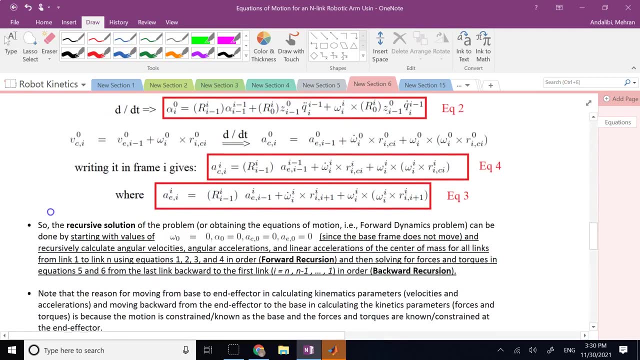 And the result of that is recursions or recursive or update formulas. So all of these equations, one, two, three, four, five, six, seven, eight, nine, 10,, 11,, 12,, 13,, 14,. 15,, 16,, 17,, 18,, 19,, 20,, 21,, 22,, 23,, 24,, 25,, 26,, 27,, 28,, 29,, 30,, 31,. 32,, 33,, 34,, 35,, 36,, 37,, 38,, 39,, 40,, 41,, 42,, 43,, 44,, 45,, 46,, 47,, 48,. 49,, 50,, 51,, 52,, 53,, 54,, 55,, 56,, 57,, 58,, 59,, 60,, 61,, 62,, 63,, 64,, 65,. 67,, 68,, 69,, 70,, 71,, 72,, 73,, 74,, 75,, 76,, 77,, 78,, 79,, 80,, 71,, 72,, 73,. 74,, 75,, 76,, 77,, 78,, 78,, 79,, 79,, 80,, 80,, 80,, 80,, 71,, 82,, 82,, 83,, 84,. 82,, 83,, 82,, 92,, 83,, 84,, 83,, 84,, 83,, 84,, 84,, 85,, 85,, 87,, 87,, 88,, 89,. 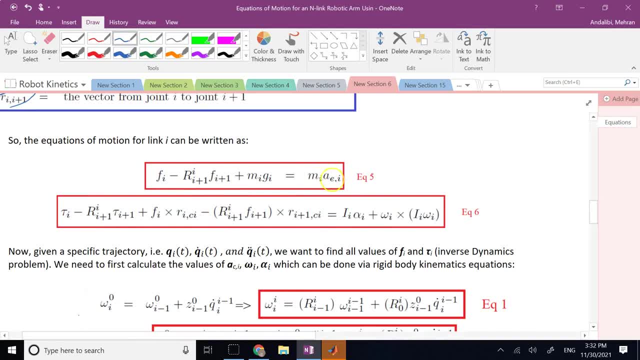 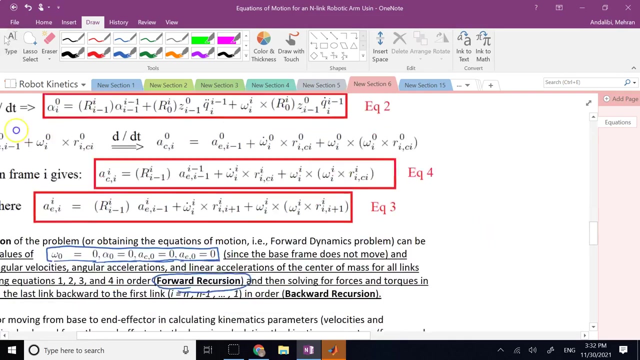 99,, 100,, 100, 100,. as I said, I have these entities that I need. in order to find the F's and the Tau's, I need to go from the end effector back to the base frame because, again, if I go back to this example of this robot, it's at the end effector that I know. 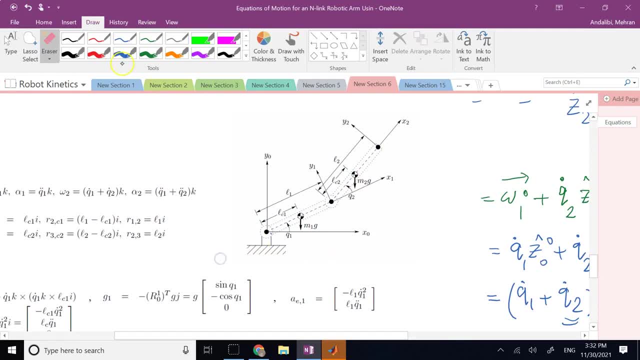 anything about the forces or the torques right. so for example, if the end effector is free, it doesn't come into contact with anything. then I know at this frame here, F number n is equal to zero and also Tau number n is equal to zero because there is no couple or there is no force applied to the end effector. 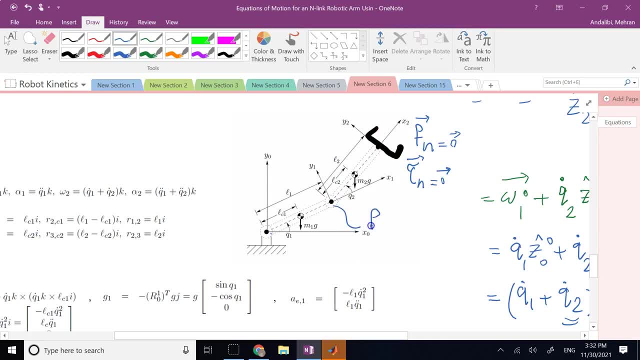 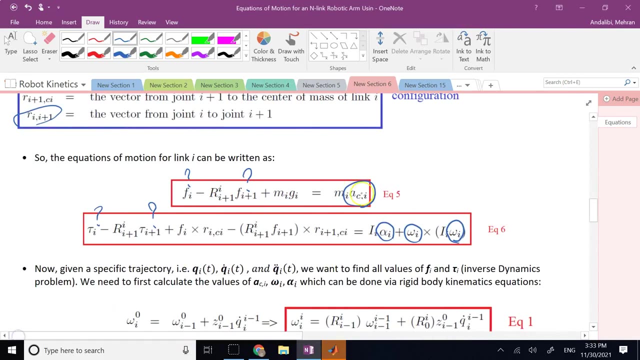 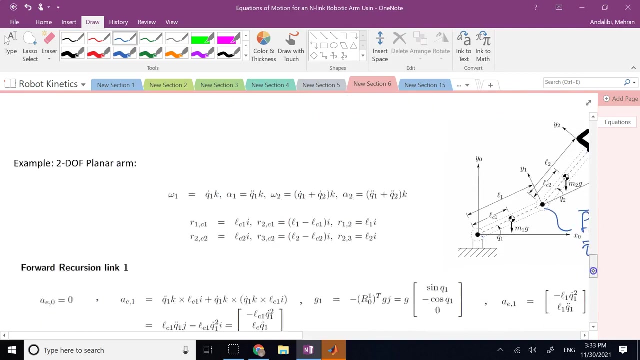 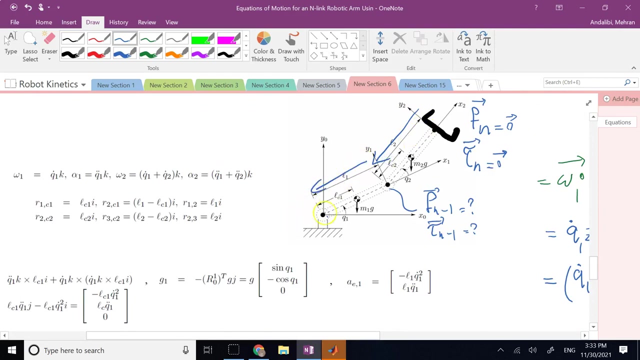 once I know that, then I should come here and calculate F n minus 1 and Tau n minus 1 by going through equations, what 5 and 6 right? and once I know the previous frame, I keep going backwards, and backwards, and backwards. so my direction of calculation is from end effector back to the base, and that's why. 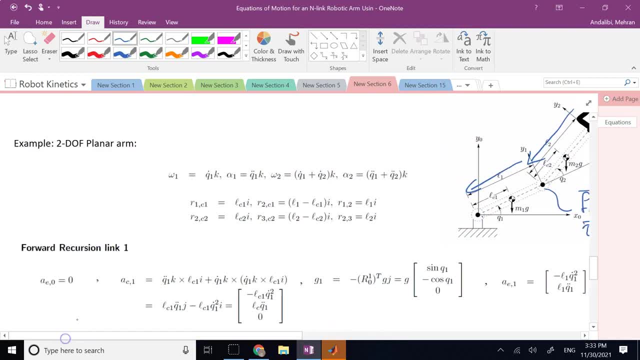 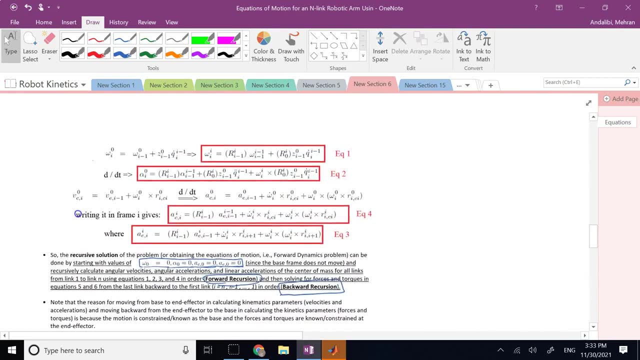 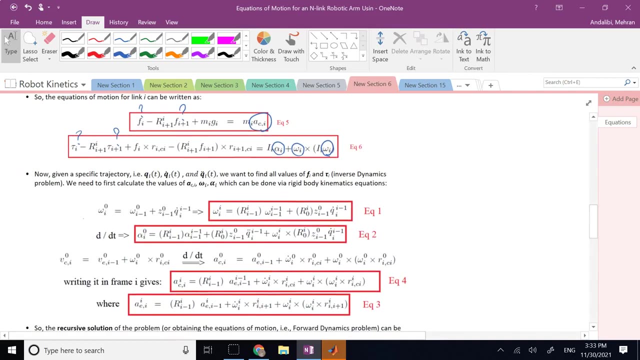 we call these equations 5 and 6. that are kinetic equations. we call them backward recursions and that's what you can see here. so, in general, solving for equations of motion and the reaction forces and torques in a robot using the Newton Euler equations needs applying. 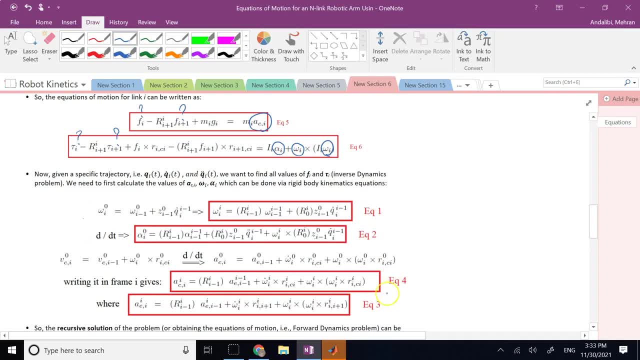 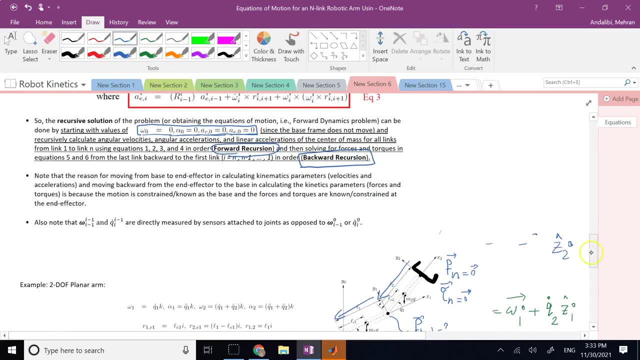 equations 1 to 6. 1 to 4 are called forward recursion, 5 and 6 are called backward recursion and they give you enough equation to solve for any type of problem, whether it's forward kinematics or inverse dynamics. you should be able to solve for anything. 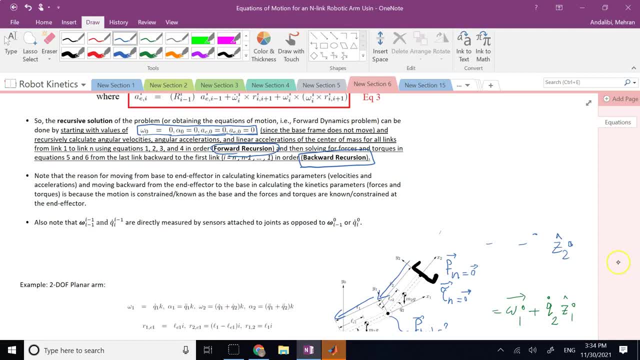 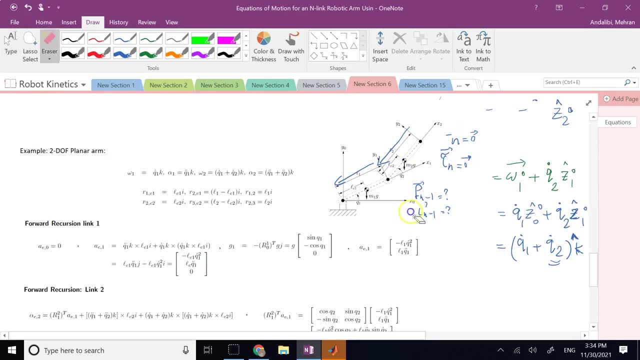 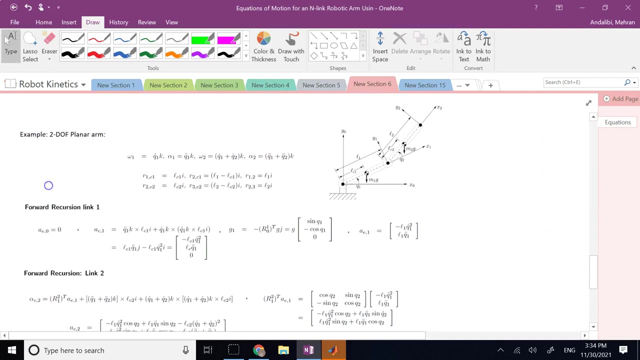 here. now let's go ahead and look at the application of what we just discussed to the two degree of freedom planar arm and see if we can find the equation of motion as we go forward, well as the reactions at the pins for these robots, based on the method we just learned. 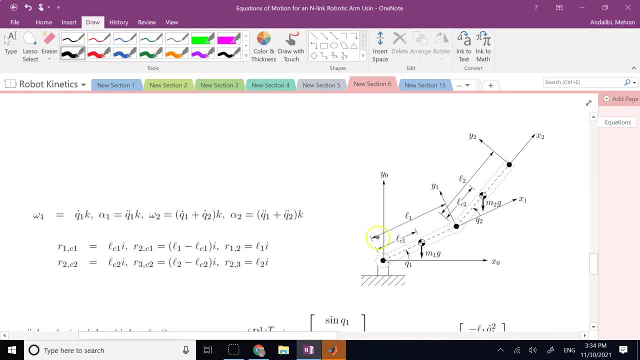 so what we have here? we have two links: l1- l2. the centroids are at distances lc1 and lc2 from the left node. they are not necessarily equal to l1 or l2 over 2, so the bars are not necessarily uniform. the mgs are shown, the angles are shown- q1 and q2. the coordinate frames of denavit hartenberg are: 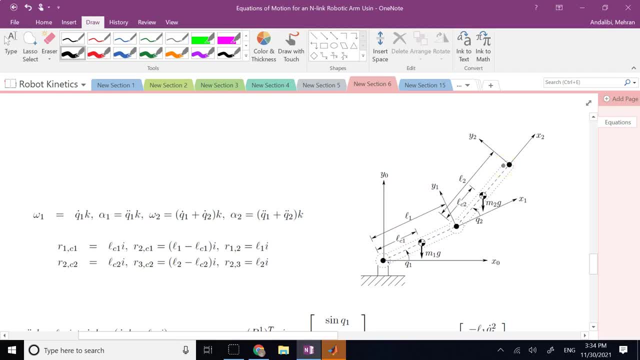 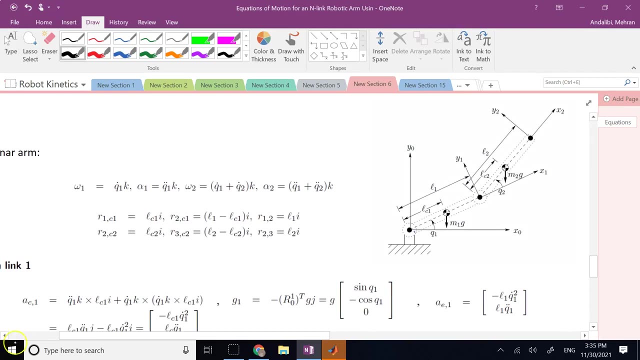 shown: frame 0, frame 1, frame 2.. so now we have to start with the forward recursion, finding omega a's and alphas, and then go to backward recursion and find f's and uh, taus. so here let's do the forward recursion. so we know that omega of zero is zero. so from there we can find omega, one omega. 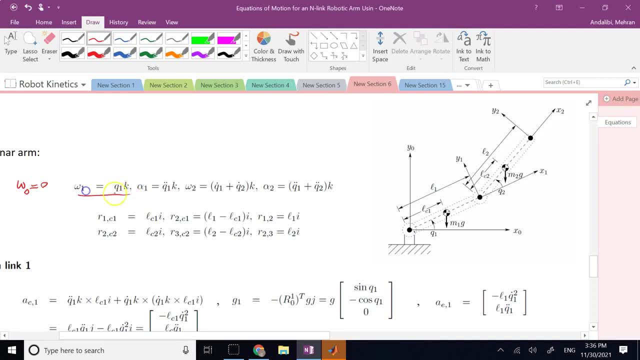 one. if you want to find it, of course, you can easily show that it's q1 dot times k and alpha one is q one double dot times k. omega two is q one dot plus q two dot times k, and alpha two is q one dot plus q two: q one double dot. 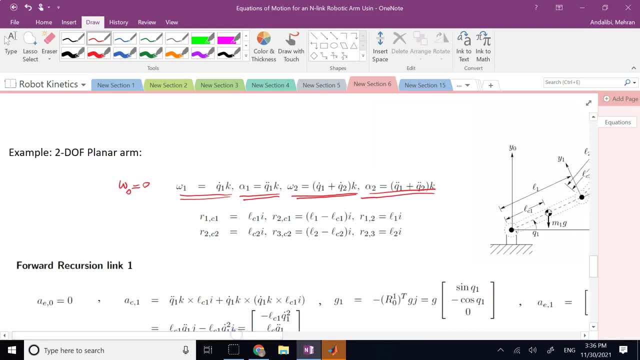 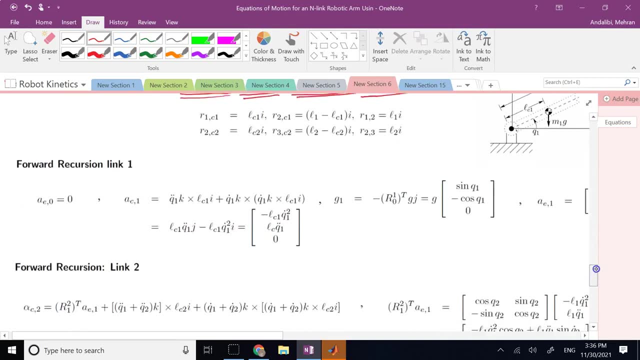 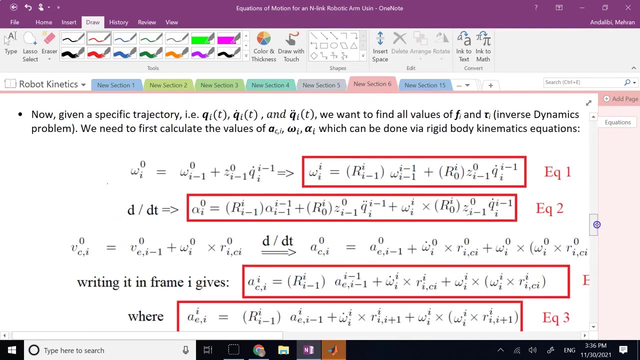 plus q, two double dot times k, and you might say: well, where did you get those? all we need is to apply that equation number one right, which says: omega i or omega i in i is equal to what, it is equal to the rotation of i minus one with respect to i. 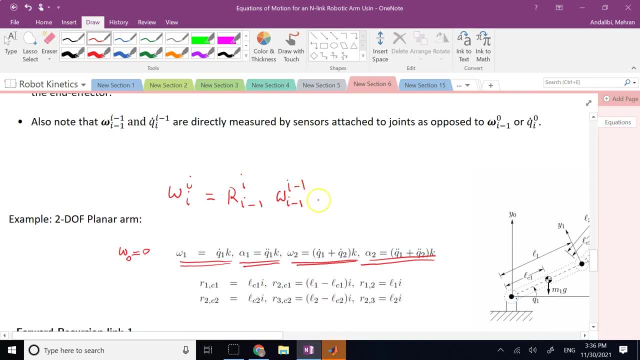 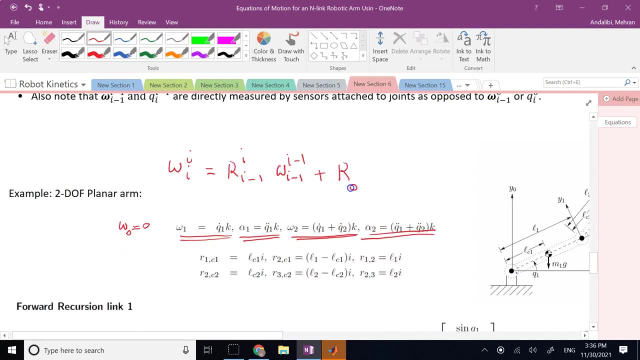 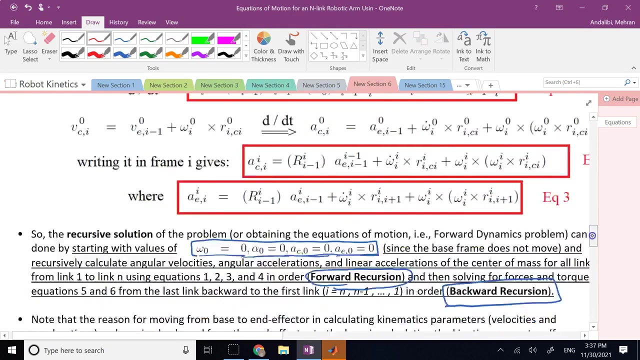 times omega of i minus one, measured in its own, and then plus what you have: rotation of zero in i, unit vector z of i minus one in zero. and then here you have q dot correct, and what you need. this one should be: i minus one in i minus 1, correct, or i in i minus one, actually. 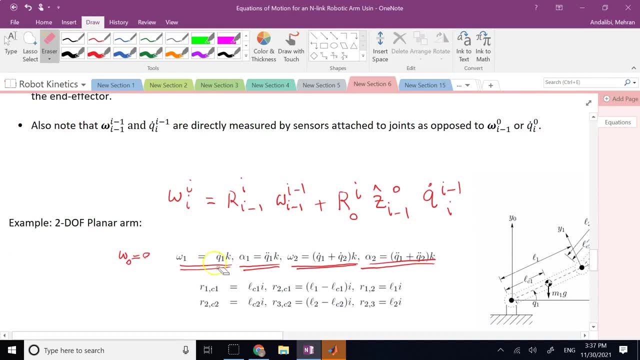 so this is your update equation. now, is that going to give me both omega 1 and omega 2? absolutely so in this case. you know, you have rotation matrices 1 and 2. what are they? well, your rotation matrix 1 with respect to 0. 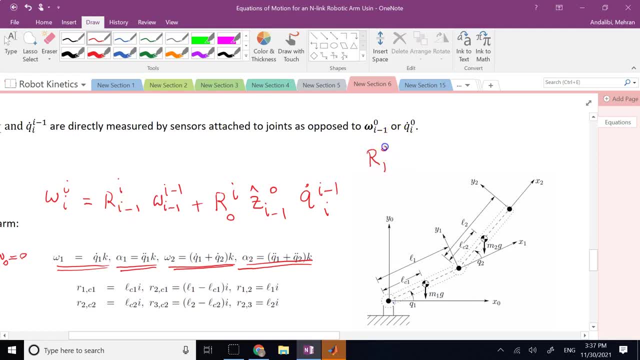 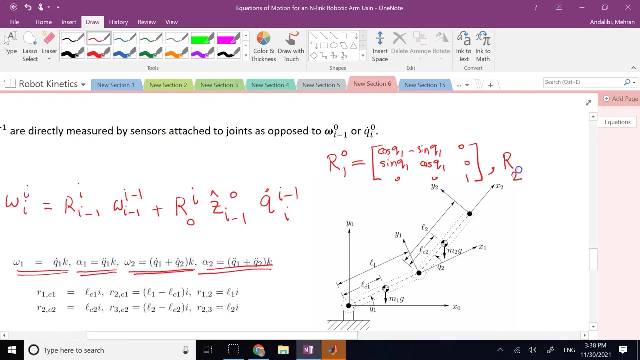 or zero with respect to one, doesn't matter, you can do the transpose of it. so rotation of one with respect to zero is what it is: cosine of q1- negative sine of q1- zero sine of q1. cosine of q1- zero, zero, zero, one. and then, similarly, you have rotation of two with respect to one. 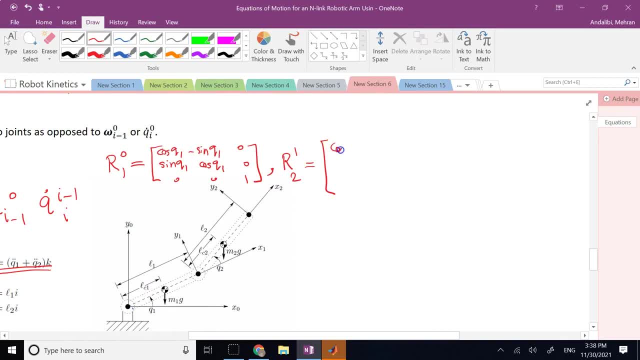 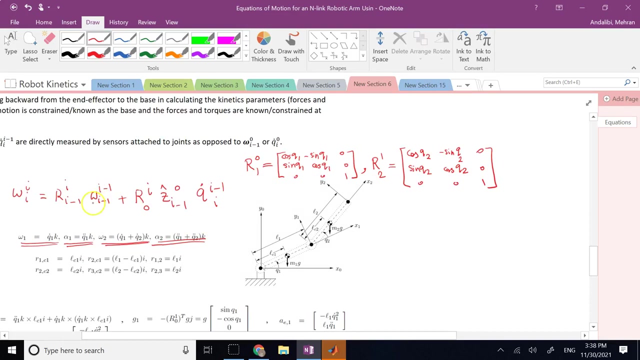 which is very similar, but except this is going to be q2, right? so these are the r's and the b's, right? so these are the r's and the b's that you need. now. what is omega of zero measured in zero? well, of course it's zero, so let's, let's plug in i equal one into that equation. 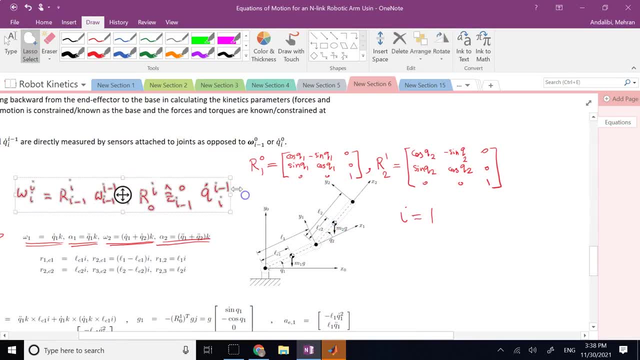 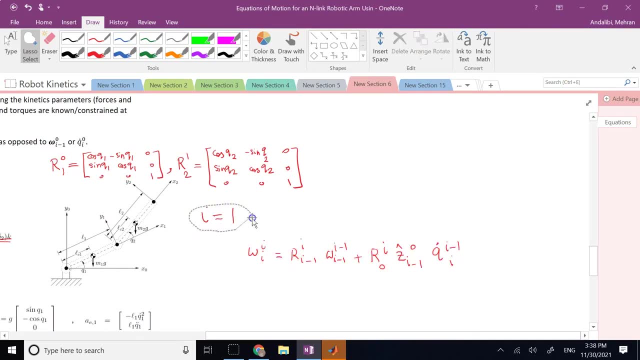 let me bring it to this side. what's going to be the result? well, you know, omega of zero in zero- that's the way to the countersti- of zero in one is equal to r of zero in one. with respect to one of omega zero, and then plus r of zero, one, z of zero, z of zero, zero, and then qenses is equal to r of zero, zero, and then qenses Critical. 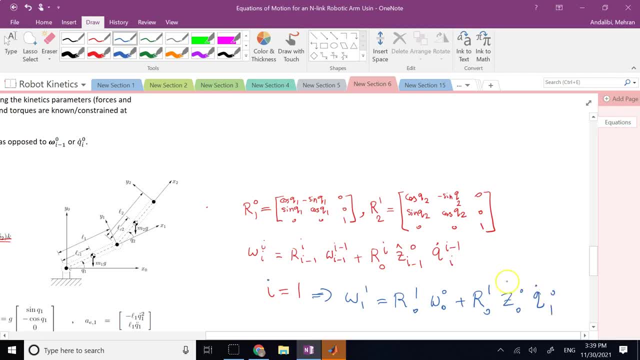 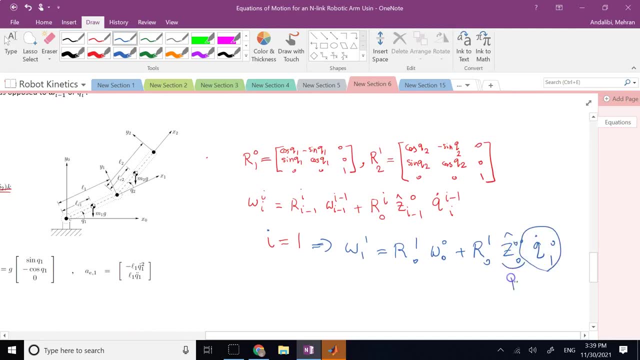 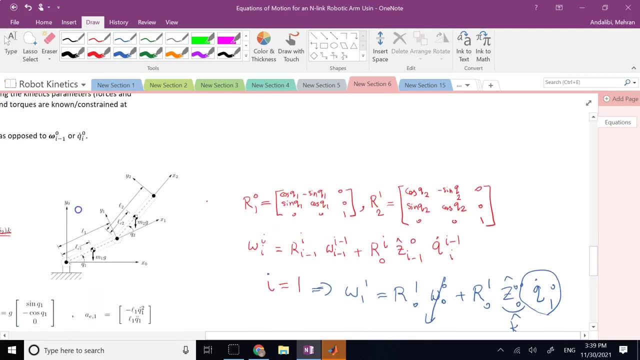 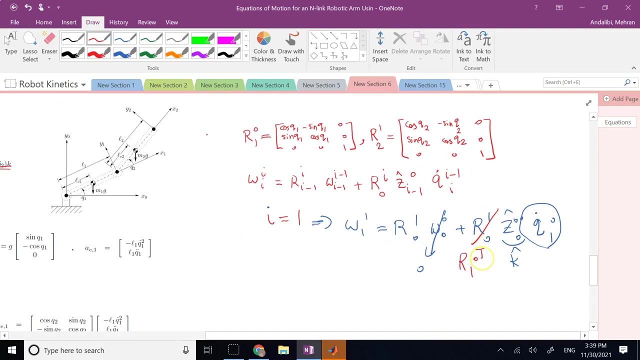 zero, and then qenses, Critical dot of 1,, 0,. right, so this is, of course, Q1 dot. this is your K, this is 0, and R of 0 with respect to 1 is the same as 1 with respect to 0,. just transpose of it, right, so it is. 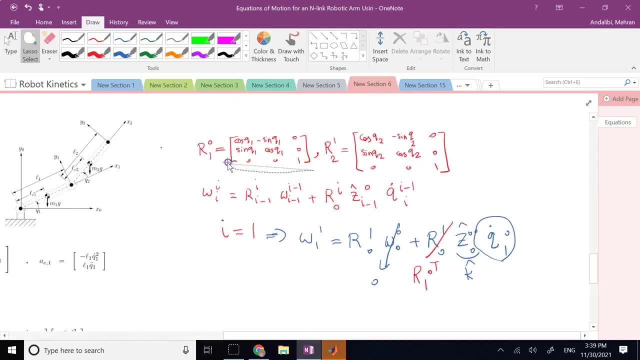 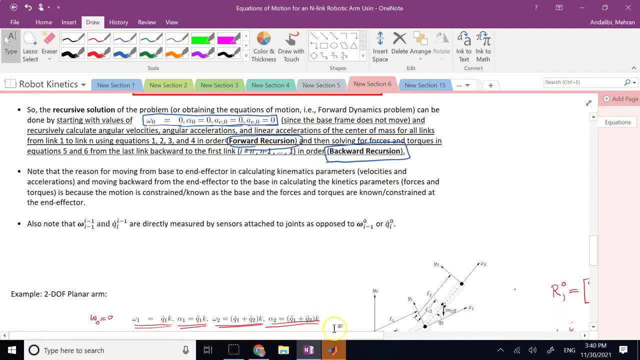 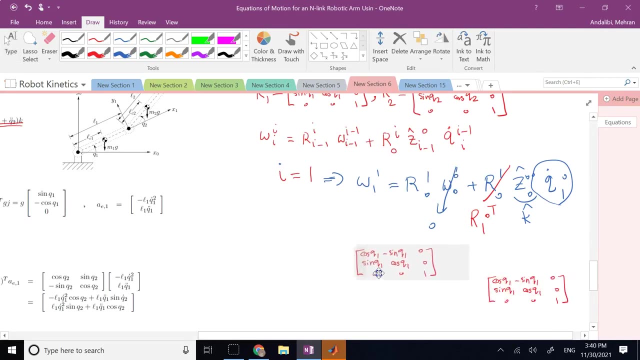 going to be basically this matrix, just the transpose of it, multiplied by K, which is 0,, 0,, 1, and then times Q1 dot. And all I need to do is multiply this matrix by 0,, 0,, 1, and then times Q1 dot. 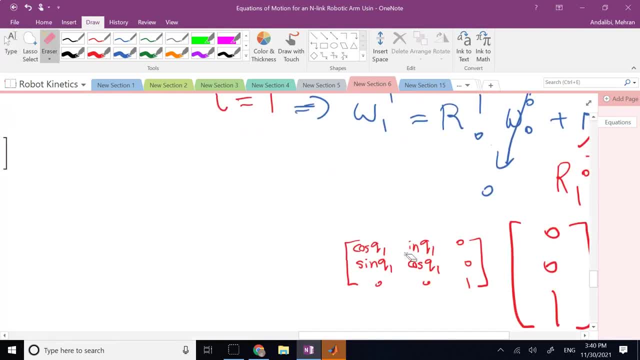 need to change, for this guy is to transpose it. so this is going to be signed. it's going to be negative sign and if I multiply, you clearly will see that the result is going to be what. so this is going to be 0. this is going to. 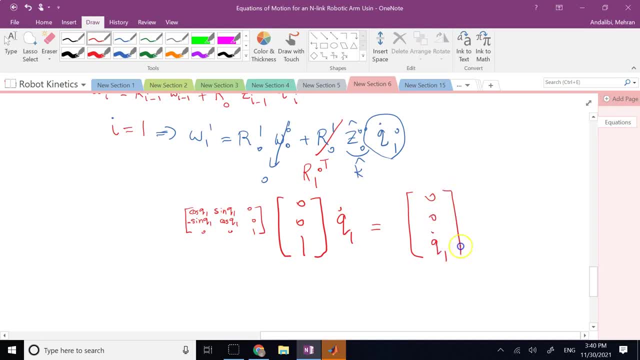 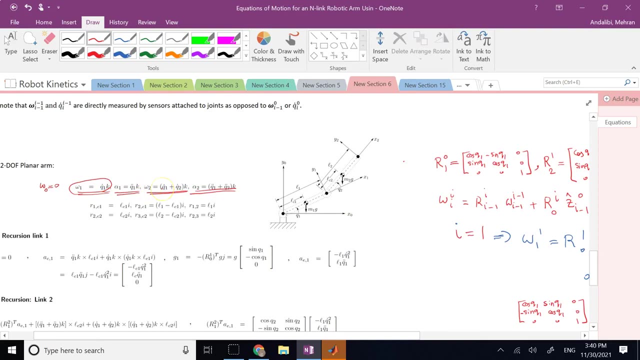 be 0, and the last one is just going to be Q 1 dot, right, so you can also write it as Q 1 dot times K, and that's exactly what I have over here: Q 1 dot K. and then you can do the similar thing: apply Omega 2, and then for Omega 2 you will get the 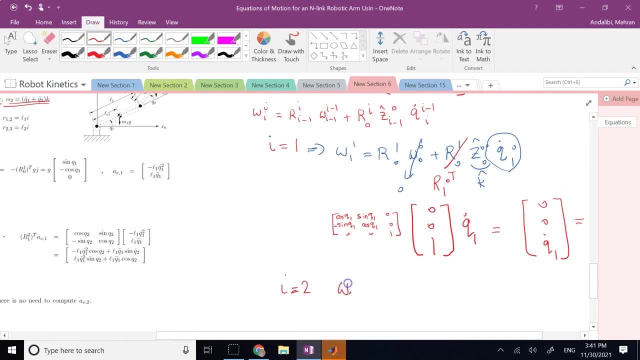 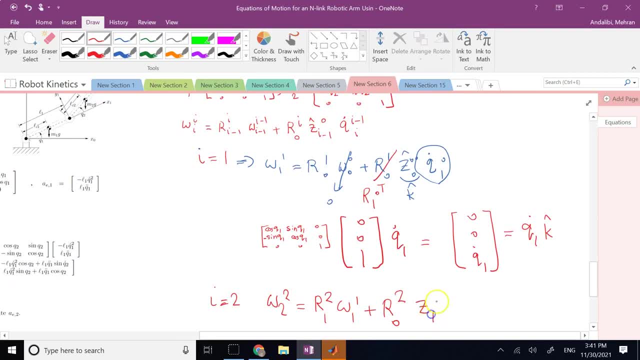 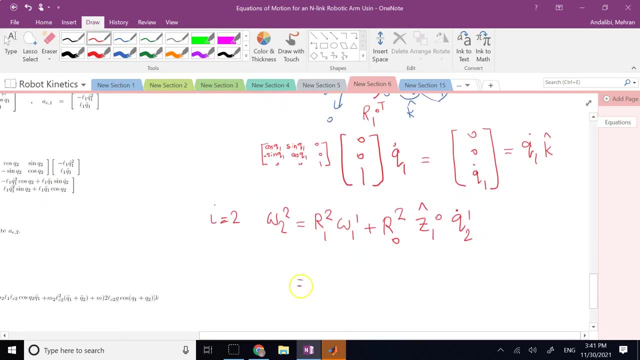 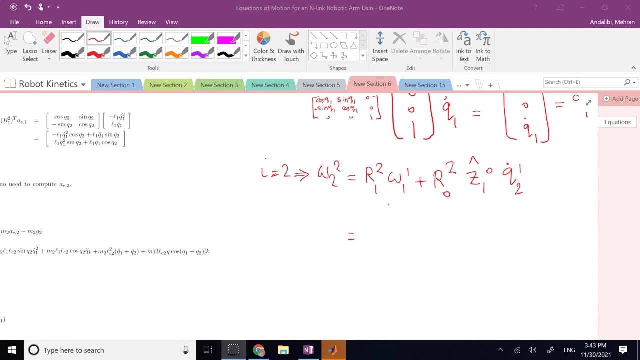 then Z of 1 in 0 and then Q dot of 2 in 1. right, so what do we get in here? so this is R of 2 with respect to 1, transpose of that which we already had above. so this is going to be basically cosine of Q 2, sine of Q 2. 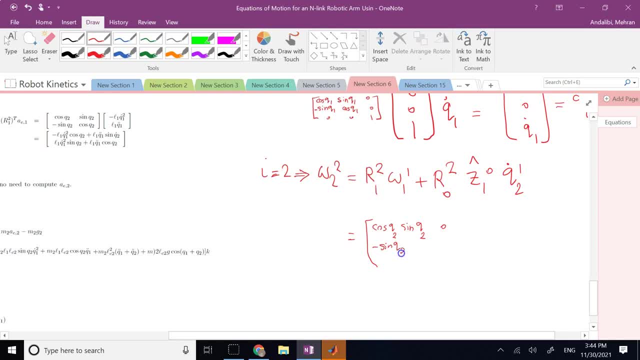 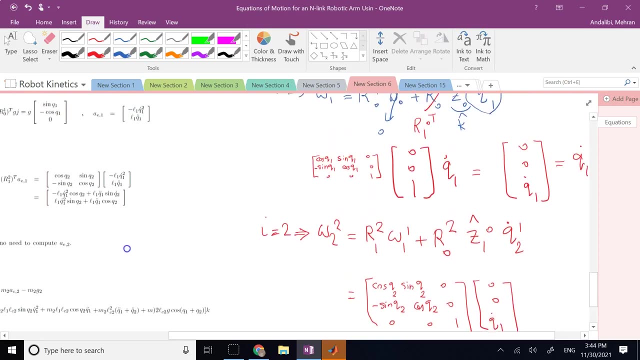 is going to be negative. sine of q to cosine of Q. 2, 0, 0, 0, 1 is to transpose of that Omega 1 was 0, 0 q0. Wordät it already from the previous case capes and that's the recursion rights for. 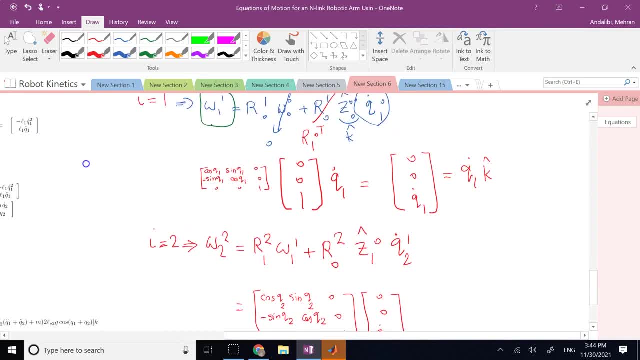 Omega 2. I had to. I have to use Omega 1. so here this is the forward recursion going from 1- quiet in breath, into n and now문 Q 2, 0. Cosine of Q 2, r0, 0, 0, 1 is the transpose of that. Omega 2 was 0, 0, Now 0, Q 1 dot. we had it already from the first case, correct, and that's the recursion right. for Omega 2, I had to use Omega 1. so here this is the forward recursion going from one. 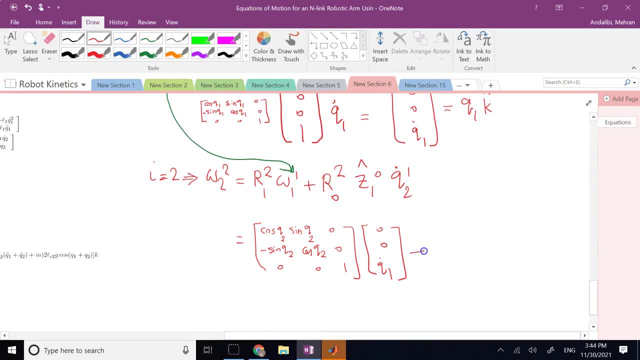 to the next, and r of zero in two. this one is equal to r of basically, um, this is two, this is one, this is one, this is zero. so it's going to be the transpose of each and every one of those two, and uh or two with respect to zero transpose. so it is going to basically be like cosine. 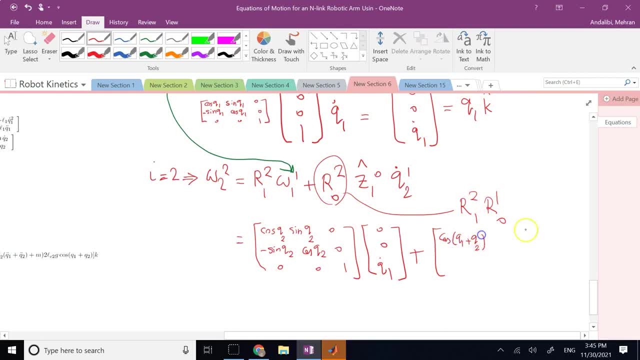 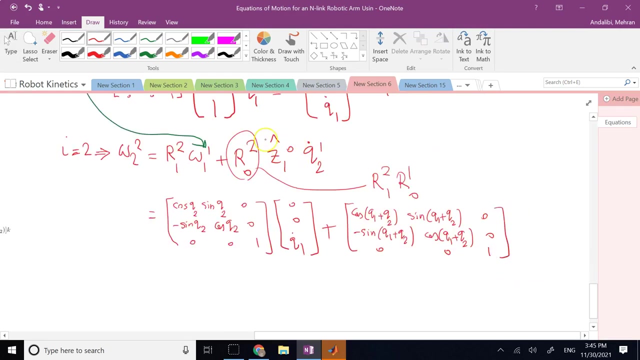 of q1 plus q2. sine of q1 plus q2: zero. negative sine of q1 plus q2. cosine of q1 plus q2: zero, zero, zero one. multiplied by z. one in zero, z one in zero, in this case, it is equal to zero zero one. and then q2 with respect to one dot, which is simply the magnitude of q2 dot, because 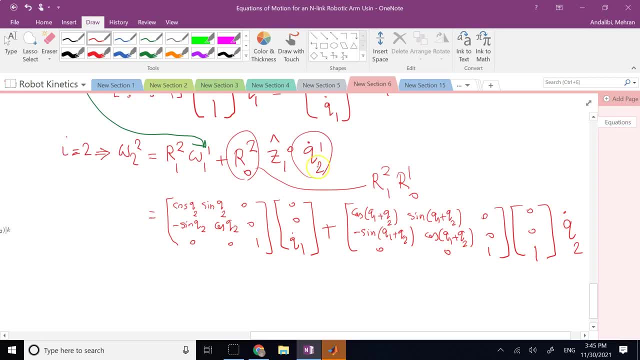 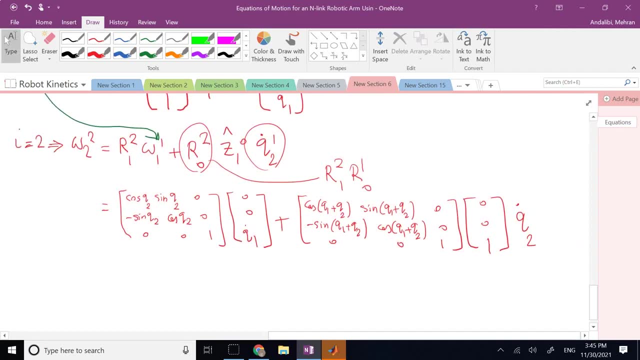 q2 dot is the angular velocity that frame two has in frame one. so that's also we define as q2 dot. now note that in general in this case it was easy for me to say that unit vector z1 is just zero, zero one in general. how do i get the z's? 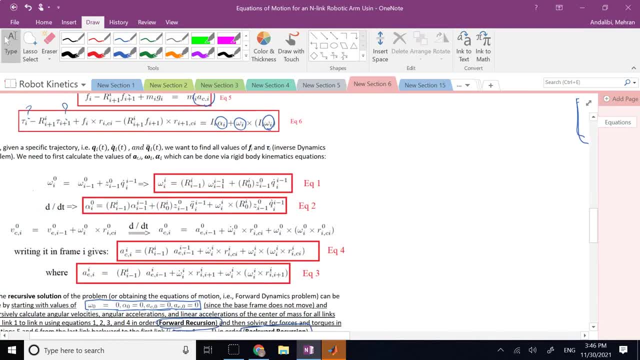 because this z, you see it in the formula for omega, right, you also see it in formula for alpha. the question is: how do i get the z's? and if you remember, we can get them from dh. so if i go back to the dh forward kinematics, for each uh frame i have a t matrix, t of i in zero. 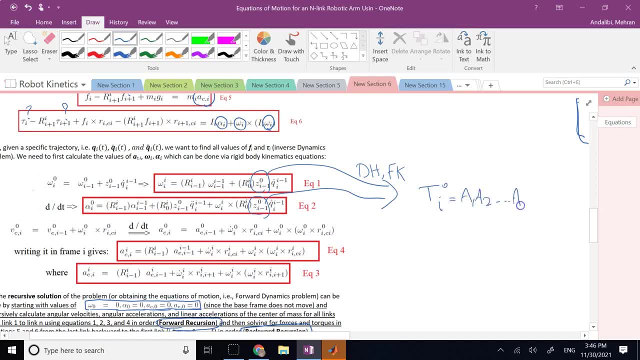 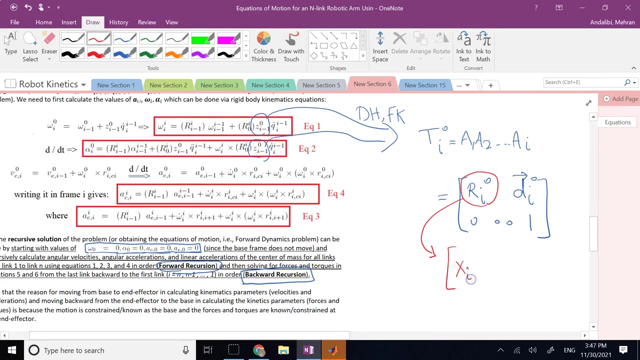 which is like a1 times a2, all the way to ai and, if you remember, this is like r of i in zero, d of i in zero, then zero, zero, zero, one, and then this, this r of i with respect to zero. it has three columns. the first one is x of i in respect to zero, the whole unit, vector y of i in frame zero and z of 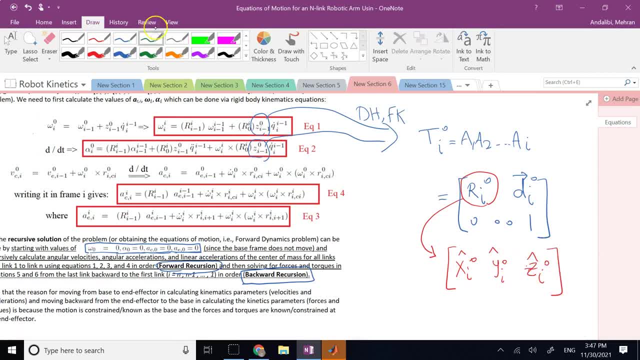 i in frame zero, so i can definitely get it from the third column of the t matrices that i have in forward kinematics using the etch method. okay, so definitely, in order for you to be able to do any of this forward or backward recursions, you initially have to: 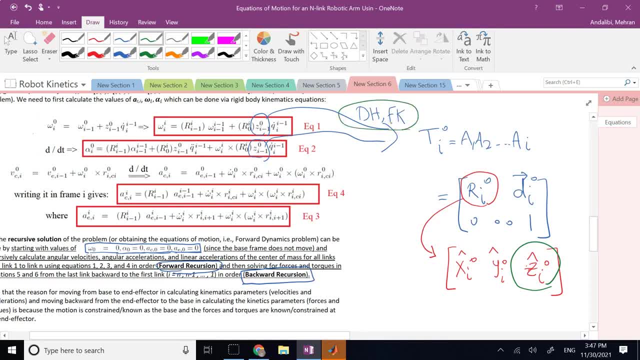 find the dh axis, the dh parameters, the a matrices, the t matrices, so you can get the r matrices that you need all the time. you see, lots of the times, you need tons of these r matrices, so all of them can come from what? from your? uh, denavid hartenberg. so you definitely always 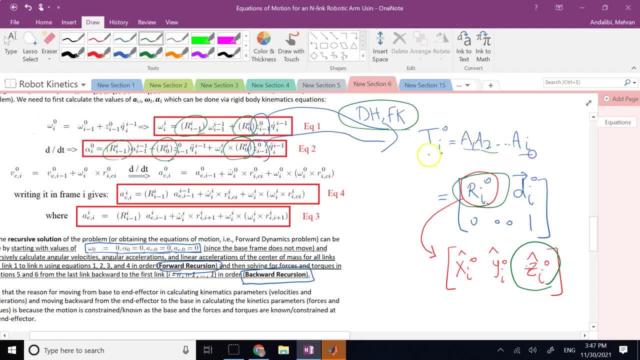 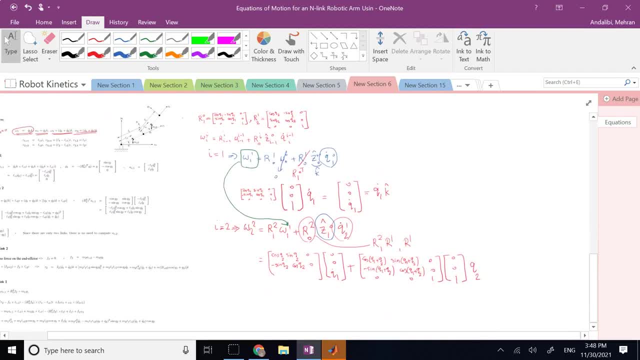 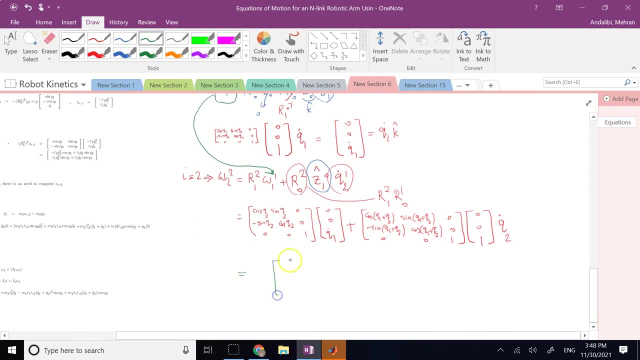 need to perform some forward kinematics and determine all of these a's and all of the t's. good, if you forgot, please watch my previous videos on Denavit Hartenberg, forward kinematics. So now, if I perform this, what's going to happen? This first one is definitely going to be again. 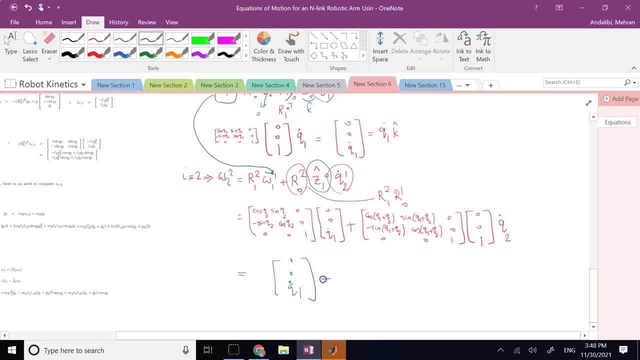 00Q1 dot and then plus. what If I multiply this whole thing? it is simply going to be 00Q2 dot. So I can write it as Q1 dot plus Q2 dot times K and again that's. 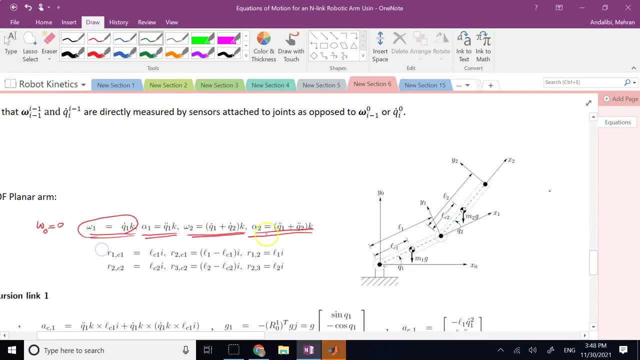 exactly what you can see over here. Okay, so clearly, you see, if I write it properly, I can get it and you might say: well, in this case it's kind of obvious that omega 1 is Q1 dot K and omega 2 is Q1 dot plus Q2 dot K. That's right, because the robot is too. 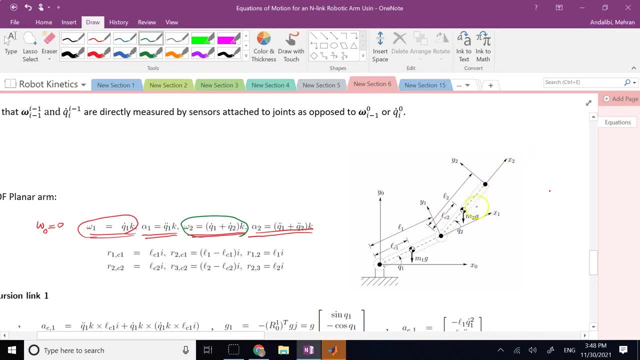 simple. If the robot is really complicated, it's not so easy to do all of those computations visually. If everything is not planar, if you have a combination of revolute and prismatic joints all together, then none of these computations is as trivial. 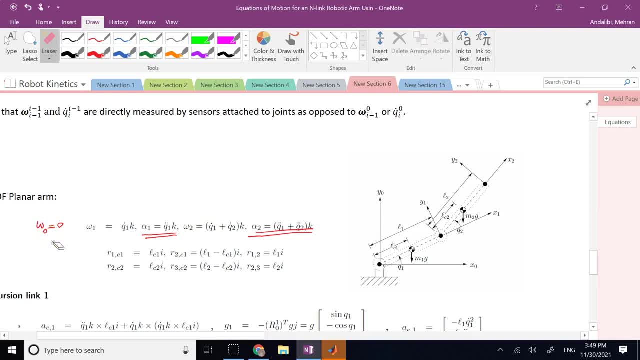 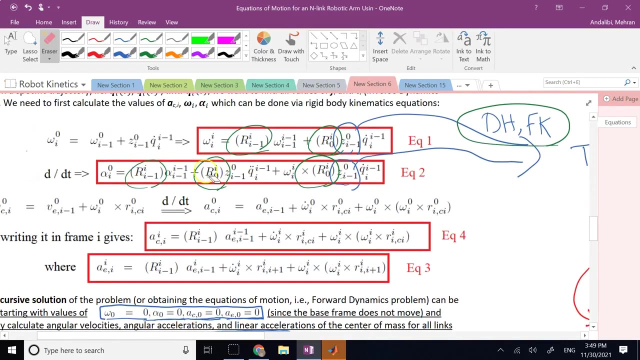 Okay. so you have to go through those recursions and get yourself all of the accurate calculations. Similarly, I can go with the alphas right. Alpha 1 is kind of obvious that it is Q1, double dot times K. Okay, because if you just do this, this one right. 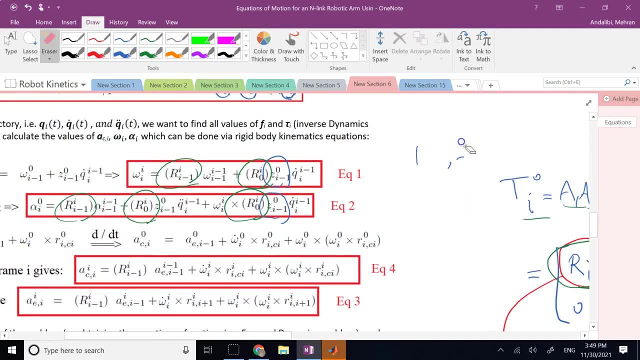 If I just apply this, let me just show you for one of the I's at least Right. So for this formula, if I apply, I equal 1, what do I get? I get alpha 1 is equal to what R of 0. 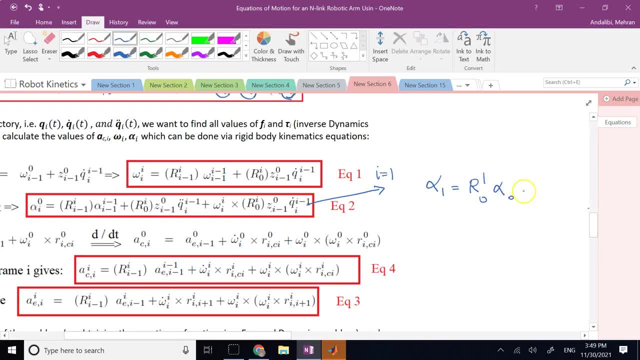 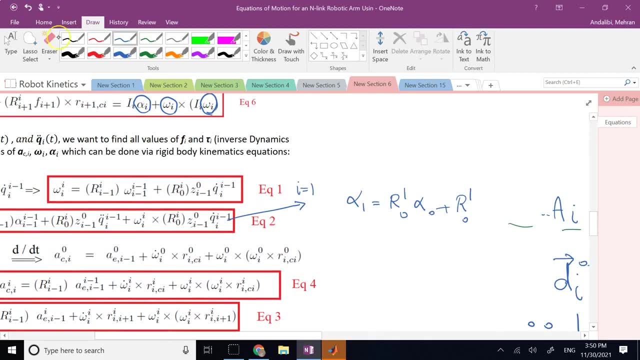 in 1, alpha of 0, and then plus R of 0,, 1 Z of 0, 0, correct, And then Q1 double dot in 0, and then plus R of 0 in 1, Z of 0 in 0,. 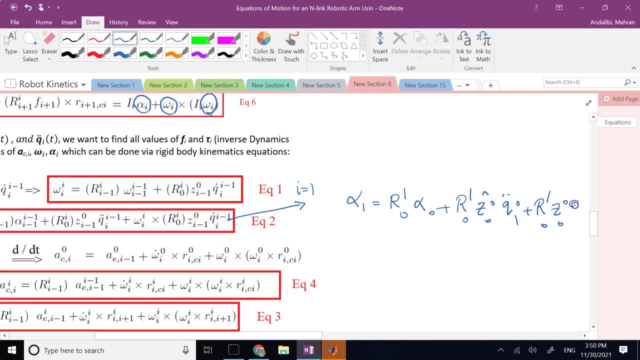 and then Q1 dot in 0, and then plus R of 0,, and then plus R of 0,, and then zero. So you know, alpha of zero is the angular acceleration of frame. zero base. So this is zero. So this is gone. What is? 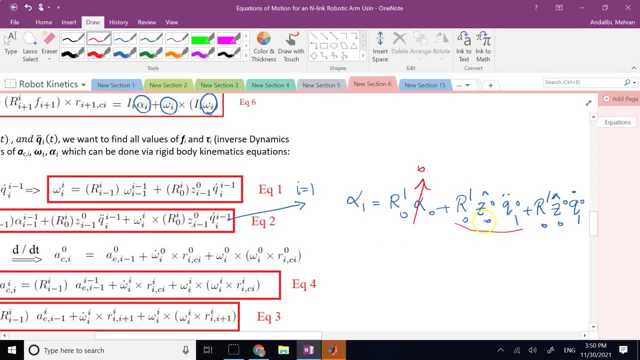 this guy going to be. This is R of zero and one, Z, zero and zero, which is simply zero, zero, one, And we just multiply. you know, when you multiply that rotation matrix, write it. you multiply this by zero, zero, one, q, one, double dots, or you can. 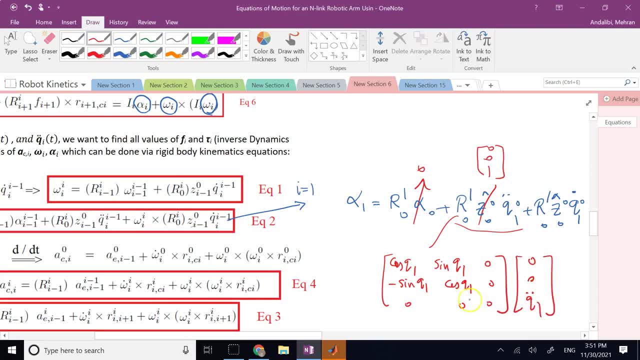 just combine them into something like this: The result of that, this is one. The result of that is simply zero, zero, q, one double dots. So basically, this rotation matrix has no effect on it. And what about this one? Well, we just forgot. 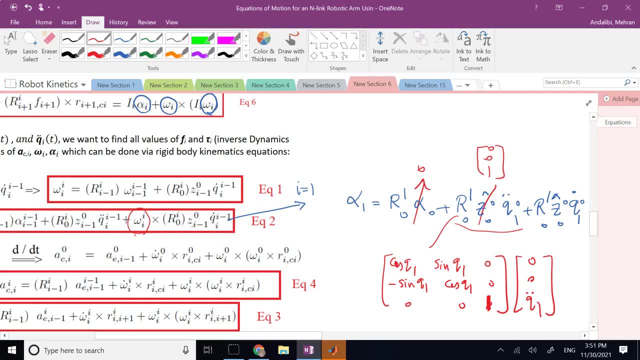 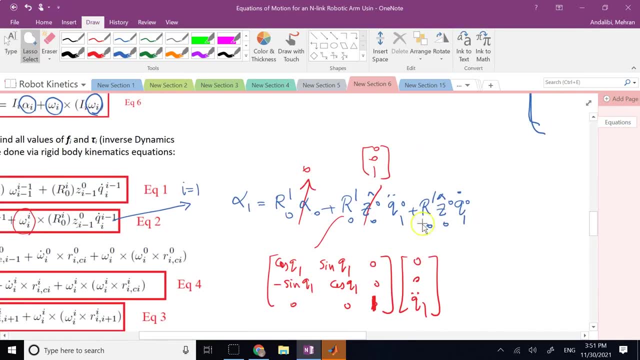 one thing, and we forgot this omega to be added here. So this is going to be like this. Let me get this shifted a little bit this way: So this is going to be plus omega of one in one cross that. So what's happening here? Omega of one in one is going to be like zero. 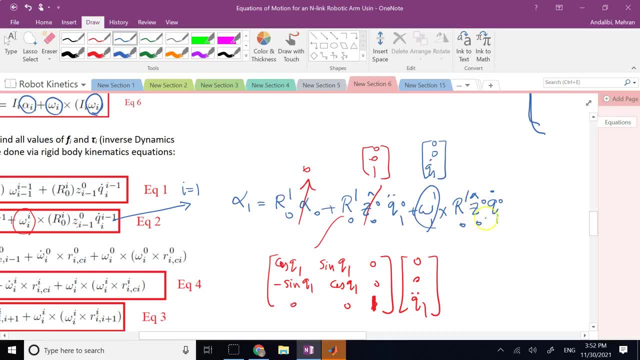 zero q one dots. This thing here also. when you do it it is going to be like zero, zero q one dots. And when you cross product a vector by itself, the result is also zero. So that is zero. this initial one is zero, the only. 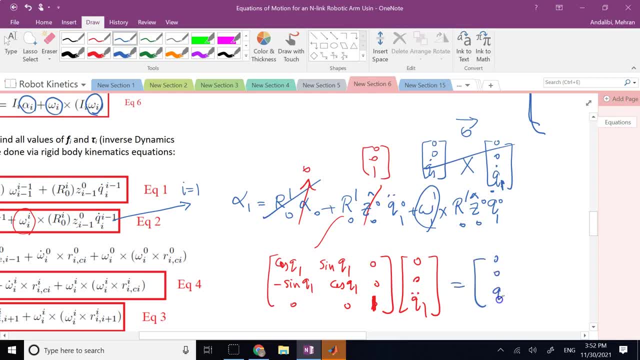 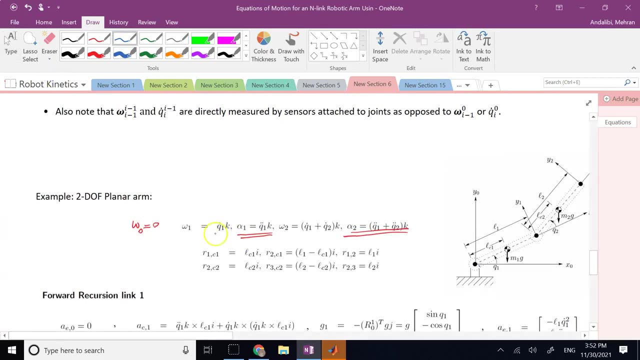 thing that is remaining is zero, zero, q one double dots, which is the middle term, this one, Or you can write it as q one double dot times k, And that's exactly what we have over here. Okay, and then you apply i of two. 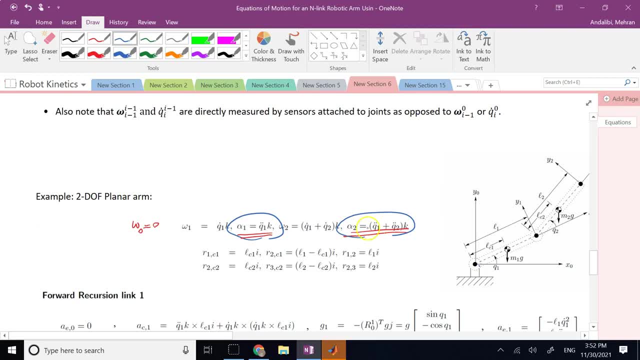 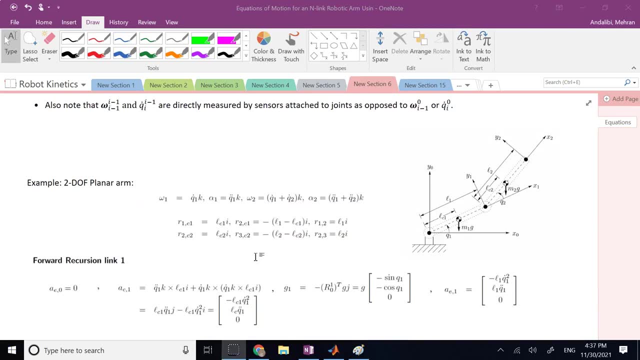 You get this one and you can keep repeating. So definitely, using equations one and two, I can get my omegas and alphas. Okay, so here I have done some cleaning so I can write on the rest of the pictures. So you also need some r vectors that 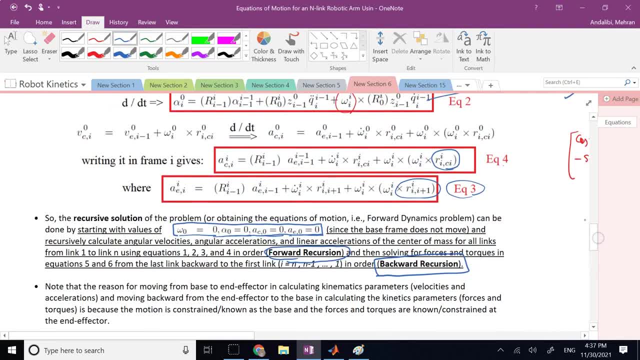 are needed for acceleration terms, right? So you need. you can see here I have these two r's right: r of i, ci and r of i and i plus one. Once you have those, then you can calculate acceleration terms from three and four. So these are those vectors. 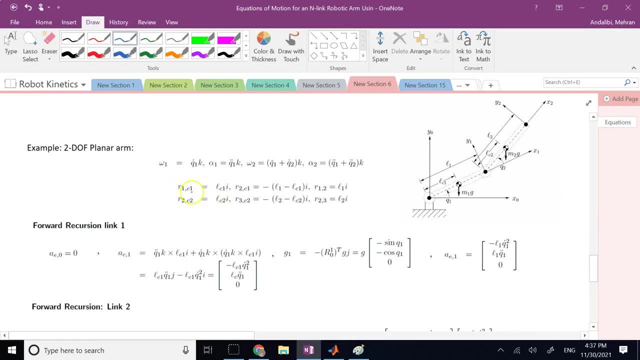 here You have r of one in C one, that's what you need- r of two in C one, and then r of one and two, And those are these vectors. This is the first one r of C one with respect to joint one right. 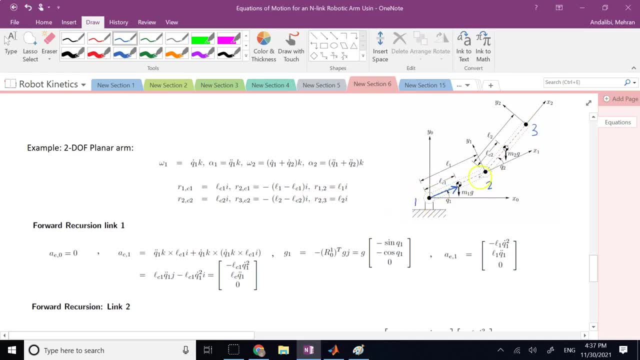 because that's joint one, joint two and joint three. The next, this one, R of C of 1 in 2, and then the other one is R of 1 in 2, which is basically this vector here. so clearly you see the R of 1 C, 1, the length of it. 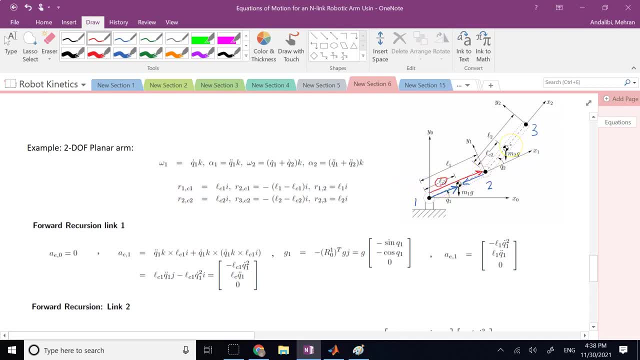 is LC 1 and the direction of it. it says I. now we have to pay attention this, I that it says here, here and here, all of them are eyes of frame 1. you are all, literally, I have this axis X 1. okay, they are not I of the base frame, okay, and 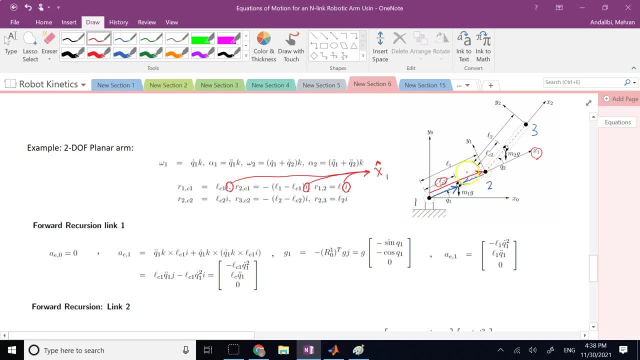 our of the C wanting to the length of it is clearly this length, which is L 1 minus LC 1, and the direction of this vector is backward, and the direction of this vector is backward, backwards. so that's why you have this negative term and r1, with respect to the whole length, is 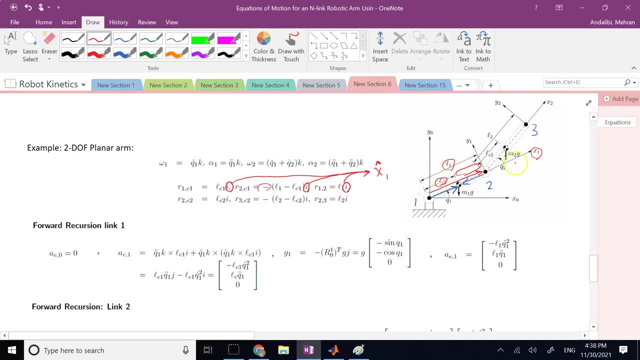 l1, and it is a long i. similarly, you can define r of c2 into r of c2 with respect to 3, and then r of 3 with respect to 2- these guys which you can see. so you need these vectors as well. what's good about using a body attached frame? this is one of the places. right, you see the. 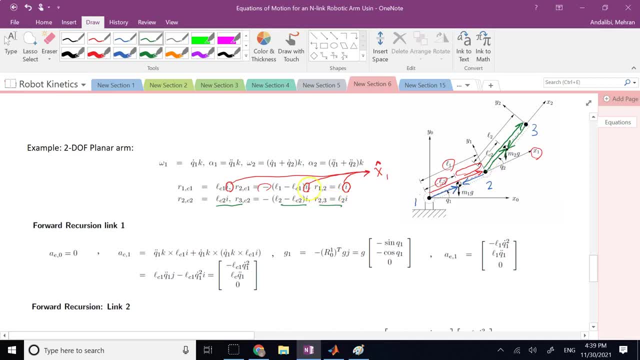 expressions are actually all written with respect to local unit vectors, and these local unit vectors make life a lot easier than to write everything about this i and this j. then definitely those vectors. you need a bunch of sine and cosine vectors to write everything about this i and this j. 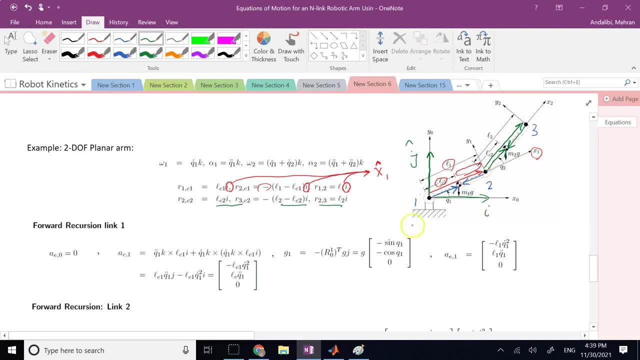 you need a bunch of sine and cosine vectors to write everything about this i and this j and then q1 plus q2 to decompose them, align the global unit vectors right. so when i use local unit vectors, writing it is a lot easier. just, we have to pay attention. when we say i, what do we mean by i? 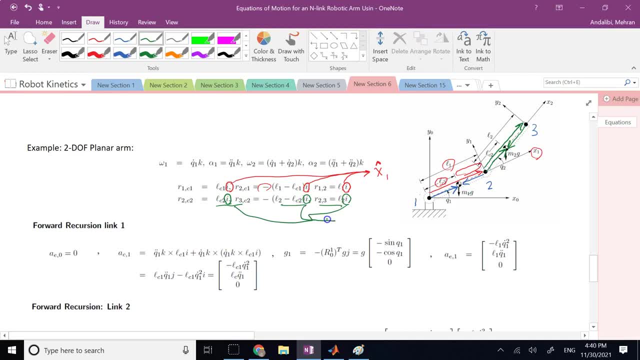 this second row. all of the i's are referring to what? to basically this one unit vector of x2. so please be careful about that. now, here we start with the forward recursion, which is basically finding the a's, and for that we start with the first link, then we go to second link. that's why. 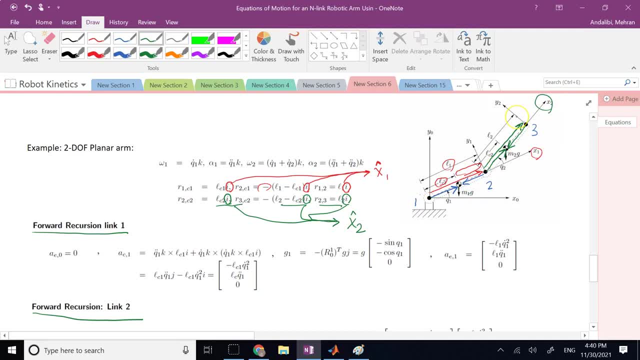 we call it forward, we start with the base, go to first link and then second link. so what we really do here is we start at the base, at the base, the. again, we start at the base and then we go to the second link and then we go to the second link of the entire unit vector and we have an 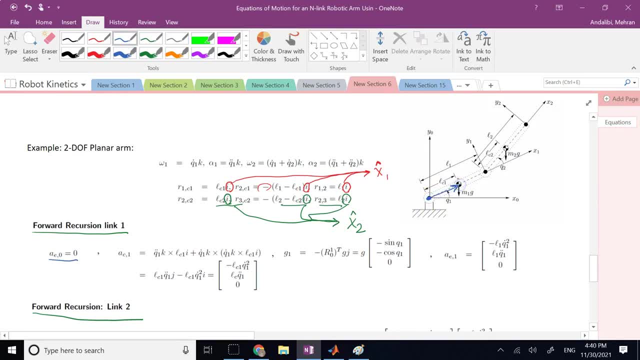 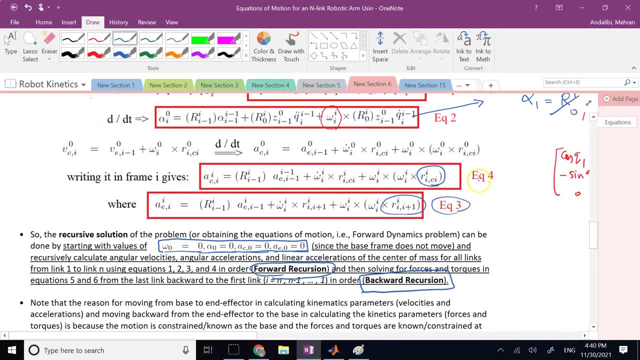 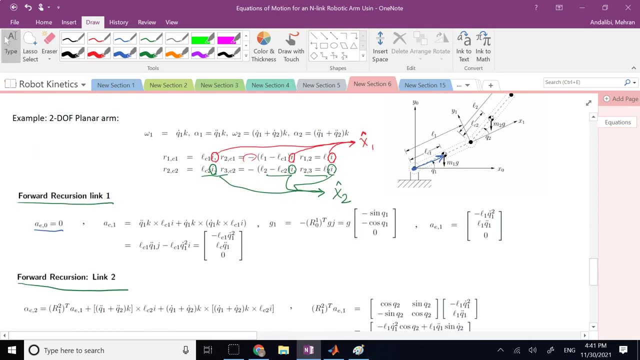 acceleration of this pin point one is zero. then once i have that acceleration of the centroid, this point is not going to be so hard because they both belong to the same rigid body. so i am going to use this formula, number four for i of one, and that will. 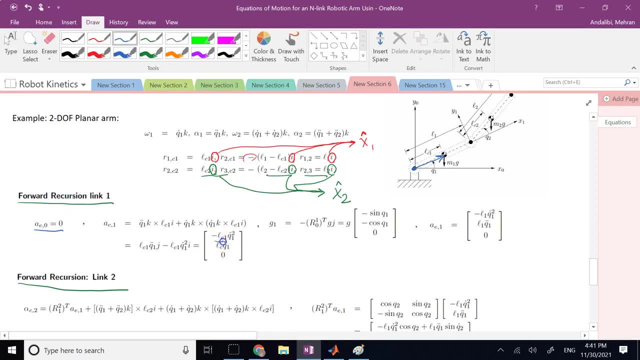 give me what. if i apply every term based on what we had in it, it will give me negative lc1q1.2. lc12 is one Q, one double dots and then zero. and does that make sense? absolutely, because if you consider those terms, the negative LC- one Q, one dot squared- is about I and 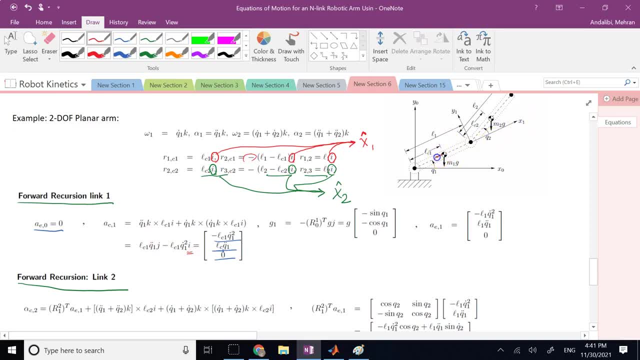 I means local I or X one. so it is basically in this direction. negative, the magnitude of it is LC one Q one dot squared, and the other term is positive J, and that's LC one, Q, one double dot. so it looks like this: so LC one, Q one, double. 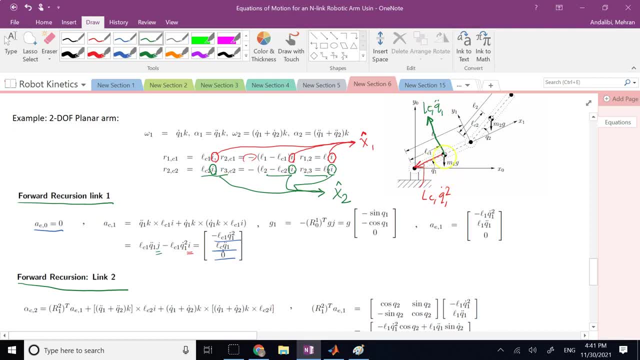 dot is the tangential acceleration and LC one Q, one dot squared is the sentry petal or normal acceleration. so definitely, see, it absolutely makes sense. as long as you know what is I, what is J, you also need acceleration of this point here, and that you find it very. 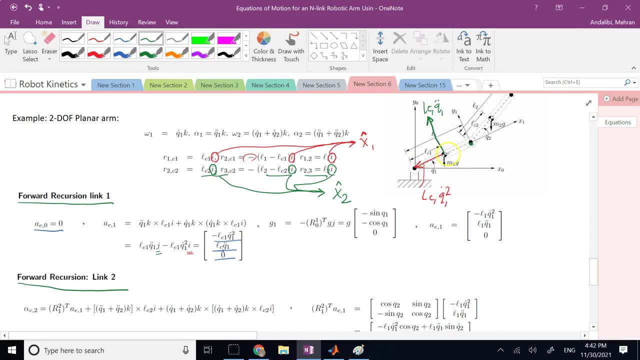 similar to the same way that you found acceleration of c1, except instead of LC one use the whole l1. so you see these two are very similar, except for LC one replaced with l1. one other thing you need is G. you see, here it says g1, it's. 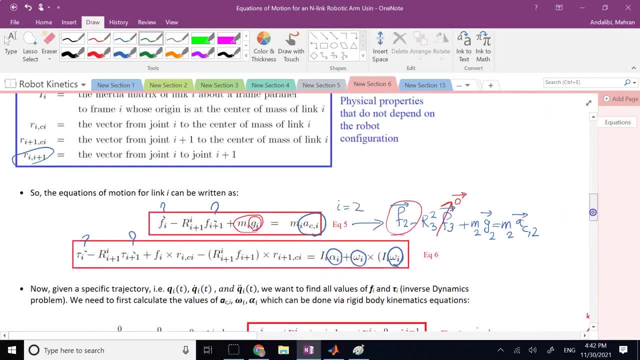 not g is g1. so you see, if you look at that request, you see that it says g1 is not g1. so you see, if you look at that request, you see that it says g1 is not g1. so you see, if you look at that request. 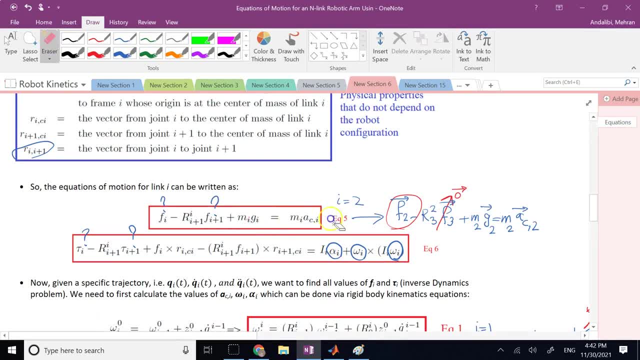 you see that it says g1 is not g1. so you see, if you look at that request, we are talking about G? I. and what does G I means? it means to project the mg or G align the local axis. okay, so that's this term here. it is important, so we need to. 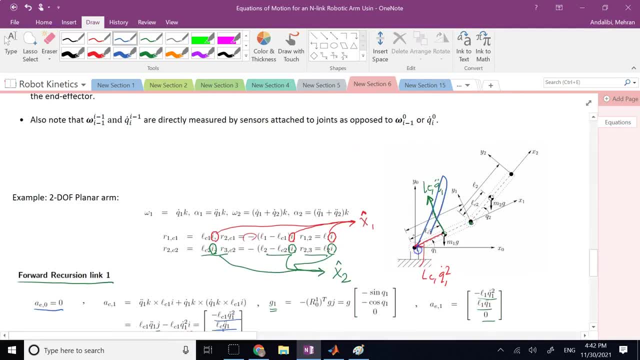 really project this gravity force m1 g1 allowing the axis of frame. one that is extremely crucial here here is that force m1 g1 and the axis of frame. one here is that force m1 g1 and the axis of frame. one that is extremely crucial here here is that 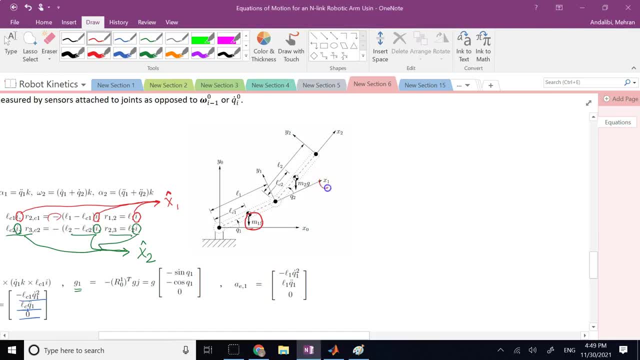 force m1- g1 and the axis of frame- one that is extremely crucial here here- is that force m1 g1, and then these are the axis, a line which force m1- g1 and the axis of frame- one that is extremely crucial here here- is that force m1 g1, and then these are the axis, a line which force m1- g1 and the axis of frame. one that is extremely crucial here here is that force m1- g1. and then these are the axis, a line which you need to project. so this is my force. you need to project, so this is my force. 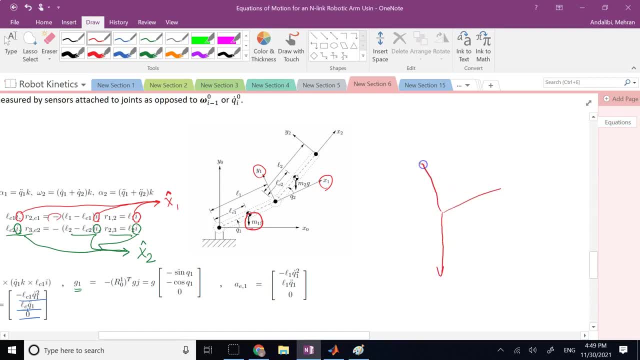 you need to project, so this is my force. these are the axis X, X is Y and this. these are the axis X, X is Y and this. these are the axis X, X is Y and this angle is definitely q1, or this angle you angle is definitely q1, or this angle you. 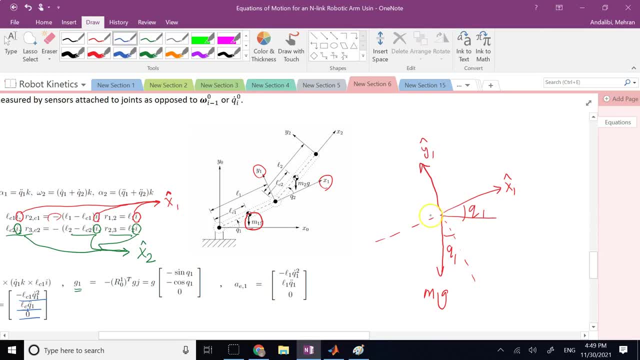 might say. and so definitely the components are going to be m1 G, cosine of q1 and m1 G sine of q1, and they're both negative. so that's why you see these components and there is no Z component. so that's a of C 1 which we 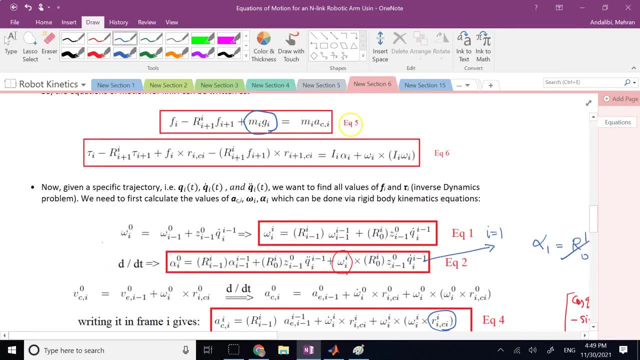 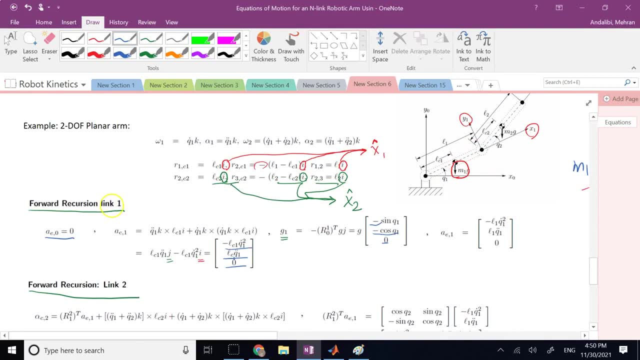 definitely need in equation 5, and then, once I have member 1 all figured out kinematically, which is called forward recursion link 1, now you go to link 2 because now you have acceleration of this point which is provided here. once you have that, now through link 2 you can find the 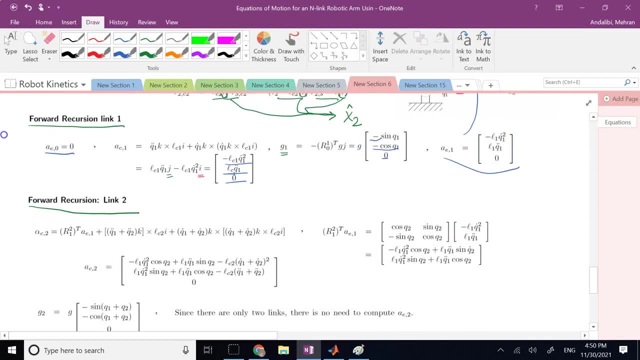 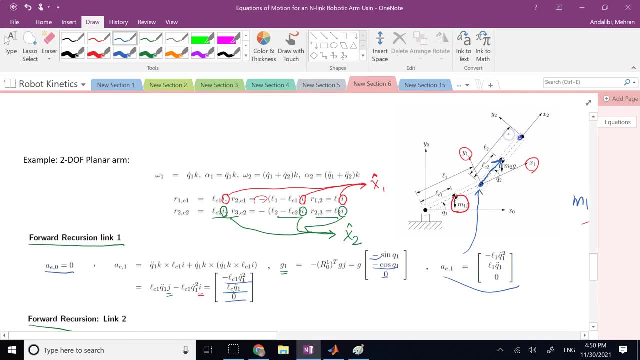 acceleration of this point, which is provided here. once you have that now and you can find the acceleration of the center a2 correct and that's what you can see here. okay, do I need to find the acceleration of this endpoint? no, you don't need it, because that one is not attached to another link, so all you need is now ac2. 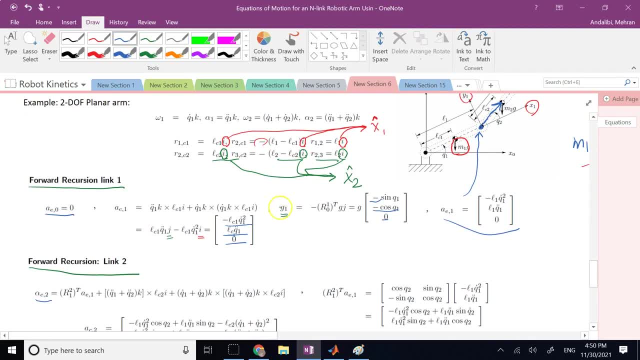 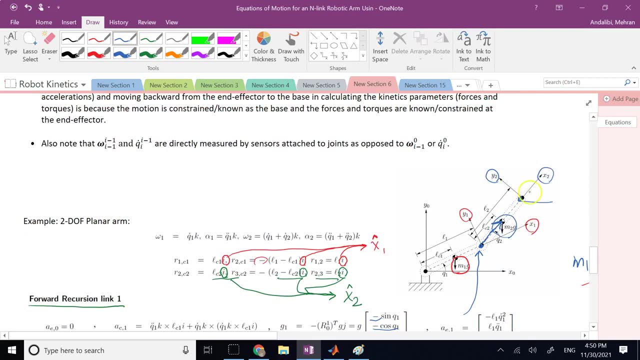 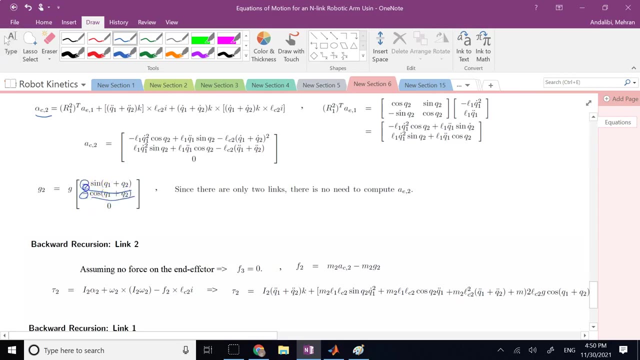 and there you stop again. you have to project the MG, this time along x2 and y2, and for that you need the total angle here, which is q1 plus q2. that's why you sine and cosine of q1 and q2 with negative signs are used for projecting g. and when you get this 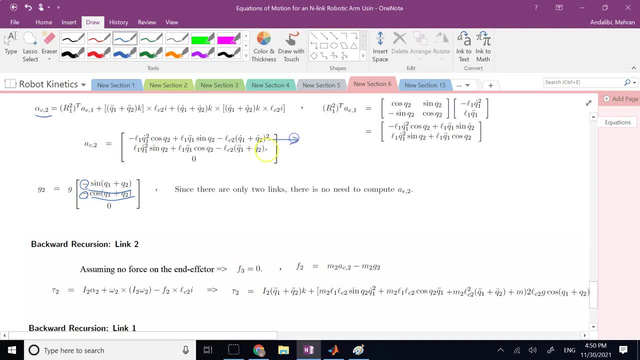 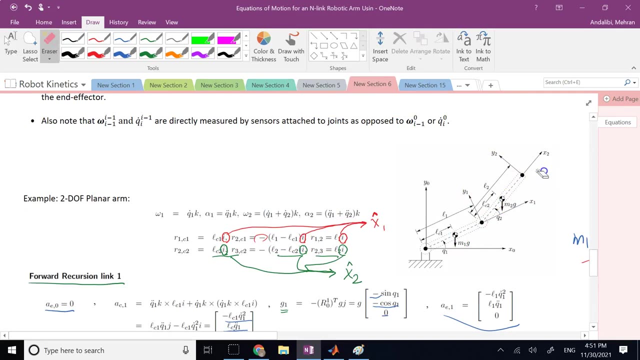 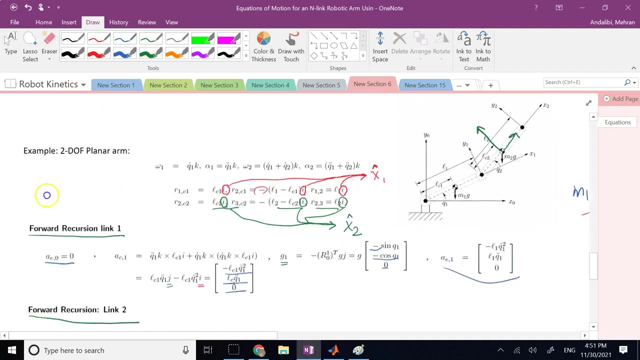 ac2. again, each one of these two components are aligned, the local x and y. okay, so if each one of them are a component that you might call ac2x and ac2y, then the direction of them is like this direction and this direction. okay, so now that your kinematics is done, recursion link. 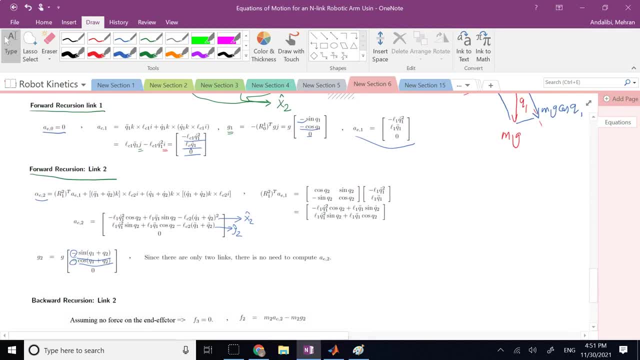 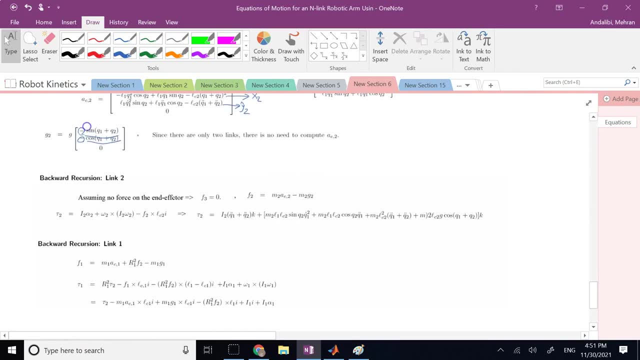 one and two forward. now we go to backward recursion. here you're going to use equations five and six, but you start at the end effector first and go back to the base. why? because at the end effector you can basically determine the forces. these are the forces that are applied. 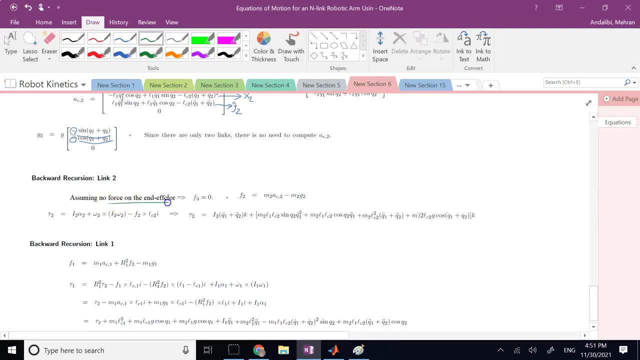 by the environment. so if we assume no forces at the end effector, then f3 the force on. really, if there was a frame three, if there was a frame right after frame two on the end effector, the force on that is zero and using that you can find f number two. how so? here you go to. 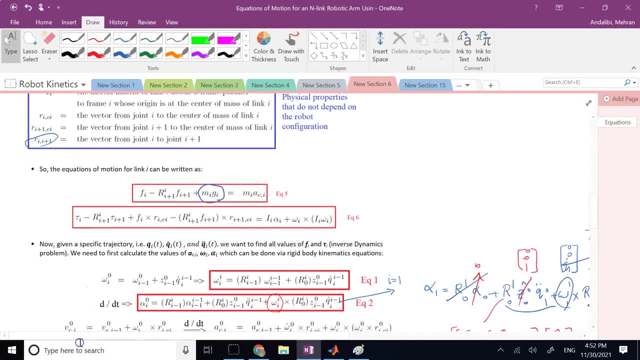 this equation, here this one, and in this equation you plug in: basically i equal two, which gives you f2 minus r of three with respect to two f3, and then plus m2, g2 is equal to m2 a of c and two f3 is zero. 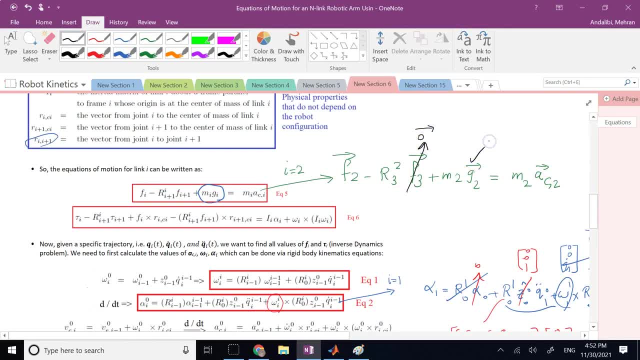 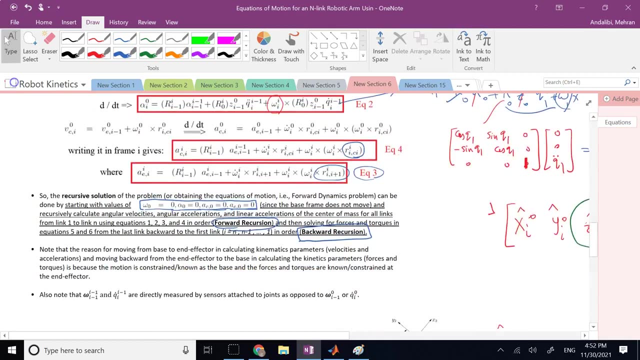 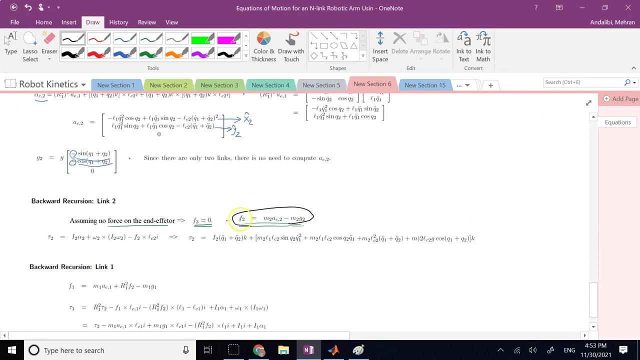 g of two is already calculated. ac2 is already calculated in recursions for forward recursion of link two. so if you take this term to the left right hand side it becomes f2 is equal to m2 ac2 minus m2 g2, and that is again exactly what you can see over here. so this is the reaction force. 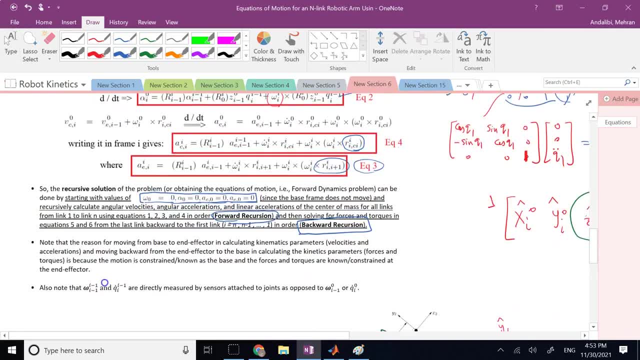 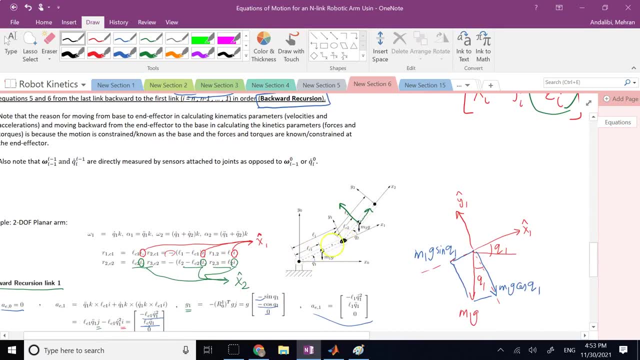 at pin number two, which is the force at pin number two, and that is the force at pin number two, which is basically this point here. so this is the force that member one applied to member two or member two applies back to member one, but when you want to interpret that, remember, just like anything else. 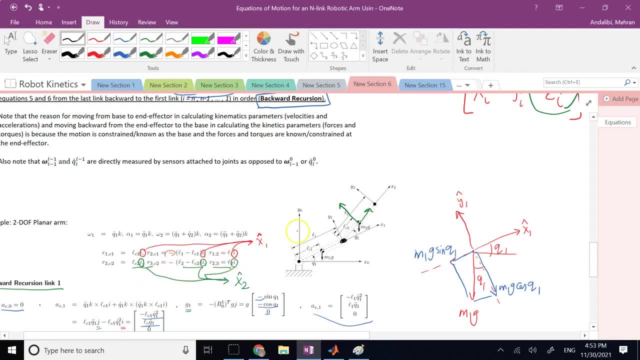 that f2. let's say, if you find some magnitudes and some directions like 2i plus 3j, what does it mean? 2i plus 3j, what is i? what is j? again, this is i, this is j because you use i of 2.. so if you found again, let's say, 2i plus 3j for that force, 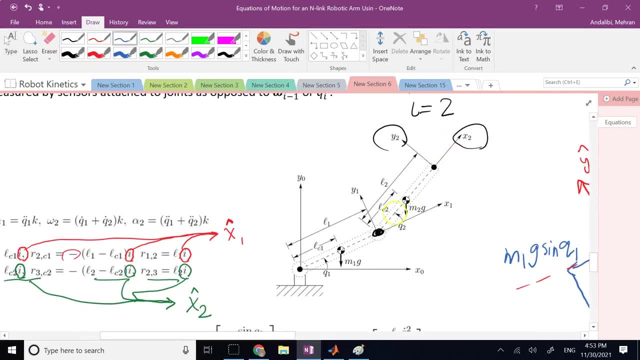 f2. that means what that means: two units align this direction and then three units align that direction. so your force is something like this. this is your f2, for example: right, the unit vector that you will find will be aligned x, 2 and y 2.. that's how you interpreted when it says 2 and 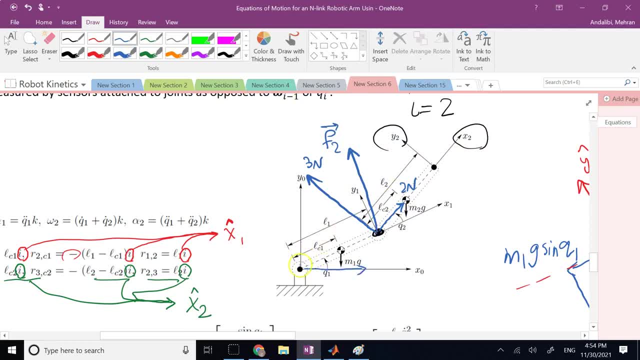 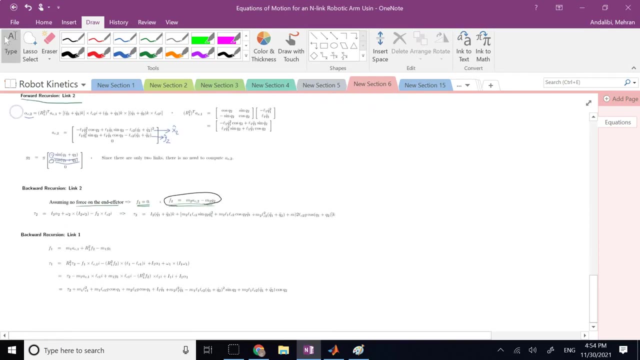 3. it doesn't mean to align the base frame x and 3 align base frame y. no, it's 2 and 3. the direction of them are determined by x 2 and y 2, not x 0 and y 0.. so that is the reaction force at pin number. 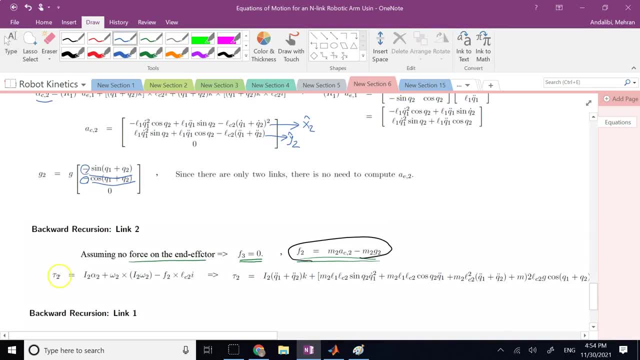 two are响 zb-2 and hvvero-12-11-11 andt-2-12-Ks2-2-x0-1-x0. So that is the reaction force at pin number two, and Then you apply the moment torque equation, which is equation number 6.. 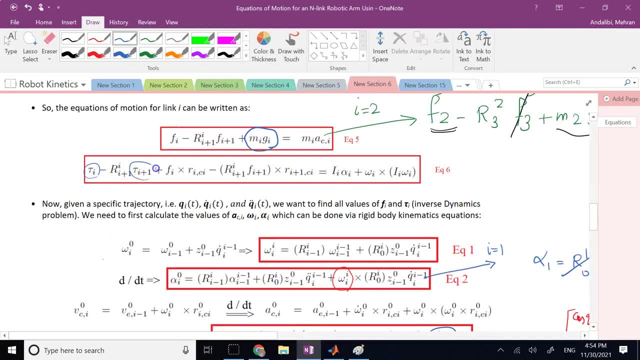 So here you're going to have T2 or tau 2 and tau 3.. Then you have F2 and F3, right, Remember F3, if I plug in I of 2, again right. So you have tau 2 minus R of 3, 2, tau 3, and then plus F2, cross R of 2 and C2.. 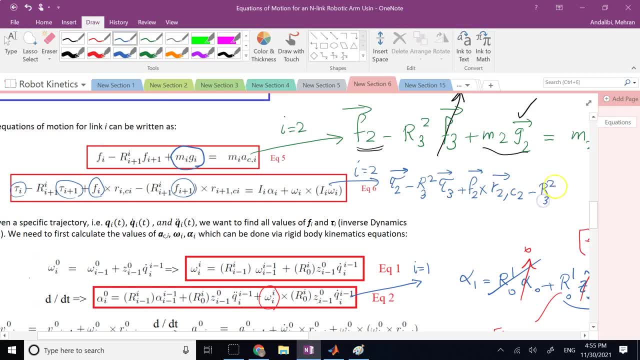 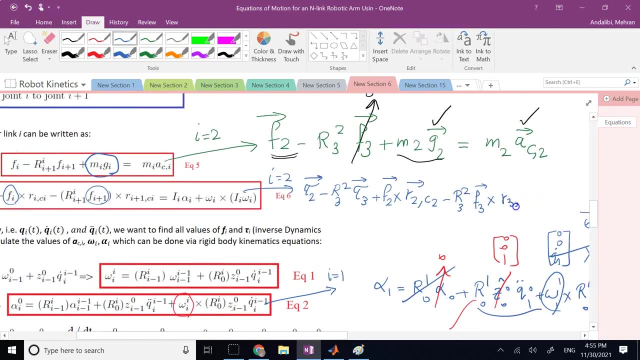 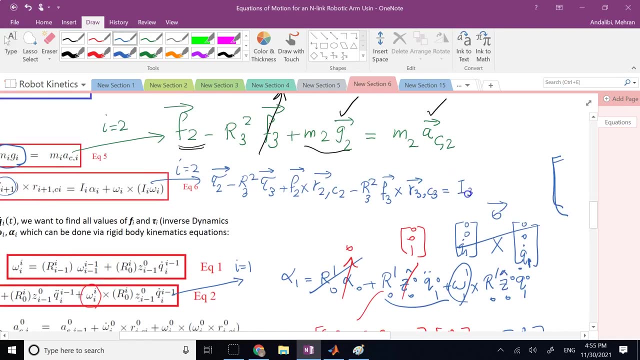 Then minus R of 3,, 2, F3 cross R of 3. And then C3 is equal to: and now you have I number 3, alpha, or I number 2, alpha, 2, right, Let me clean up in front of this area. 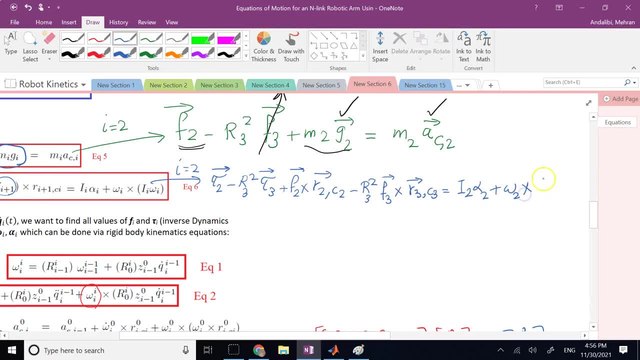 And then, plus omega 2, cross I 2, omega 2.. And guess what? Alpha 2 and omega 2 are already calculated for me. So I have them. I2 is already calculated. And the good thing about this I2 is I do not need to use a similarity transform to transform it back to any frame. 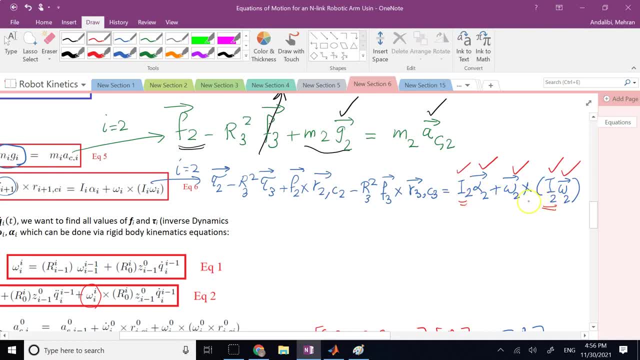 because it is already about frame I, or at least a frame parallel to frame I, by passing through the centroid. So I do not need to use a similarity transform to transform it back to any frame, because it is already about frame. I do not need to recalculate this I2.. This is the part that you just use it, as is Omega 2 and alpha. 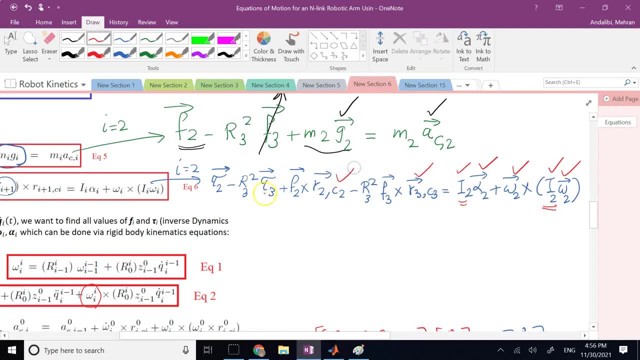 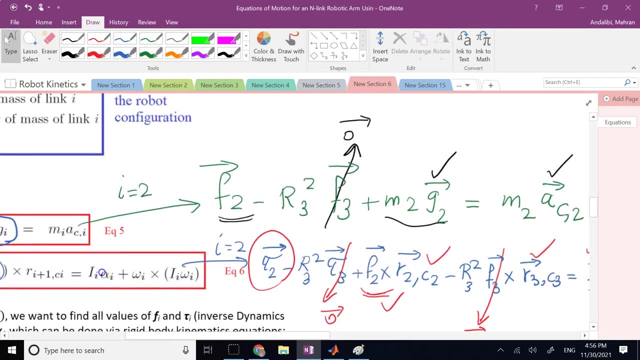 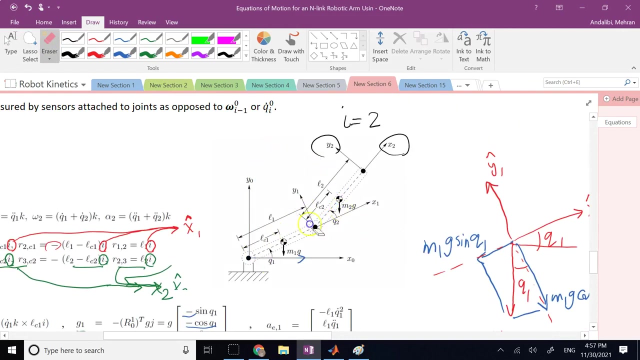 2 already calculated. The R's are calculated. Tau 3 is zero. F3 is zero. F2 is already calculated in the previous step. That allows me to calculate what Tau number 2, the torque that you have applied to this joint to rotate it correct. So now you can calculate what. 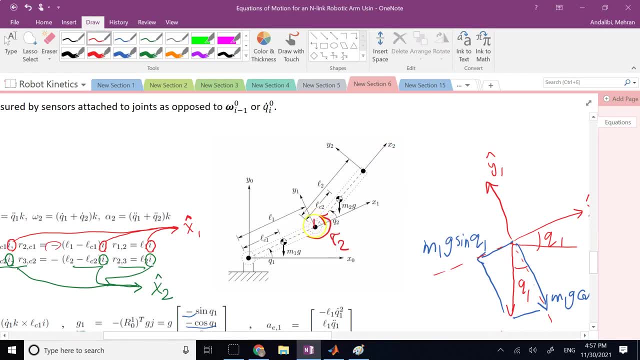 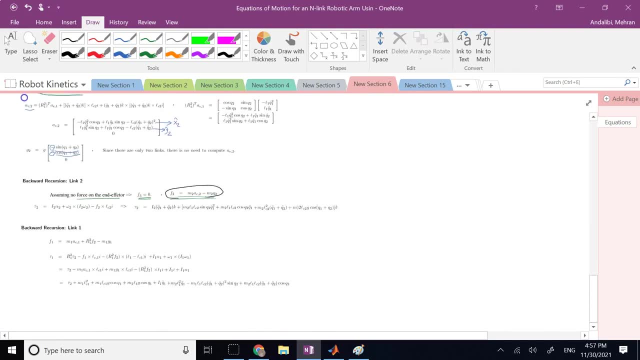 How much torque you need at that joint. So tau 2 and then F2.. You found both of these now in this step using equations 5 and 6.. So this is going to be your tau 2, quite long. 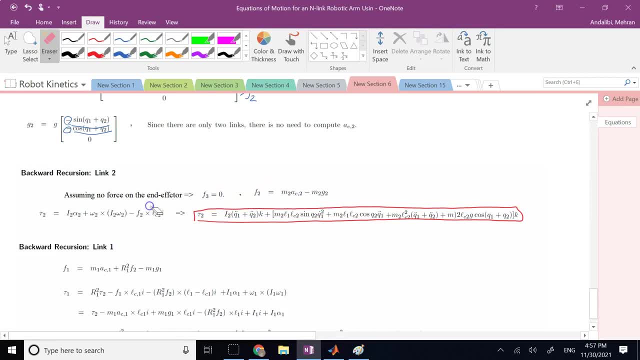 Okay, And, as I said, this is going to be your F2.. So this one is equation of motion, Because if I know the torque, I can find my double dot terms. On the other hand, if I know my double dot terms, I can calculate tau. This F2 is definitely. what Is the reaction to? 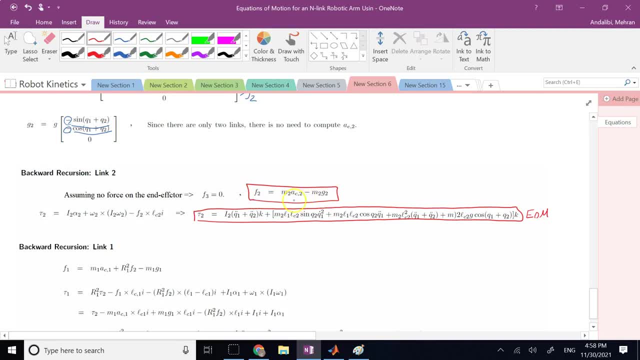 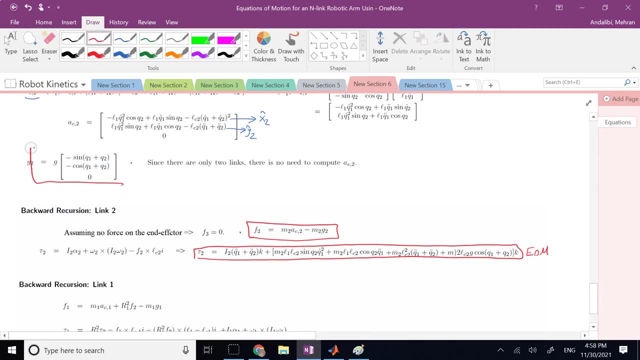 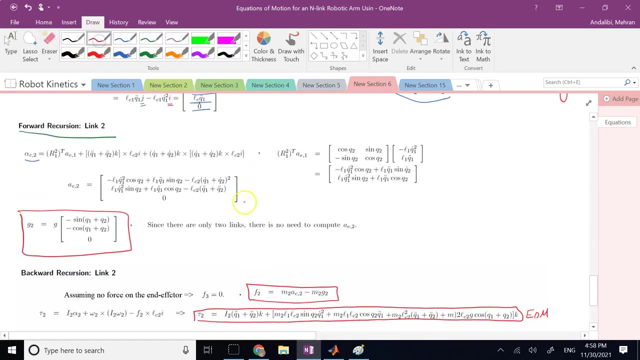 the reaction force. For it, you clearly see I need G2 and AC2.. And G2 is already here And AC2 is what It is also calculated up here. There are double dot terms in it. So this equation: if I want to determine the force F2,. 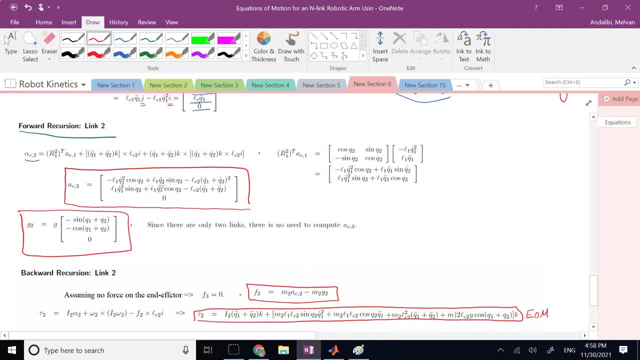 I also need to know the force F2.. So I need to know the force F2.. And this is going to be the force F2.. the double dot terms? okay. so this is also like equation of motion too, because there is double dot in it. so i have to combine all of this together if the q's are given to me, if i exactly. 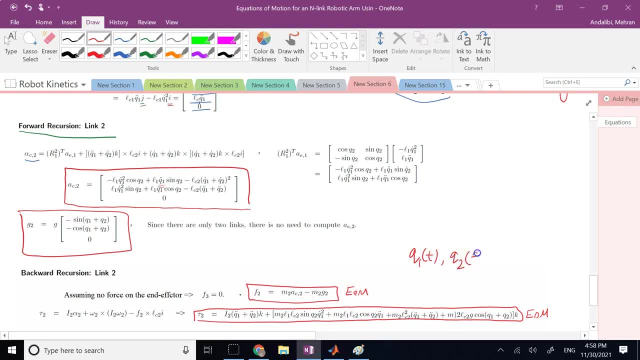 know q1 of t and q2 of t. if somebody has dictated these two to me and says: now find f's, find the taus, well, you can easily do that, because once you know the q's, it means you can also determine what the q dots and the double dots, and once i know those i can calculate any term inside these two. 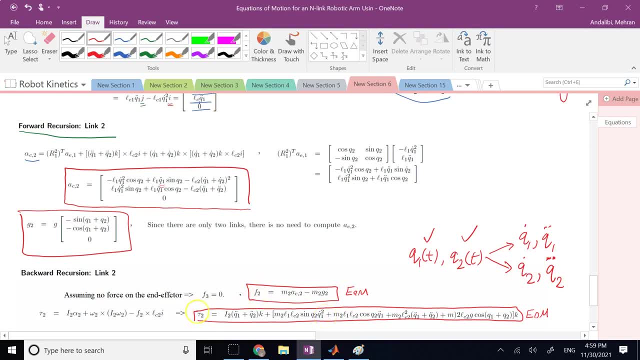 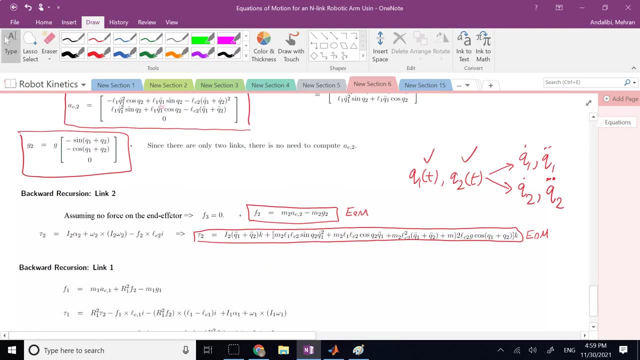 last equations, and that means i can determine my pin force and i can determine my tab. on the other hand, if the um uh taus are given to me, the torques are the joints, then i need to solve this equation, along with another one that we derive for the next link. 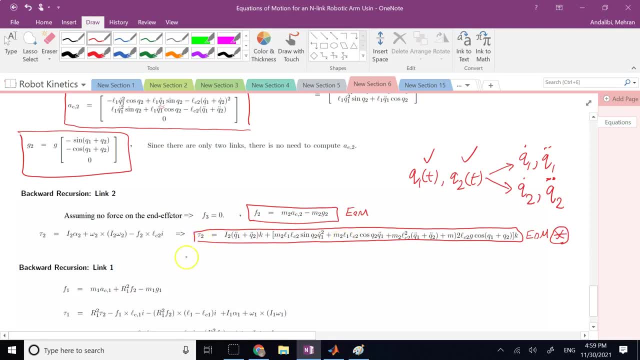 and in that with tau 2 and tau 1, given i need to solve for the double dot terms, that gives me differential equations. two second orders. if i can decouple them and solve separately. for the second order, i can decouple them and solve separately for the second order if i can decouple them and solve separately for. 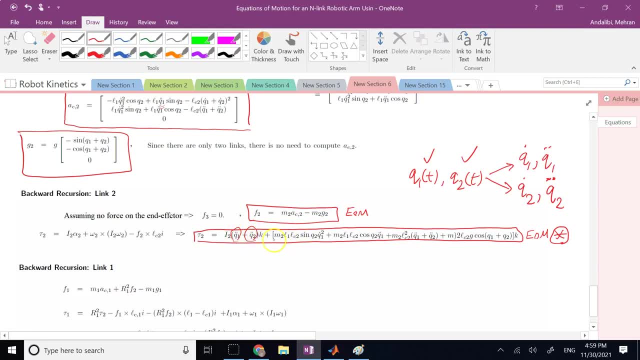 them. then through the numerical solution of that, with the taus given, i can find q1 and q2 and the dots all numerically and then i can plug them back into this equation and that gives me the values of the force numerically. there is very small chance that you can solve these equations of motion with 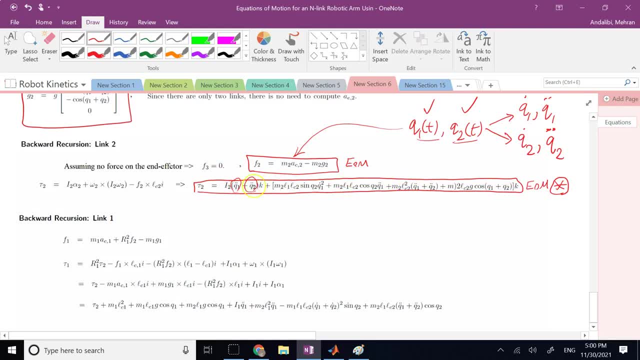 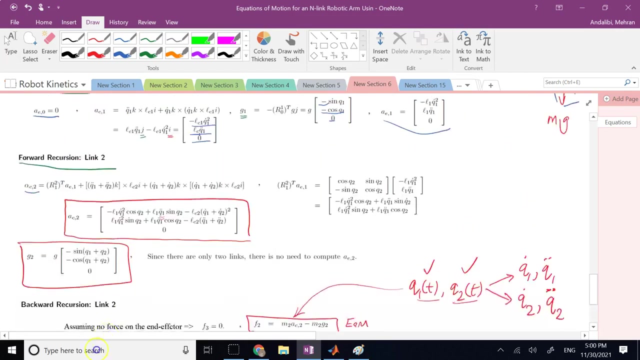 given torques analytically, because if you look at the equations they are highly non-linear, highly non-linear coupled second order ode's. so once you know your forces and torques on link number two, now you go backward to link number one and you apply i of one to the equation number one. that gives you f1, the force at pin number one. so 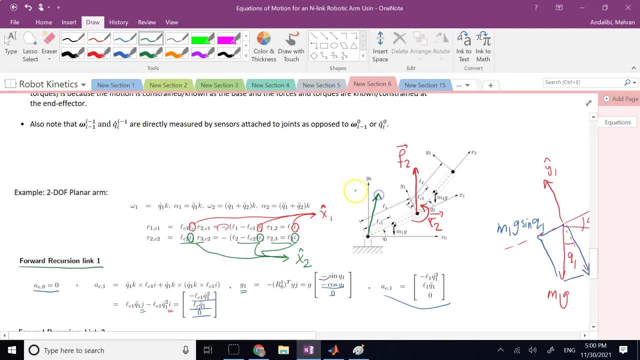 it is going to be something like this, for example, and it also gives you the torque that you need at joint one and similar to tau two and f2, the components. when i say two i plus three j for f2 and tau two, they were both about what- x2 and y2, when i'm talking about tau 1 and f1, and i saved like 4i plus 6j. 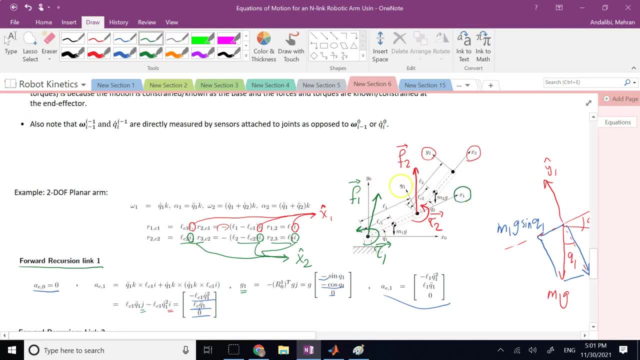 here i and j means what the x's are, frame one. okay, so f1 and tau 1 are described in frame one. tau 2 and f2 are described here, described in frame two with respect to unit vectors of that. so be very careful, none of those are described in the base frame. so if I do that, now I have my f1. 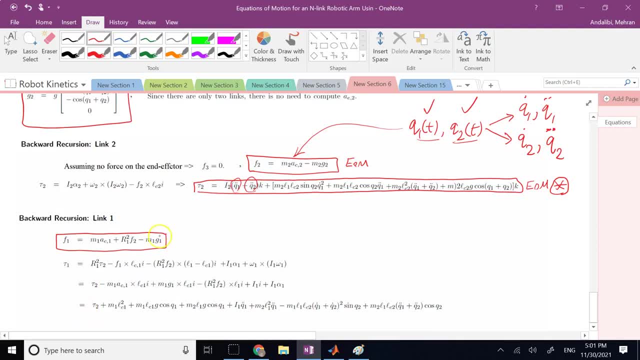 the pin reaction at pin one. for that I also need f2. so this f2 has to come down here and then I can calculate tau 1. for tau 1, not only I need f1 right, I need a bunch of other terms. and if I do that and simplify for f1 based on what I have, 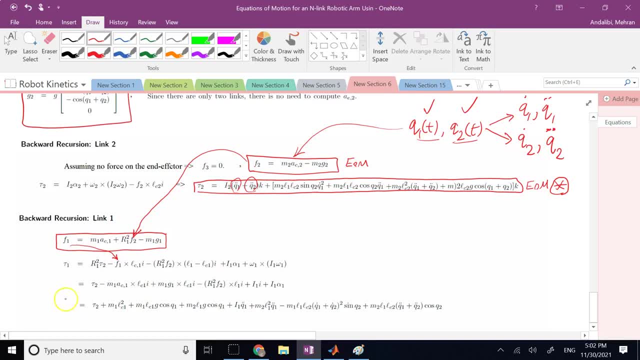 and do a bunch of simplifications, you will get tau 1 is equal to tau 2, and then you can plus all the other terms and you might say: how come you have both tau 1 and tau 2 in here? well, the reason is, if tau 1 is applied to, 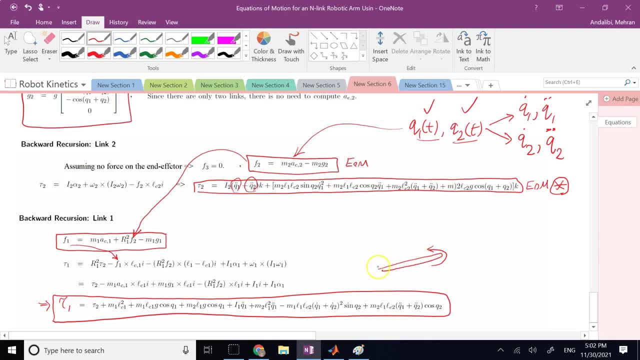 joint 1 here and tau 2 is applied here. it's the relative measurements again, because this tau 2 is relatively met. it's measured with respect to a frame that itself it is driven by tau 1, so it is kind of normal. that's the real. 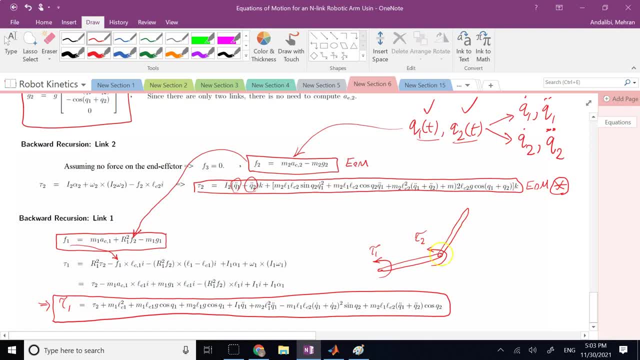 effective tau for the motion of that joint alone is kind of like tau 1 minus tau 2, which you can. take this tau 2 to the other side. okay, so here I have a food one and I have all of these equations and that means I can now 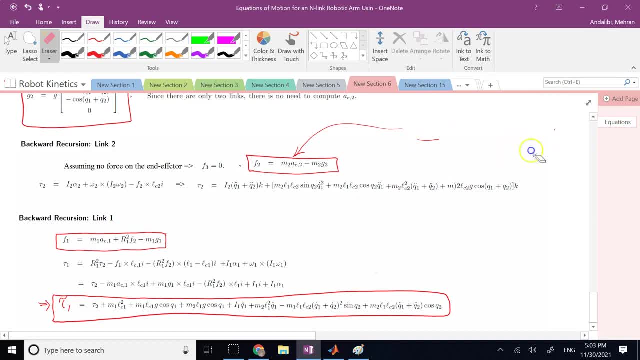 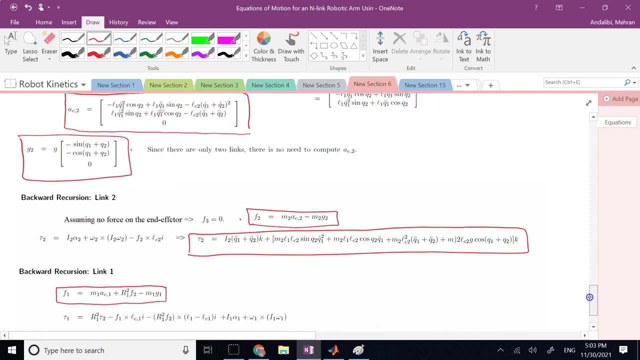 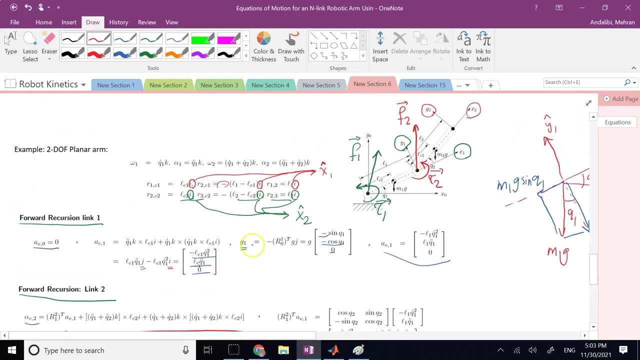 simulate the behavior of this system and find all of the reaction forces. so let me just put them all in some boxes for you: f2, tau 2, f1, tau 1, and for that I I also need to know G1 and G2, and AC1 and AC2, and that's AC2, G2, and then here is AC1, and what G1. 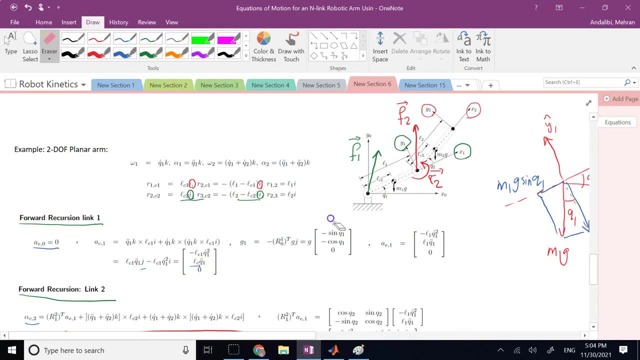 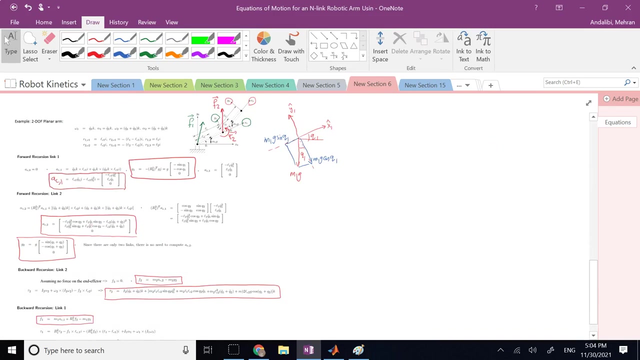 So once I have all of this, then I am good to do any, let's say, MATLAB simulation or anything for that matter. So here let me mark down what are these that you need to have handy here Once you have these six equations inside these boxes, or more eight really. 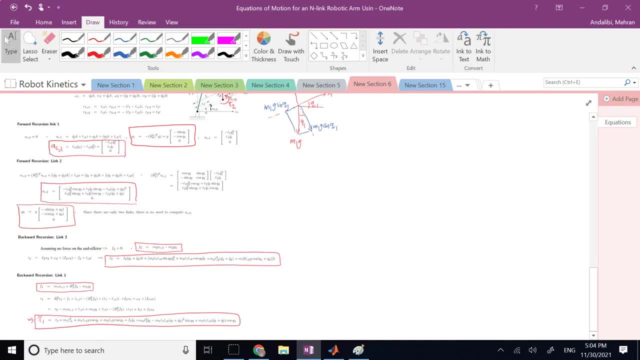 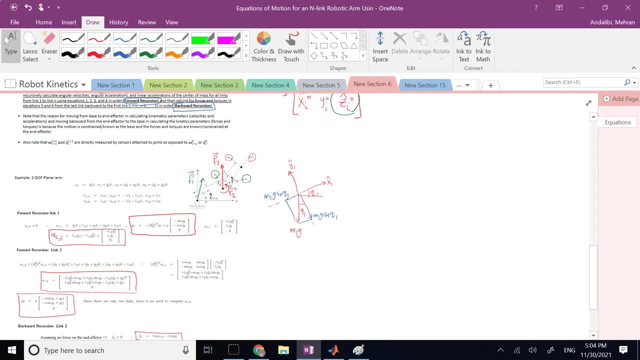 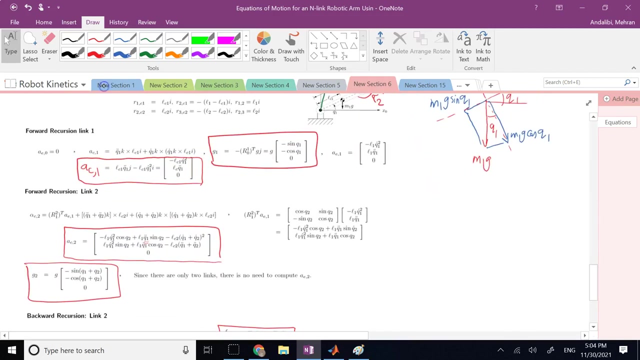 you can simulate the total behavior of this simple 2D planar arm. So now imagine if your robot has six joints Or something, how much more scary looking and much more complicated the shape of your dynamics equation is going to be. But as you clearly see here, the Newton method allows me to calculate Fs. that in the Lagrangian method. 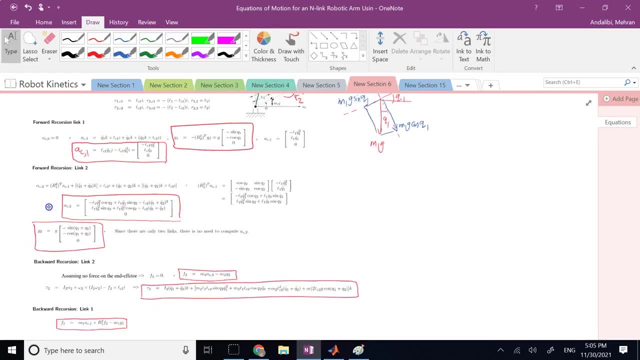 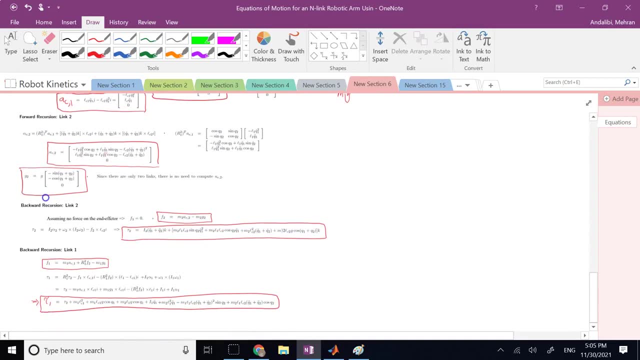 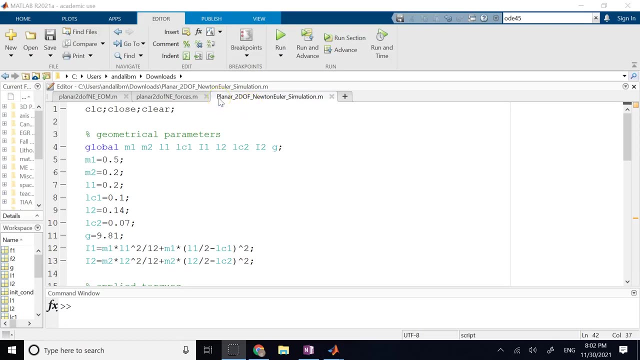 they disappear and they never show up. Okay, so here I'm going to show you a simulation of this H2O And I'm going to show you how to calculate equations in these boxes in MATLAB. So here is the code, that is the script. 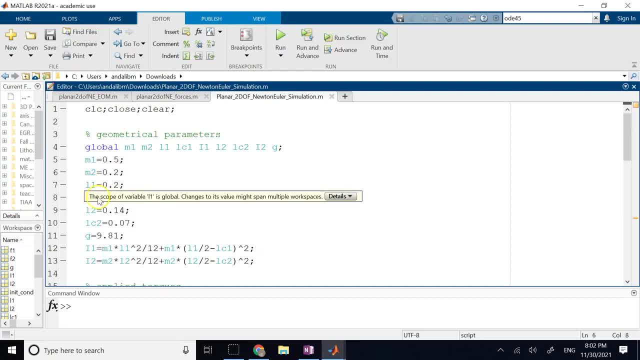 You define all of your parameters here. I made the Lc's to be half of L's, So the center is are exactly at the center of each link. Calculate the moments of inertia. They are all defined global parameters. I have two torques, five and three Newton meters. 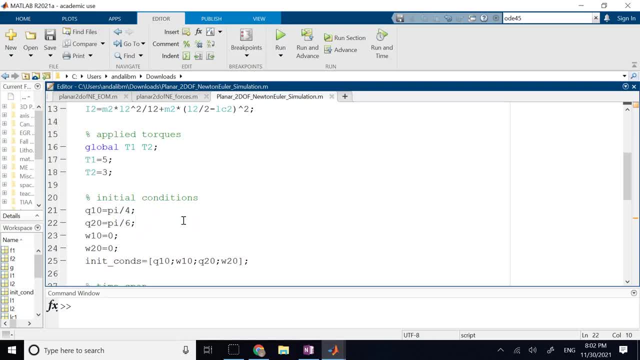 I have these initial conditions. They are 45 and 30 degrees for Q1 and Q2.. The omegas: we start from zero. We solve this set of equations for two seconds. And then here I have one function that I use with OD 45 to give me the solution. 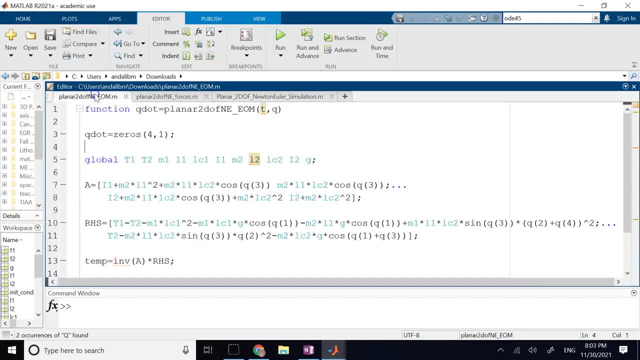 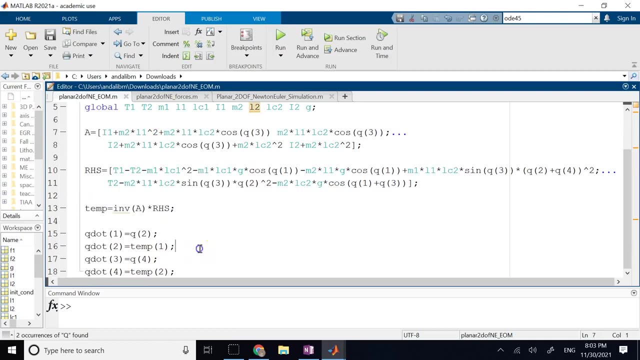 Q1 and Q2 versus time Right, and that is this function. So here what I did: I solve for Q1 double dot and Q2 double dot From the governing equations and then here And then I use those to be the time derivatives of Q1 dot and Q2 dot. 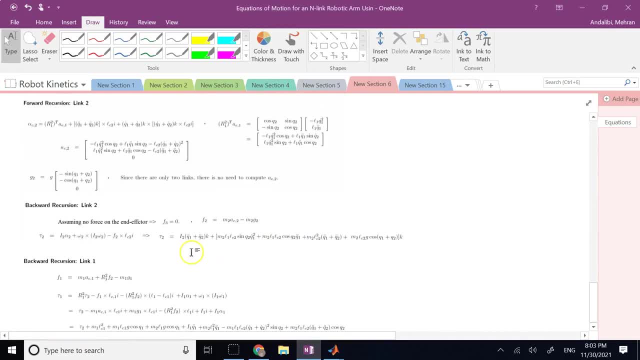 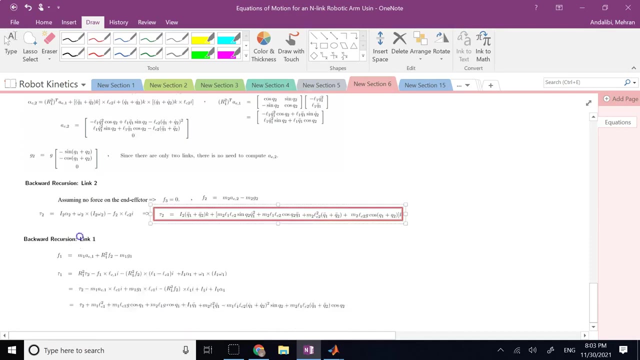 Because if you look here into your governing equation, this one here, Right, if you look here, this equation is not only about Q2 double dot, There is also Q1 double dot in it. The same thing goes down to this box. 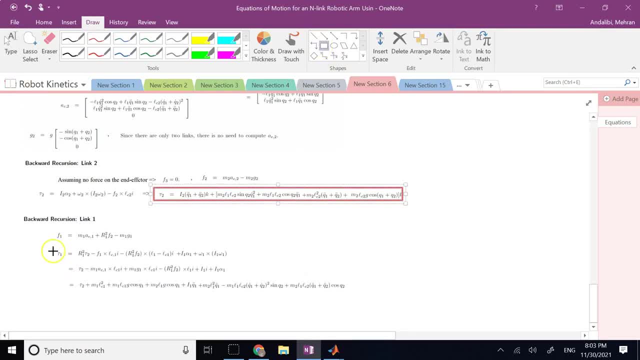 This is the bottom equation here. Also that one right again. if you look at the last line, You clearly see in the last line you have both Q1 double dot and Q2 double dot. So what I did? I wrote the equations inside these two boxes. 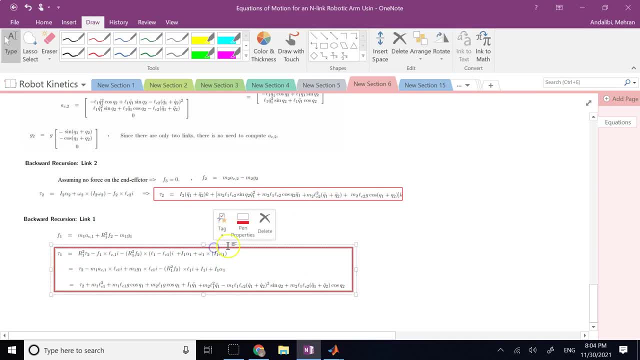 Specifically for this last, for the bottom one is the last line really. So tau 1 equal the whole thing. I wrote those two as a linear set of equations: A coefficient matrix times the unknown vector. Q1 double dot and Q2 double dot equals a right hand side. 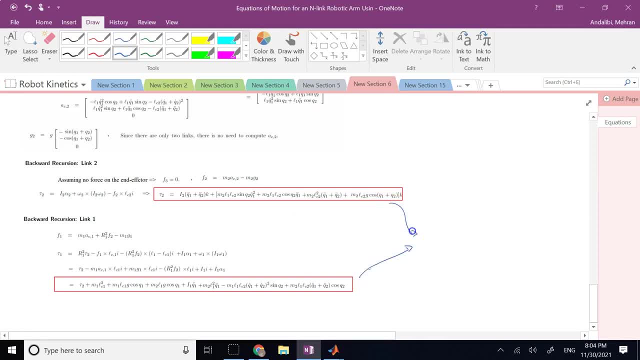 Right, so this is what I did. And A and right hand side. as you clearly see, there are functions of tau 1, tau 2 and Q's and Q dots, And then I use inverse of A multiplied by right hand side to get my double dots that I need for OD45. 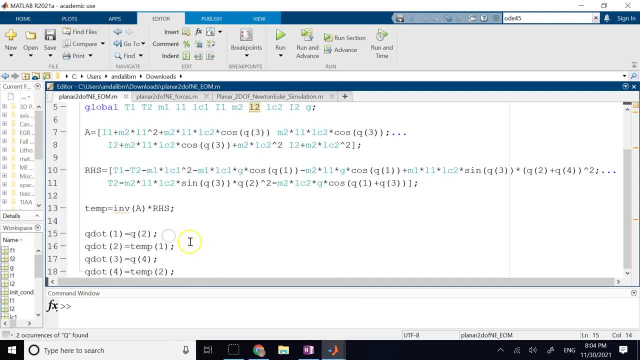 You know, OD45 only solves first order ODEs. Here you have two second order ODEs, so you need four dummy variables And that's what you see over here. Please watch my video on solving dynamic problems, or what we call initial value problems, using MATLAB with OD45. 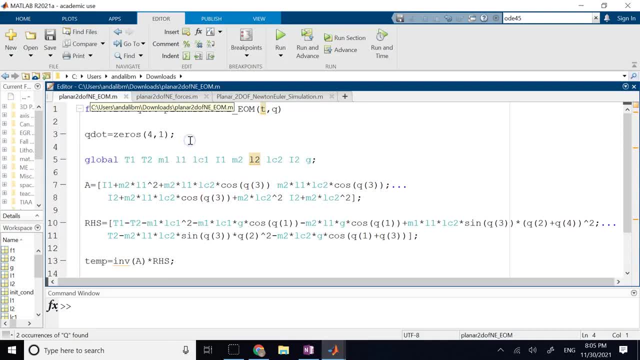 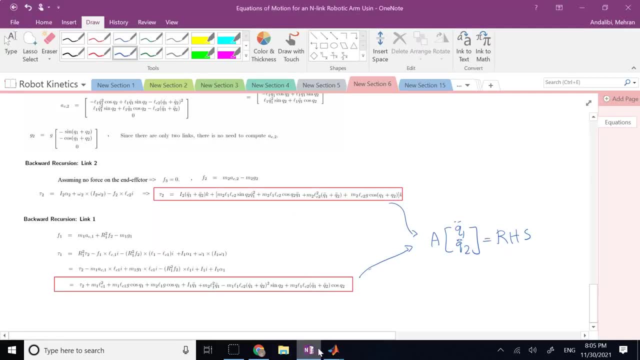 It is under my playlist, MATLAB, And you can see how you can use OD45.. So when I did that, then I have another function. I pass all of the Q's, Q dots and the double dots. I pass all of them to those calculating functions. 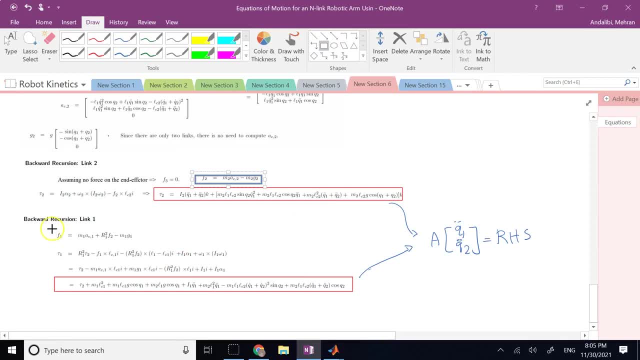 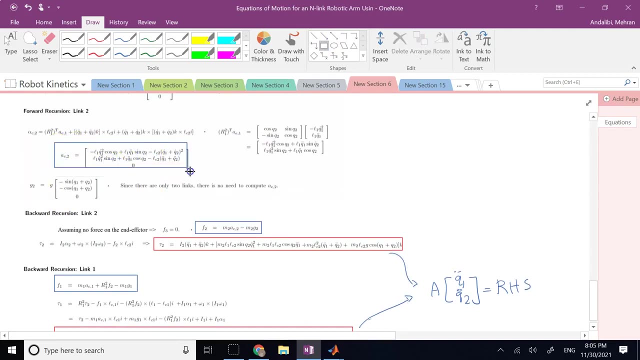 And those functions based on these two formulas will calculate for me F1 and F2.. Right, And clearly, when you calculate F2. You need to know your AC2.. Right, And you also need your G2.. So these two guys here. 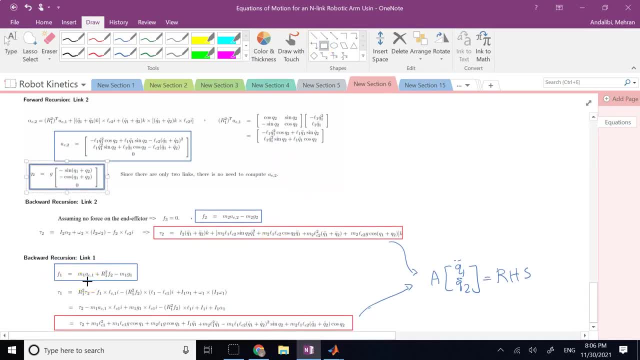 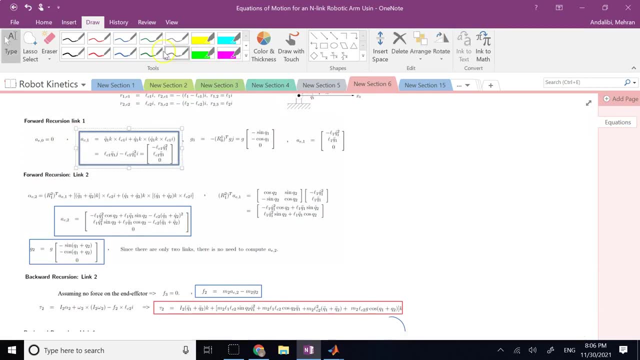 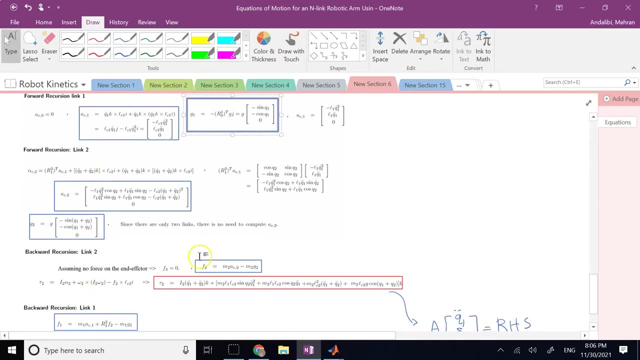 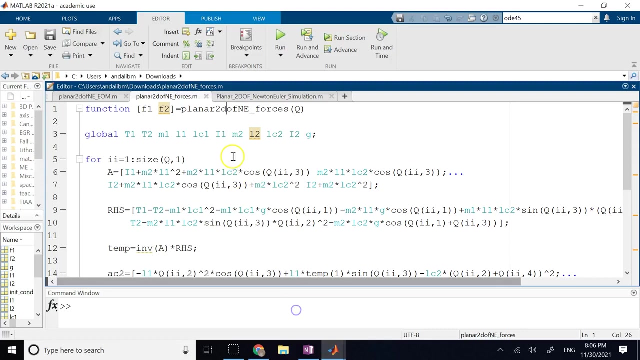 And when you calculate your F1, you need AC1 and you need G1. So you need this one here And this one. So all of those are incorporated in the second function to give me F1 and F2.. And this is this function. 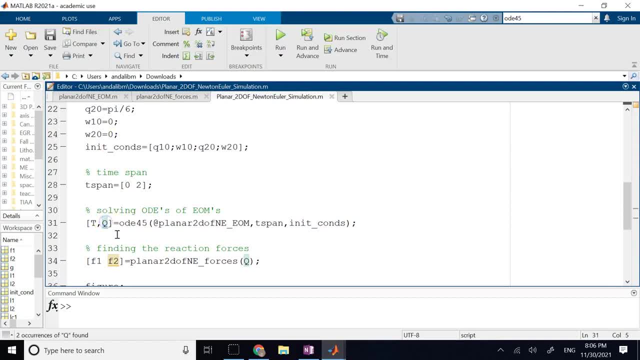 So when in my script I solve for Q's, then I pass all of the results to this function. It gives me F1 and F2 as big vectors. And then here I'm plotting versus time The norm of each one of these vectors for each time point. 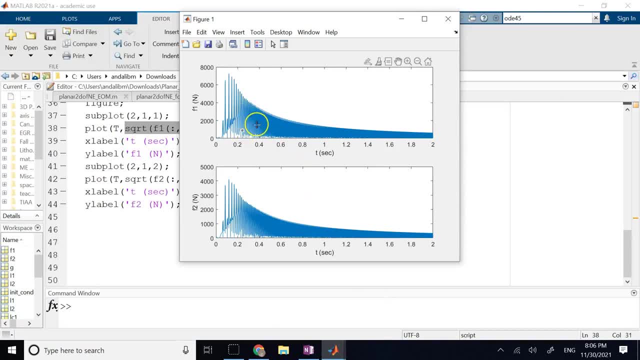 And this is the result. As you clearly can see, it has a ton of oscillations Due to nature of the physics of the problem. All of those centripetal and Coriolis acceleration will cause all of these oscillations that you will see. 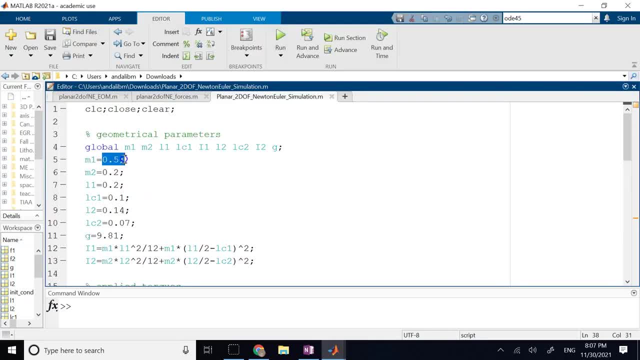 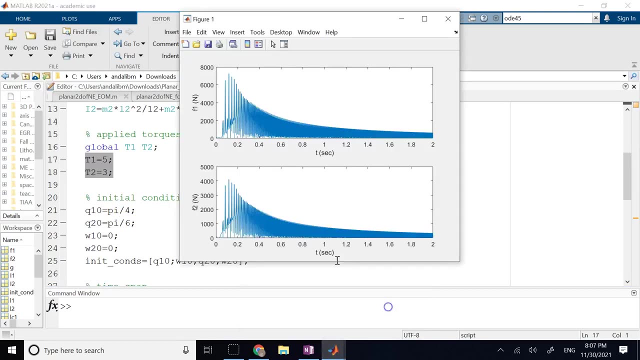 And even for a small robot with like half a kilogram first link, 200 gram second link, 20 centimeters first link And 14 centimeters second link And some relatively small torques. If you look here, The maximum value of my F1 can go all the way up to something like 7300 Newtons. 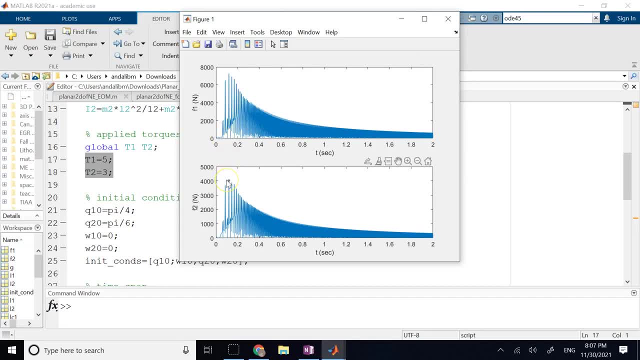 And the same thing. for what? For F2 also, it goes above 4000 Newtons. Okay, So definitely the load is variable, So you definitely will see fatigue In those joints that are subjected to the forces F1 and F2.. 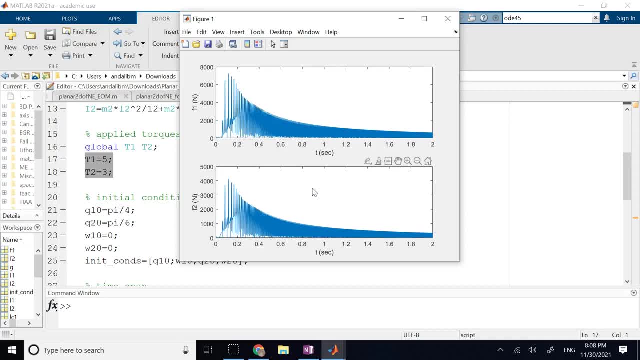 But even if you want to design based on static analysis, Which is absolutely wrong- But if you want to do that, What force do you consider here? on the joints, Definitely you need to use the maximum force that you can see here, Right? 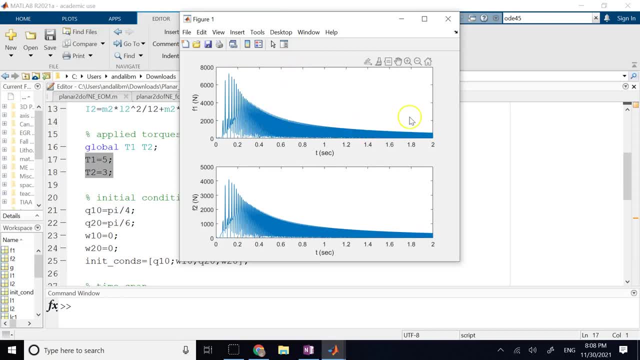 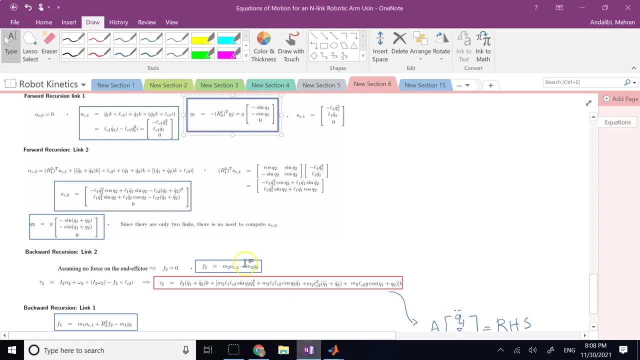 So these are extremely important for your design purposes, To know how much force is at each and every one of the joints. This you cannot do by a Lagrangian method, And one thing that might cross your mind is: Well, if I go back here for F1 and F2.. 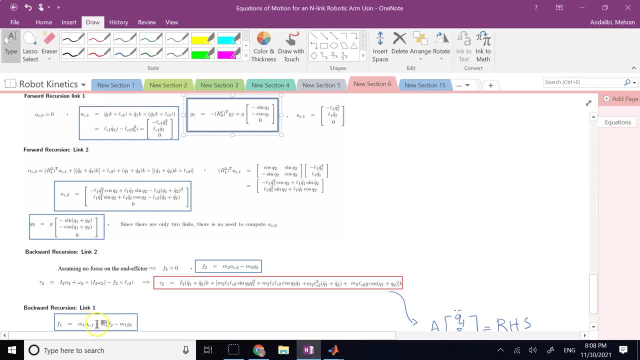 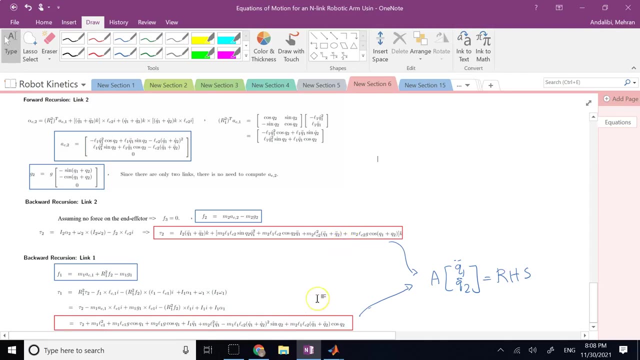 What I really need is acceleration of Centroid 1 and Centroid 2.. Can I find them by Lagrangian? Well, Lagrangian gives you these two equations of motion in red, Gives you something very, very similar to that, With the exact result. 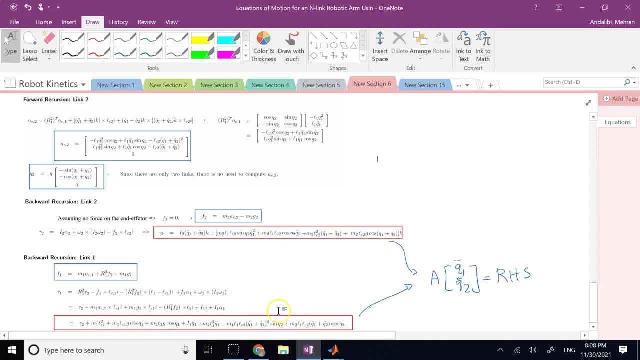 Okay Now when these two equations will give you Q1 and Q2.. When you use OD45. Right, And OD45 gives you Q1 and Q2.. So you can Also you can have Qdos and Q2.. Q- double dots. 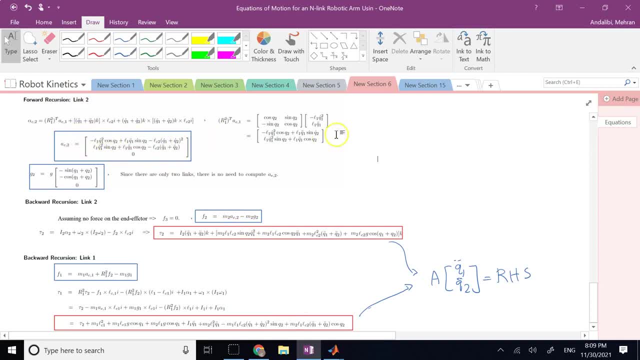 Then you can go and calculate AC1 and AC2. Based on these formulas. So if I want to get to these two equations in red, Do I need to use Newton, Euler? Absolutely, But alternative is to get to these two equations also using Lagrangian.